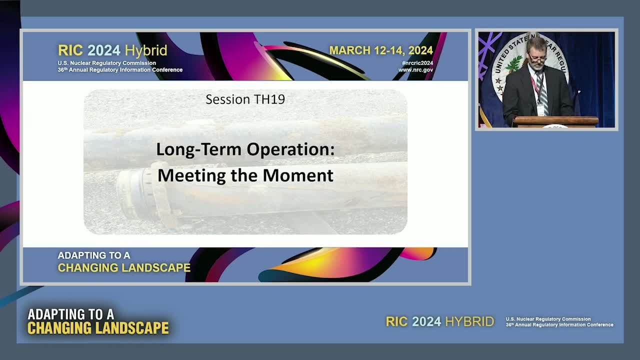 Meeting the Moment Here in the US and across the world, as the power reactors age to their original license and into long-term operation, we have seen various degradation issues arise. According to the IAEA, about two-thirds of the global fleet global reactor fleet of 413 reactors is over 30 years old. Specifically here in the US, for the fleet of 94 reactors, 90 have exceeded 30 years of operation, 54 have exceeded 40 years and with our oldest reactor being unoperated for 54 years, We've been busy for many years now with evaluating license renewals. in the US, Only nine reactors still have their 40-year licenses, 78 have been initially renewed for 60 years and six have been subsequently renewed for up to 80 years. 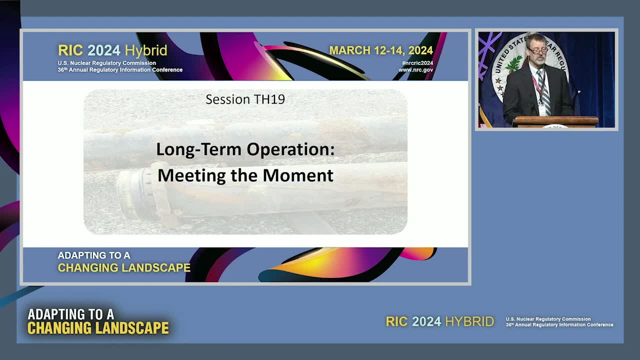 With many more under review right now and many more applications expected. Luckily, we are not in this alone. International cooperation continues to serve a valuable role in long-term operations. Through this, we were able to share operating experience and emerging issues with our foreign partners. 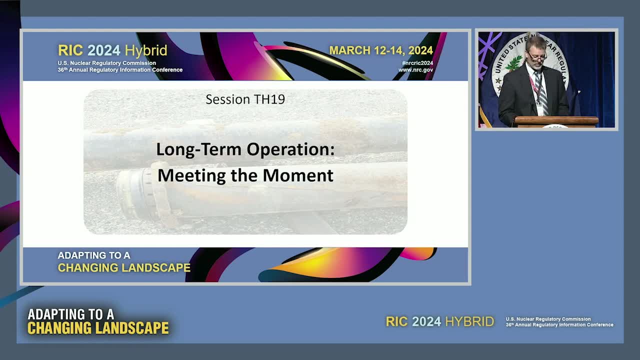 like we have with us here today. We're able to leverage research programs and share best practices in aging, management and regulatory strategies. We do this through bilateral engagements, such as on Monday, when we met with Flavian to talk about thermal embrittlement of cast austenitic stainless steel. 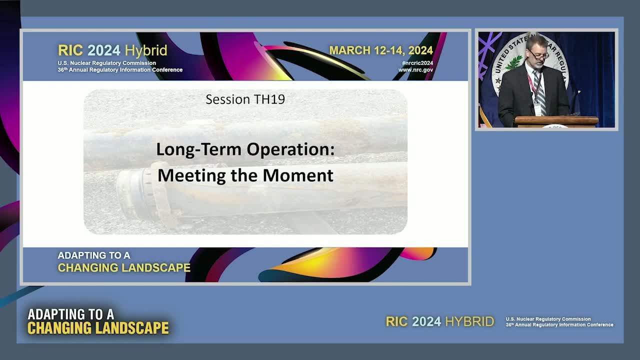 And on Friday we're going to meet with Haruku to discuss PWR core barrel cracking and stress corrosion cracking, And we've had ongoing discussions with Jen Ho and Kins throughout the year. We're also active in ongoing multilateral programs, including the IAEA's IGAL program. 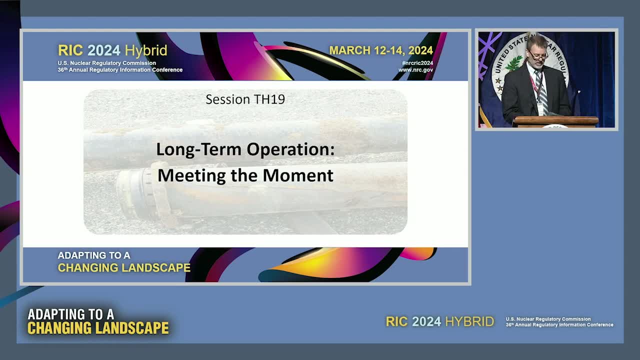 and the NEA OECD Working Group on Integrity and Aging of Cards and Aging of Components and Structures. Also note that here in the US we are currently updating our SLR guidance with a planned issuance date of January 2025.. We plan to have a public meeting next month in April. 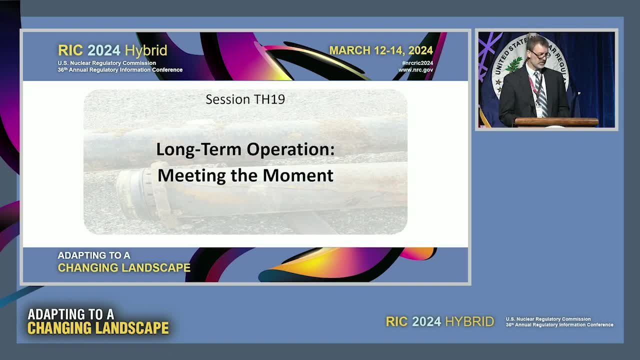 to discuss how we resolve the public comments on the draft documents. So look for that notice coming out before long. And lastly, research. our Office of Research will be conducting a workshop this fall on planning for research for operating in the US and the US and beyond 80 years. 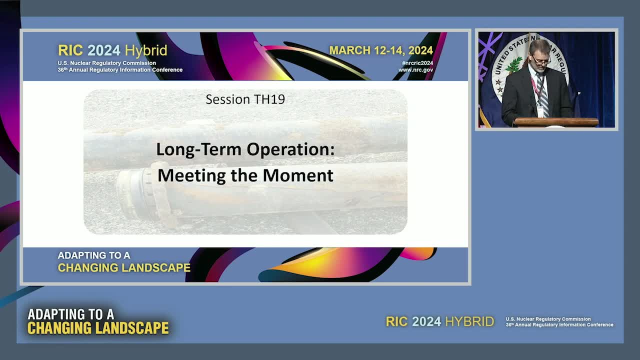 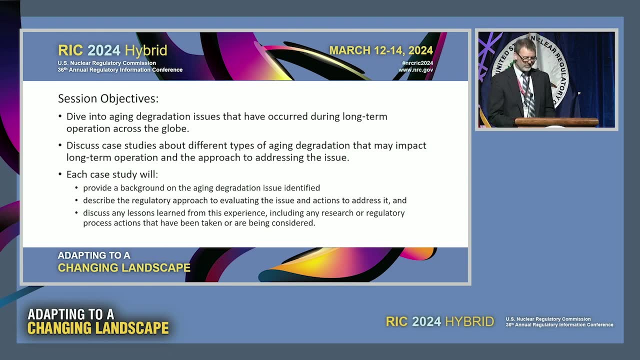 So if you're interested in that, please stop by and see one of us after the session. So in this session we'll dive into aging degradation issues that have occurred during long-term operation. This session will discuss case studies about different types of aging degradation that may impact long-term operation. 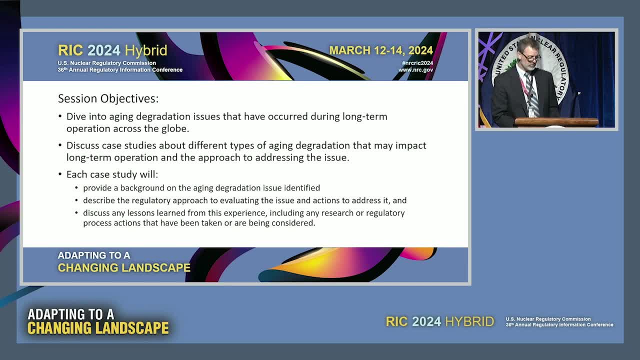 and the approach to addressing the issue. Each case study will provide some background on the aging degradation issue identified by the US Department of Education. the US Department of Education, the Department of Health and Human Services and the Department of Health and Human Services. 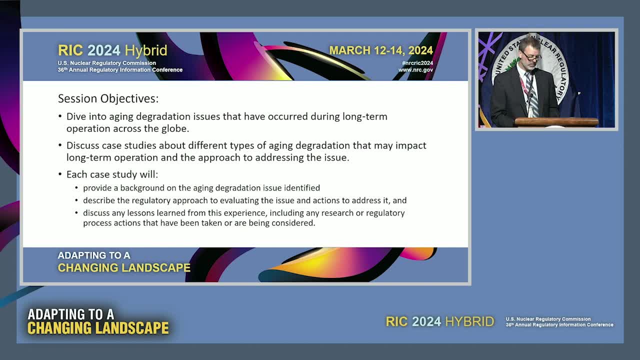 The program will discuss the regulatory approach to evaluating the issue and actions to address it and discuss any lessons learned from this experience, including any research or regulatory process actions that have been taken or are being considered. Following the presentations, we'll have a few predefined. 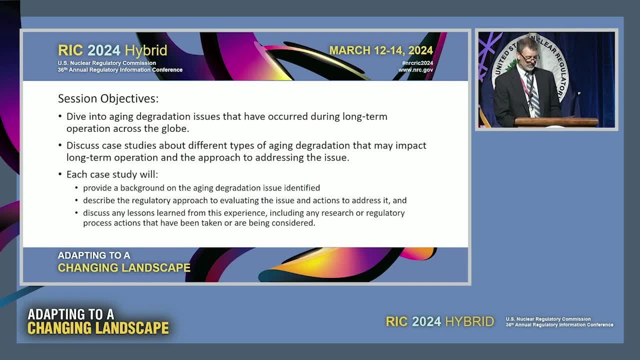 questions for the panelists, which will be followed by audience Q and A. So a few notes about Q and A's, But first, since this is the first session of the day, please remember to silence your electronic devices. The Q and A portion of this session will be: 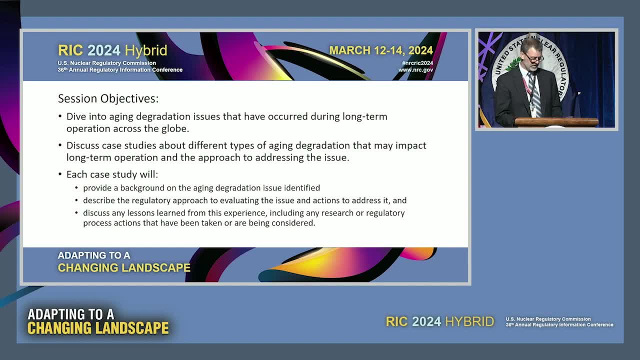 through electronic means for both the virtual and in-person attendees. for those of you in the room here, you may have scanned the QR code from the displays out in the foyer, but if not, please take a moment and scan the QR code. you'll see up on the screen. you'll then be redirected to the specific 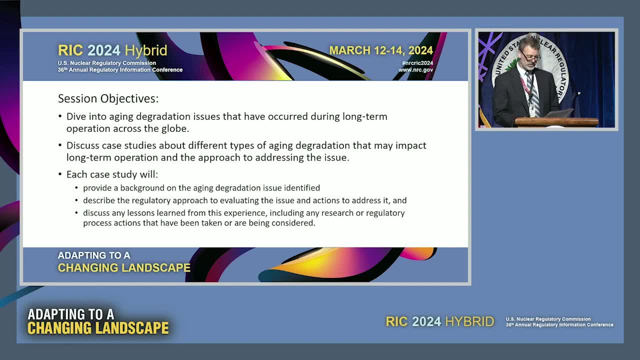 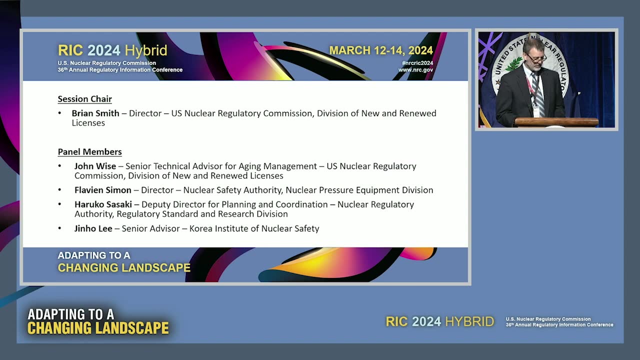 session page for Q&A. for those of you joining virtually, once you've logged on to the virtual conference platform and join the session, there is a tab for electronic Q&A. okay, so I have four speakers with me today on the panel. the first speaker will be John wise. dr wise is a senior technical advisor and the 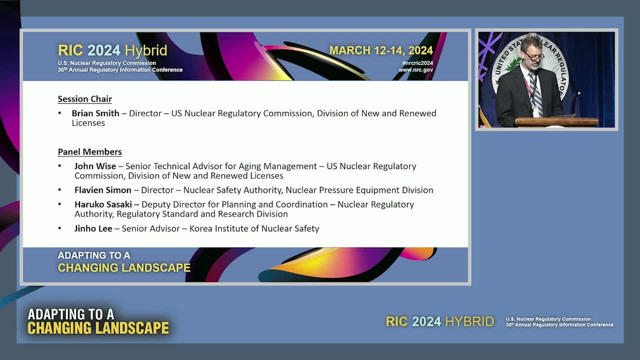 NRC division of new and renew licenses. he supports the resolution of technical and regulatory issues on a broad variety of materials topics, with particular emphasis on long-term plant operation and aging management. his career at the NRC has also included positions as a manager of the NRC and as a director of the NRC, and as a director of the NRC and as a 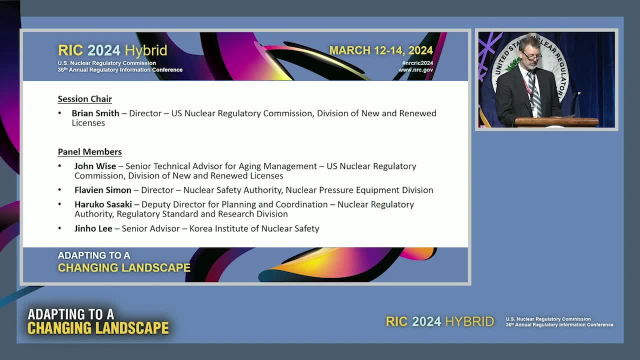 materials, technical reviewer for reactors and spent fuel storage and transportation systems. prior to joining the NRC, John held metallurgical engineering positions in the steelmaking industry and in failure analysis consulting. he's a graduate of Michigan Tech and Northwestern universities. our second speaker will be Flavia and Simone. mr Simone studied mathematics and 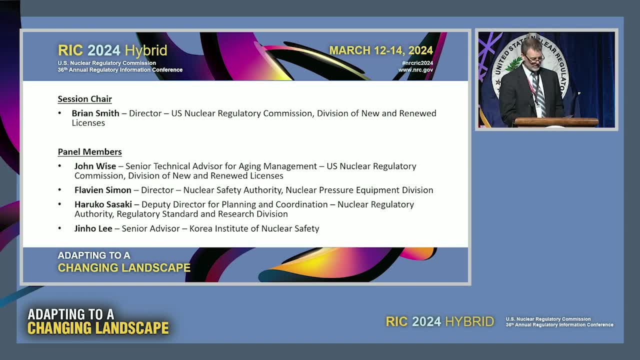 fundamental physics at a coal polytechnic in France. after graduating from this school, he decided to join the French civil administration. he first became chief of a risk prevention department and a French regional administration, his team being responsible for the control of the hazards caused by industrial activities and their impact on the environment. he 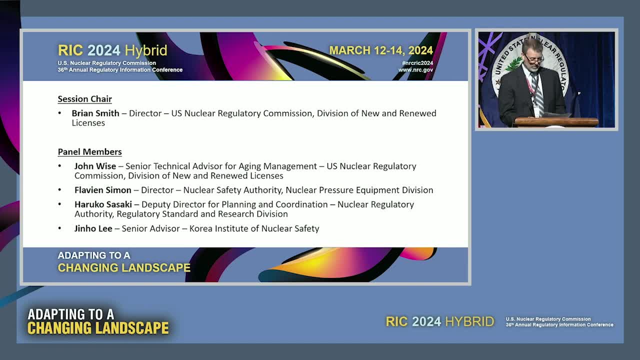 then joined the French nuclear safety authority, a SN, becoming the deputy director and later the director of the pressure vessels division. in this division they oversee the control of all matters related to the design, manufacturing and operation of pressure vessels and piping and civil. the recent years they have been particularly involved in the control of the manufacturing of the. 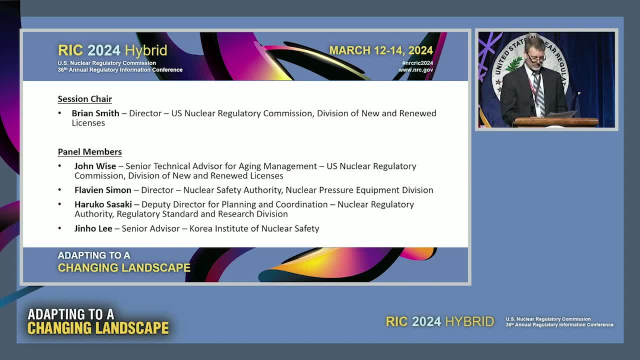 equipment of the EPR and EPR2 types of reactors, the stress corrosion, cracking issue and the aging of reactor pressure vessels and cast stainless steel components. Our third speaker will be Ms Haruko Sasaki. Ms Sasaki is currently a Deputy Director for Planning and Coordination in the Regulatory. 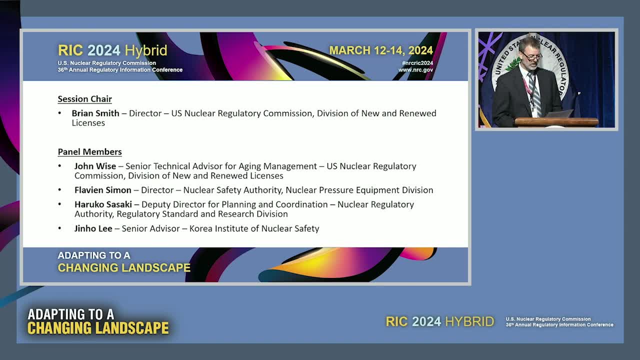 Standard and Research Division in the NRA in Japan. She has been with the agency for 10 years and supports the technical evaluations of the codes and standards and coordinates the public meetings related to the various technical issues. She was a Vice Chair of the Codes and Standards Working Group of MDEP and a member of the 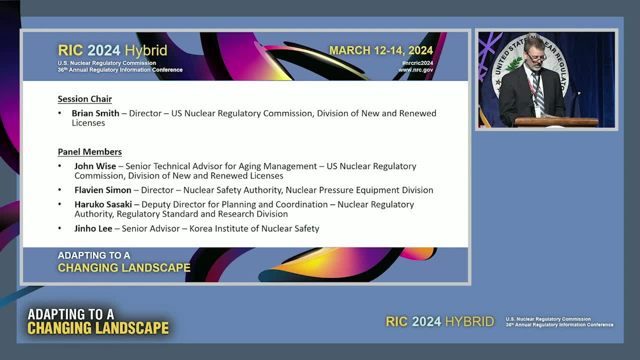 Working Group on Codes and Standards of the CNRA. Our last speaker will be Jinho Lee. Dr Lee serves as a Senior Advisor at KINS, the Korea Institute of Nuclear Safety. He joined KINS in 2000 and has held various key management and leadership positions in. 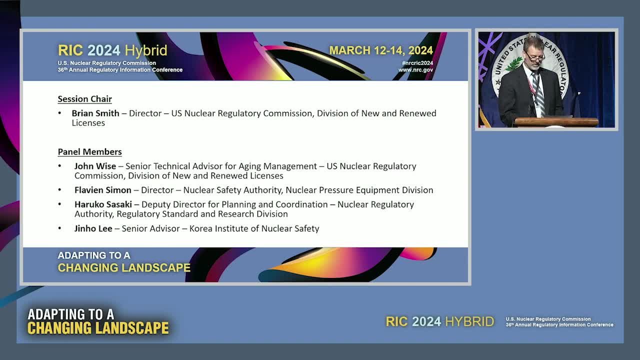 the state, including Executive Vice President from 2018 to 2021 and Director of Safety Research Division. He also served as the Head of four different departments, including International Project Management, International Cooperation, Mechanical and Materials Engineering and Legal Affairs and Safety Standards. 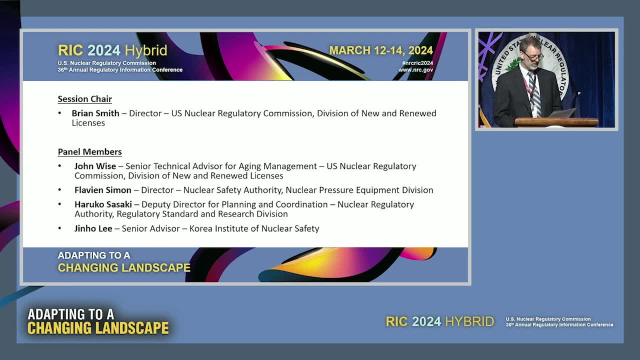 For 12 months, starting in May 2004,. Dr Lee visited the Argonne National Lab and performed joint research on steam generator tube integrity. Dr Lee also served as a member of the IEA Commission on Safety Standards and Research. Dr Lee also serves as the Executive Director of the NRA, which is the NRA's Native Apprenticeship. 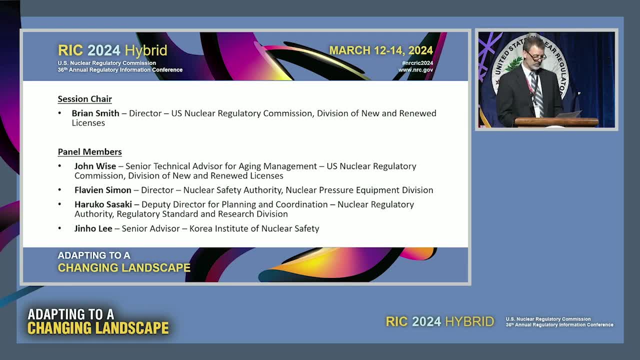 and Research Association standards, a nuclear safety standards committee from 2018 to 2023.. Before joining KINS, he served in the military as a professor in mechanical engineering department of the Korea Military Academy. He received bachelor's, master's and doctoral degrees in mechanical engineering from Sungkyu. 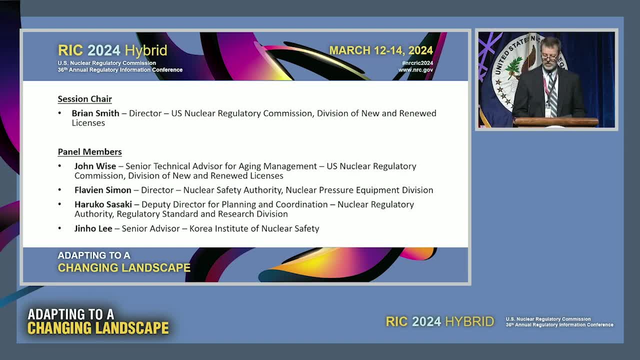 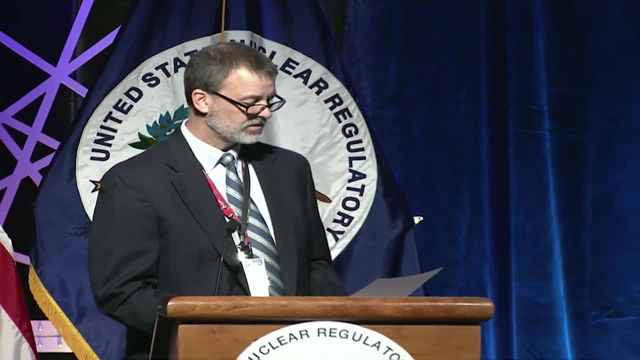 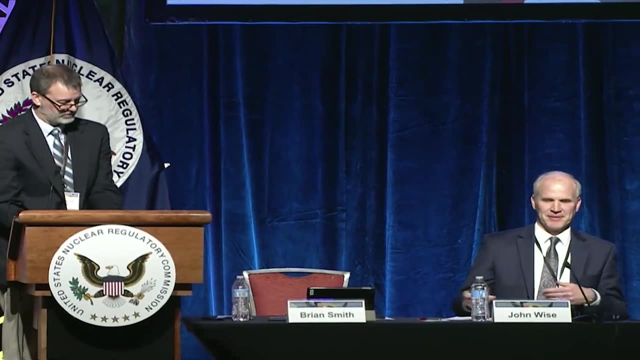 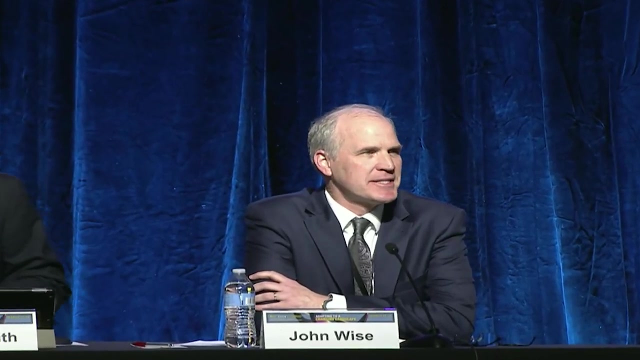 Kwon University in the Republic of Korea. Our first speaker today will be John Wise. the topic of managing selective leaching during long-term operation. Thank you, Brian. Good morning. This morning I'm going to explain the NRC's approach to addressing emergent aging issues. 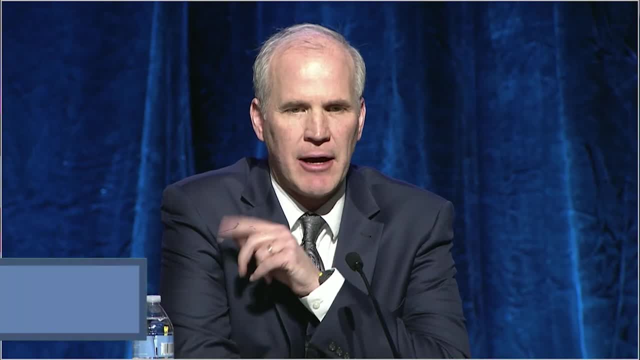 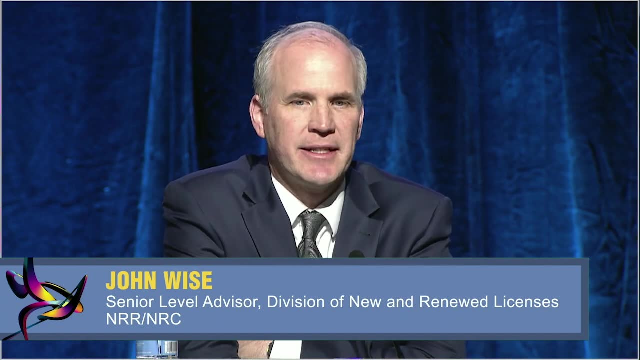 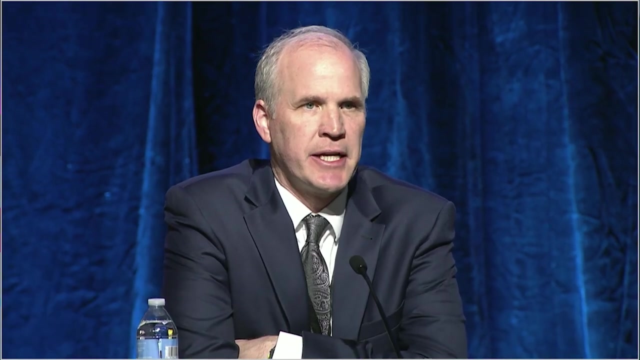 in long-term operation And, as Brian outlined in one of his first slides, the idea is to walk through this case studies, And so what I'm going to do this morning is I'm going to use selective leaching, The aging mechanism, As an example of how we work through an emergent aging issue, you know. so I'll talk a little. 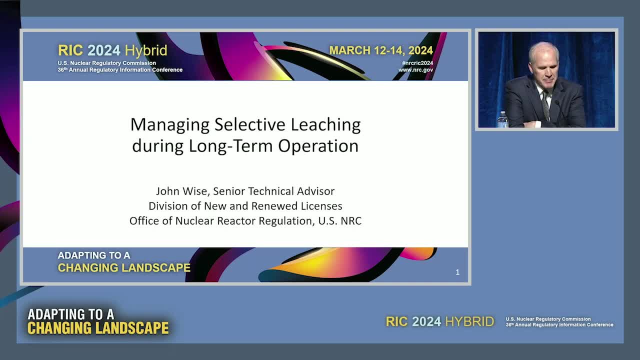 bit about the background of this particular aging mechanism, But then discuss how the NRC, you know, takes such an issue to evaluate it, assess its implications for the wider industry and then make decisions about whether or not that experience needs to be shared more broadly. 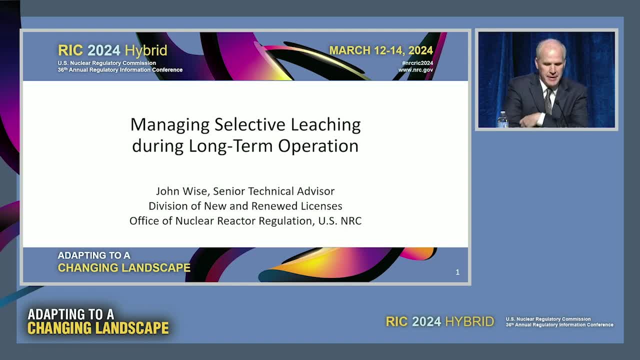 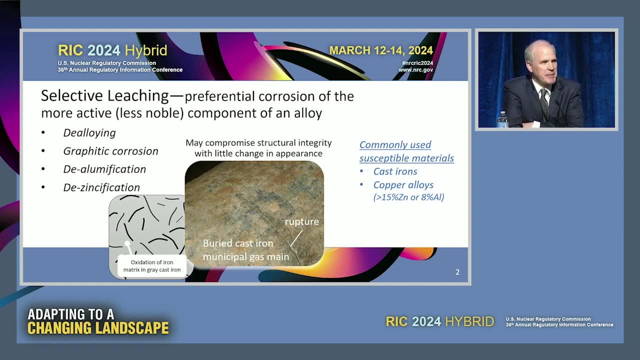 Or whether our regulatory programs need to be So. first, just a couple of minutes on selective leaching, to bring everybody up to speed on this aging mechanism. This is a generic term. It's often it goes by many other names as well. 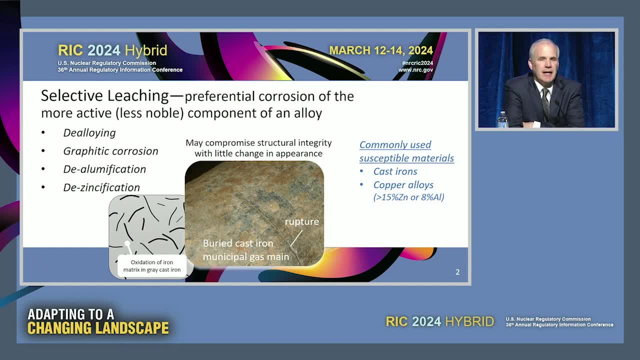 It's very frequently referred to as de-alloying. There are also very specific terms that are used when you're talking about a particular material. Usually, in the case of cast iron, this would be calligraphy- A bit of corrosion, And you can see the other terms there listed. 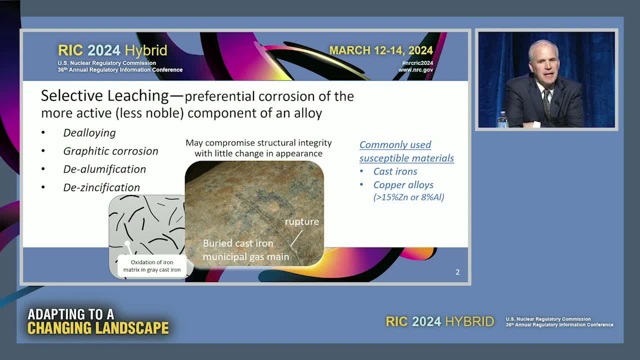 De-allumification, for example, for copper-based alloys. But what all of these mechanisms have in common, regardless of the material, is the feature that it represents a corrosion mechanism where, basically, you have a galvanic cell where one part of the microstructure acts as a sacrificial anode to the other part of the microstructure. 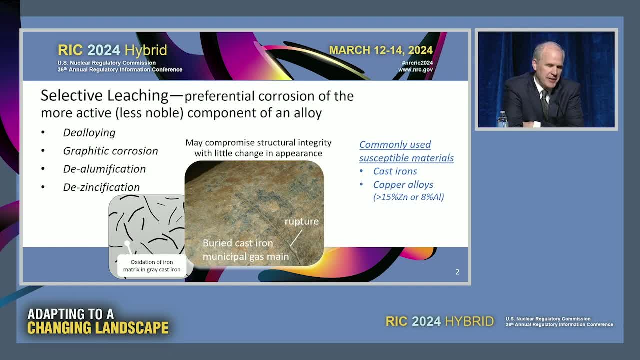 And so if you look at that example of cast iron And that, Yeah, That graphic on the bottom, In that case the iron matrix of cast iron sacrifices itself for the graphite flakes in the microstructure. And so, in the case of cast iron in particular, what makes this a particularly challenging? 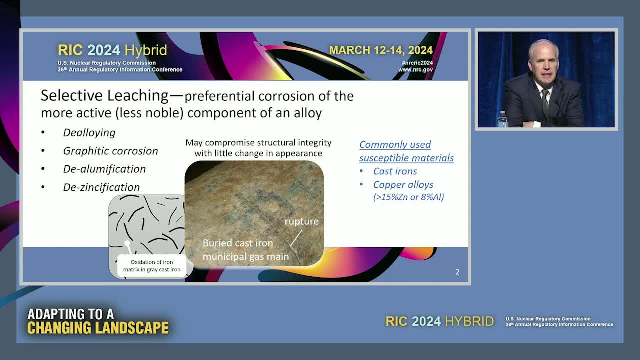 degradation mechanism is a couple of things. First of all, it can take a long time to show up. So you may have decades, Even decades of experience and without any indication that anything is happening, But then it emerges later on, after many years. 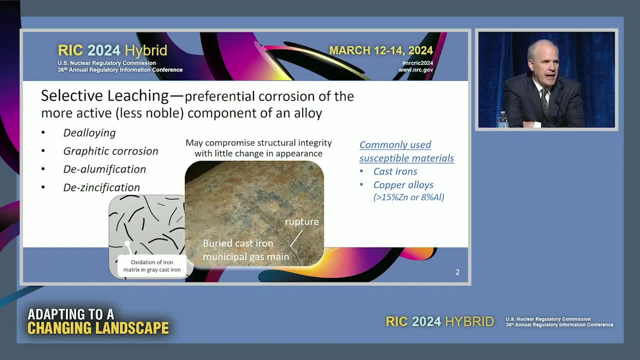 And so recognizing that and planning for that in our aging management strategy is always something we have to keep in mind. And the other part about this mechanism- again in the particular case of cast iron- is you can get a significant loss in the structural integrity of a component without any really. 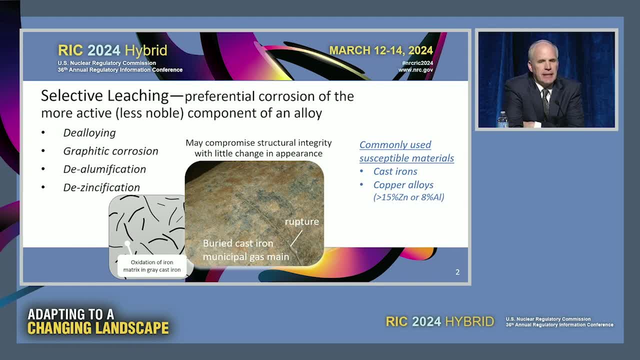 any visual indication that that has happened In that picture there you see, I took that picture and it's of a cast iron pipe in municipal gas main And I can tell you that you can see the rupture there and the pipe itself essentially lost. 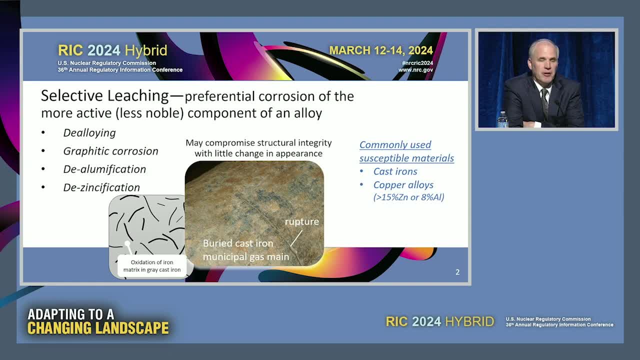 all structural integrity. It didn't have any toughness. But looking at it, If you had your hand on that pipe and even wrapping on it with your hand, you'd think it was a solid pipe. But in fact most of the iron matrix in that cast iron had been converted to iron oxide. 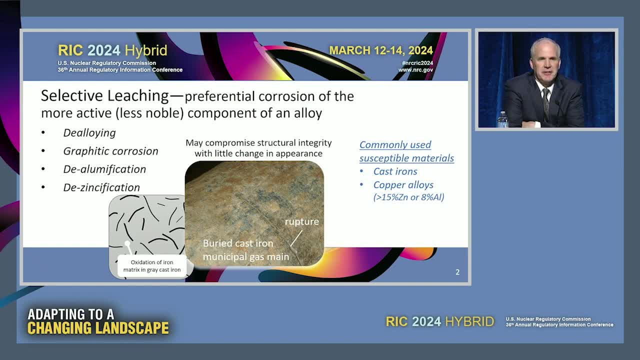 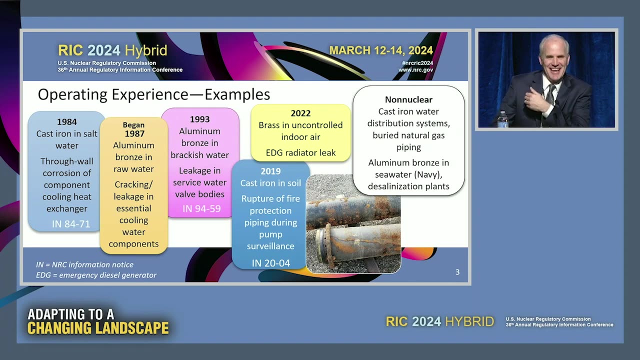 And it really didn't have any structural integrity, And that makes it a particularly hard aging mechanism to manage, just given that lack of visual indication. Next slide please. Oh sorry, I've got to tell myself the next slide. Come on, Brian. 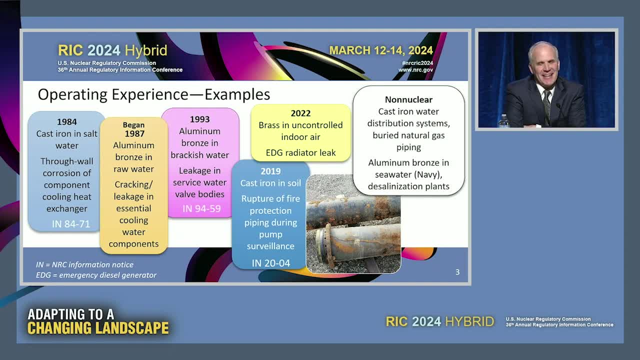 Yeah, So, yeah. So, just very briefly, we've had here's some examples of operating experience over the years associated with this particular aging mechanism. In the United States the experience tends to be associated with cast irons, But you see, aluminum bronze is also one of the materials that this occurs in. 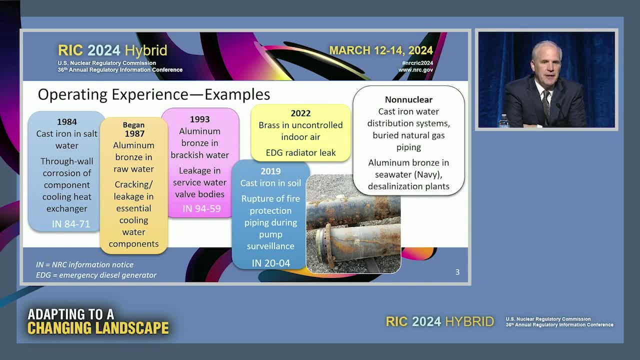 We've had experience in. in that particular case, the aluminum is lost in the material due to the selective leaching mechanism, And my intent isn't to go through one by one, But just recognize that we've experienced, seen instances of selective leaching over. 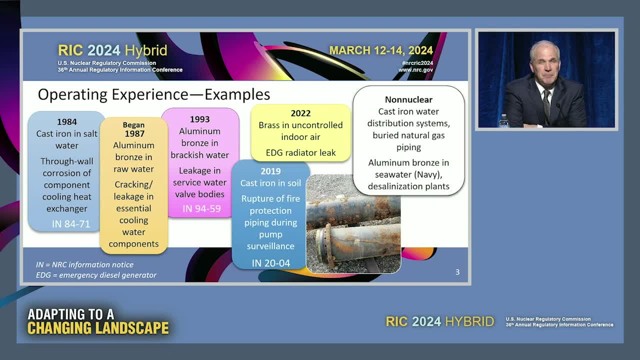 the years And in those cases where we felt that the experience was warranted, Yeah, Yeah, And in those cases where we felt that the experience warranted a broader communication. you will see those indications of an information notice or IN numbers at the bottom. 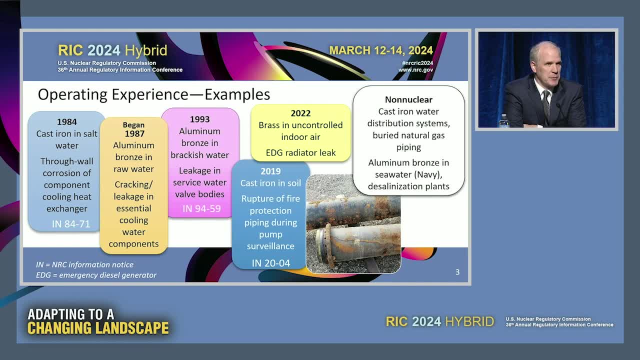 And those are cases where we felt that the experience was significant enough that we, as a regulator, felt that we needed to issue a communication to the broader industry for their awareness. And finally, on the far right-hand side, we talk about the experience in the nuclear industry. 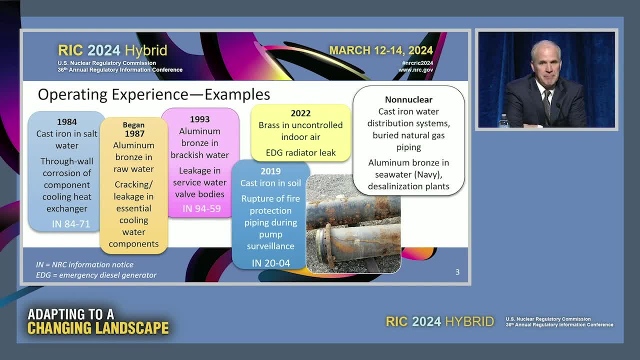 But it's really the non-nuclear operating experience in many cases is the most telling and most helpful for us to learn about this aging mechanism Because the selective leaching of cast irons in water distribution systems. in the United States, particularly the East Coast cities, have some really old cast iron piping systems. 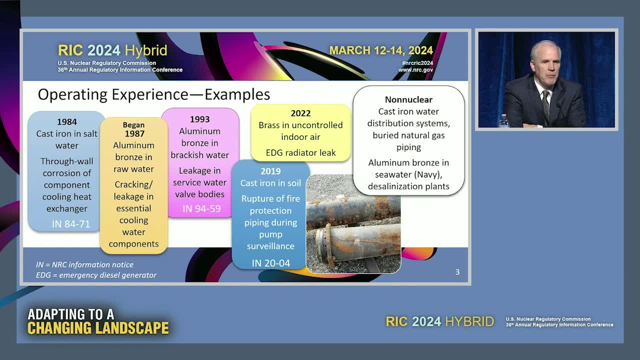 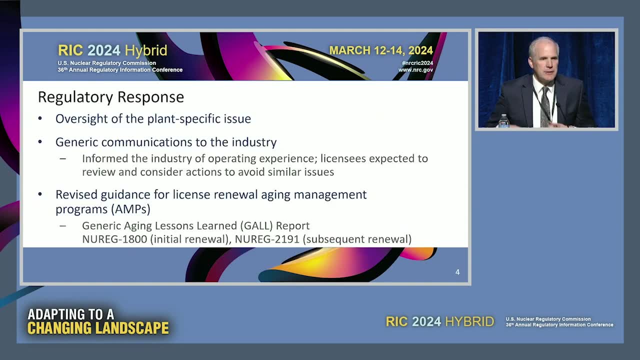 They provide a lot of information that we use to inform how we address selective leaching in the nuclear area. So, as with all instances of operating experience, the NRC, through its operating experience program, goes through a number of steps. We collect the operating experience. 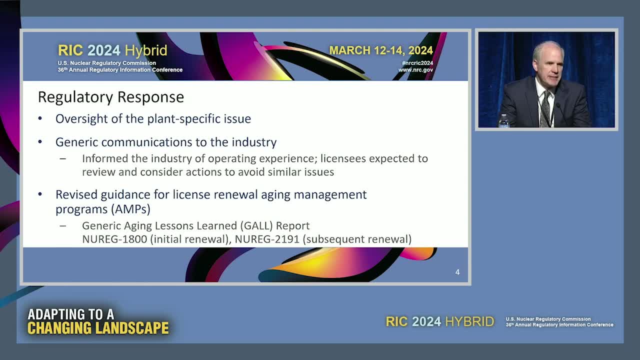 We review it, assess the implications, the safety significance, applicability to whether the operating experience is unique to the plant or applicable to the wider industry, And then we need to make a decision as a regulator whether we feel that there is a need to broadly 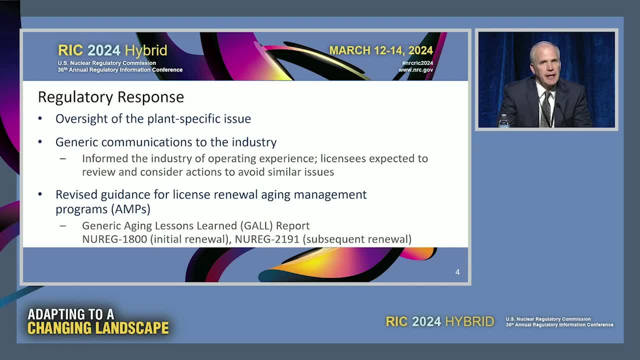 communicate this experience to the broader industry and whether or not our own regulatory programs need to be adjusted. So, typically, what's happened in the case of the selective leaching mechanism? we've obviously, case by case- our inspectors in the regions handled a plant specific issue in particular. 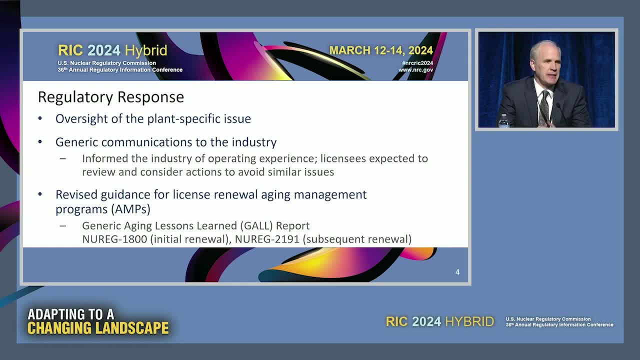 But generically we've assessed that information and, as I showed in the prior slides, we've issued communications to the industry when we felt that it needed to be broadcast And we generally have used these information notices and that's just one of our communication. 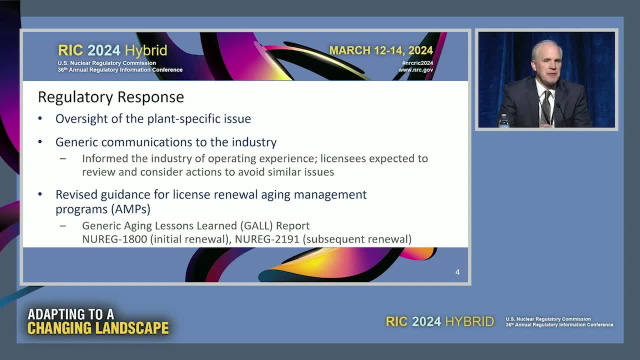 vehicles that push the information out to the industry, with the expectation that each plant will take that information and themselves evaluate it and consider whether or not it needs to lead to specific actions at their plants. And we have different types of communications that we use. Information notices are one, but the different types of communications vary by the type of 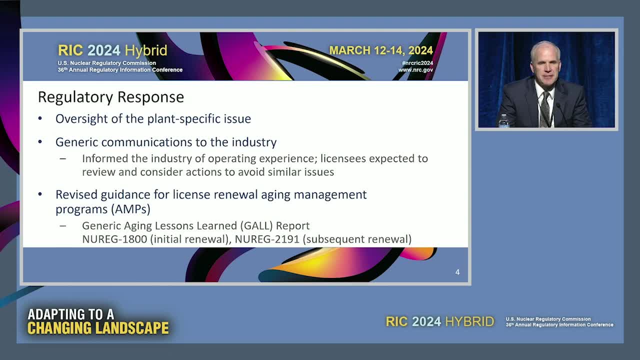 information we wish to communicate and the expected actions of the plant. And finally, the bullet down at the bottom is really what we're talking about a great deal today is long-term operation, and when we talk about long-term operation, we're usually talking about aging management programs. 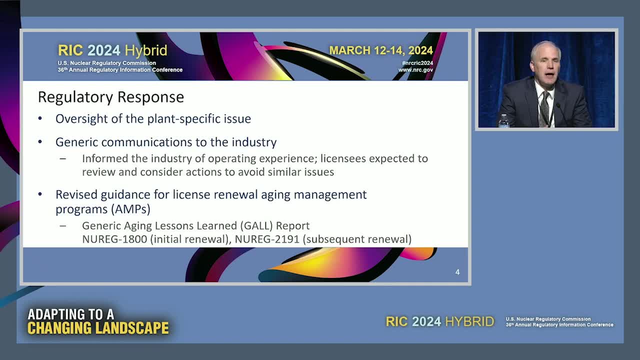 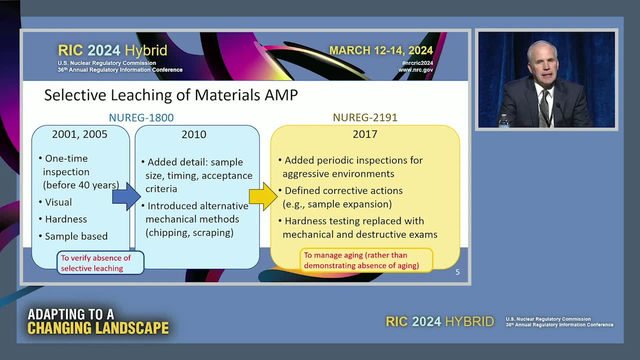 And so we look at this operating experience to determine whether or not our own guidance for aging management needs to be revised, And that indeed has happened. I don't want to get into all the details of this slide, but just broadly. we have our 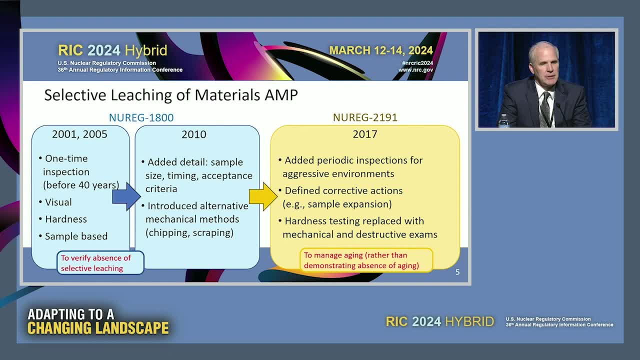 generic aging lessons learned report which provides example acceptable approaches to manage aging, And we have a program that We provide in our Gall Report and that program has evolved over the years as we've learned more about this particular aging mechanism. The blue boxes represent our initial license renewal or 40 to 60-year guidance. 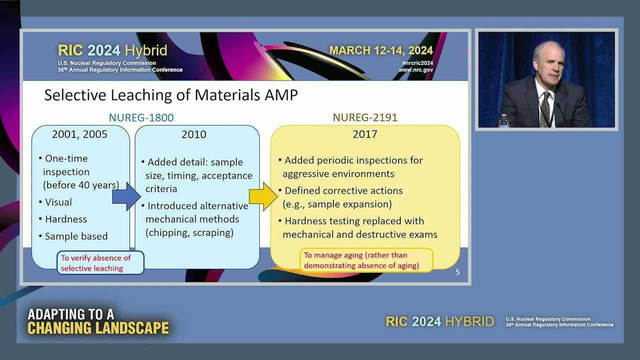 The orange-yellow box is our subsequent license renewal guidance for 60 to 80 years And, as you can see early on, this program was one-time inspection You did When you entered year 40, you know 40-plus at your plant. you selected a sample of components. 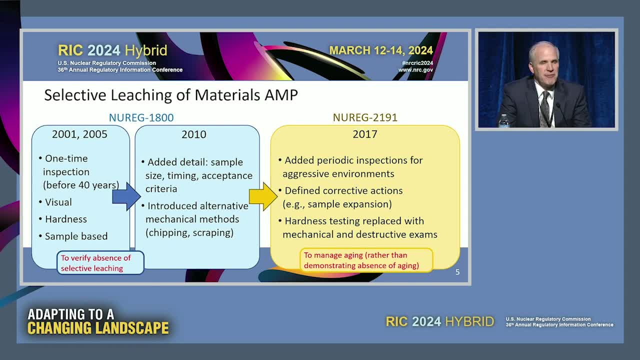 at your plant to determine whether or not really to verify that this wasn't an issue at your plant. That is the program And you can see there's a. It had a combination of visual inspections but, as we already discussed, you need to do. 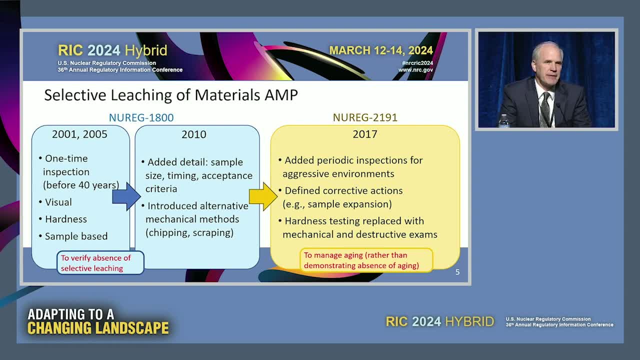 some sort of mechanical inspections as well to really understand the structural component of this aging mechanism. But what we've learned and what we've seen at the The prior slides was we're kind of beyond in many materials just verifying that selective leaching isn't happening, because in many cases, for particular materials, in particular environments, 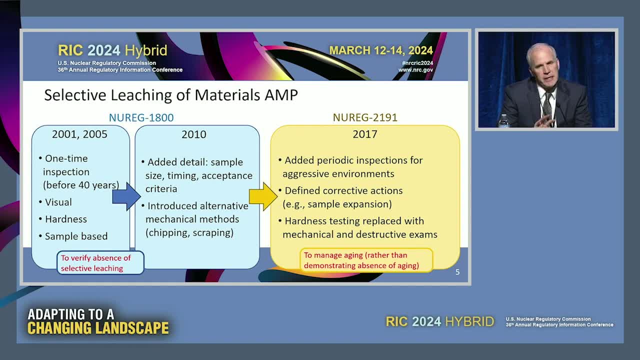 we know it is happening And so over the years and as you go to the right-hand side of the page, our aging management approach has moved from a one-time inspection to verify it's not happening to periodic inspections now Where we're really managing an aging mechanism. in many cases we expect to happen for specific 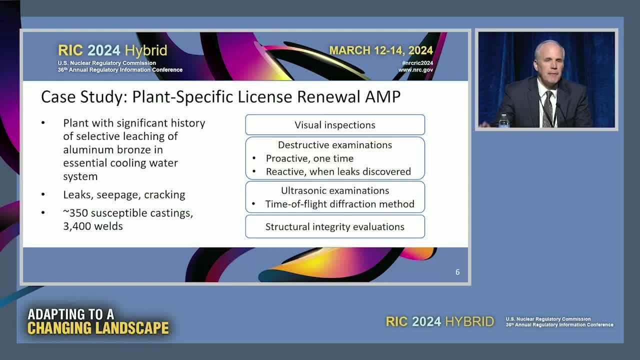 materials and environments. But that's our generic guidance And, plant by plant, there may very well be plant-specific considerations where that generic guidance doesn't work, And so in this particular case study I'm showing here in this slide, it was a plant that was. 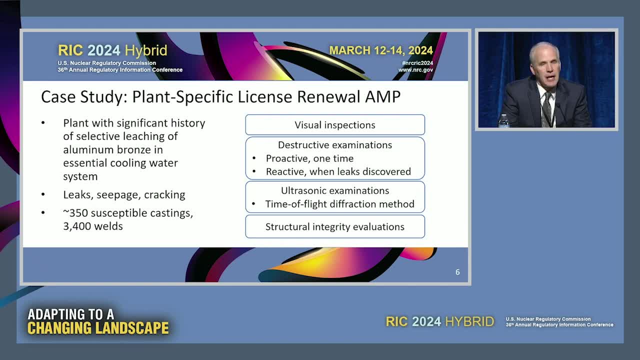 coming in for initial renewal- 40 to 60 years. They had a significant history of selective leaching of aluminum bronze And you can see the huge population of castings and welds that were considered susceptible to this aging mechanism. And, as I said in my prior slide, the 40 to 60-year recommended program was really just. 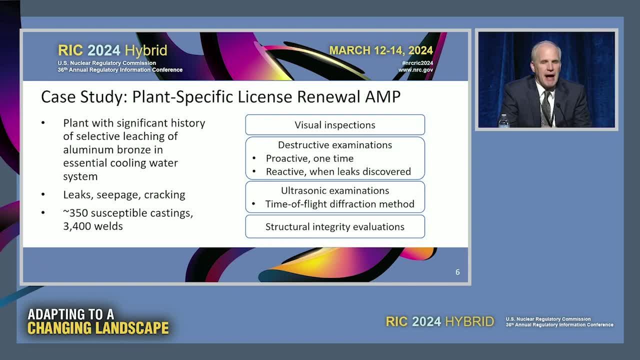 a one-time inspection to verify that it's not happening. Obviously, that's not appropriate in this particular case because it was happening, And so, in this particular case, the NRC staff had to work with the applicant to come up with a program to address the fact that it is happening and there's a very large population. 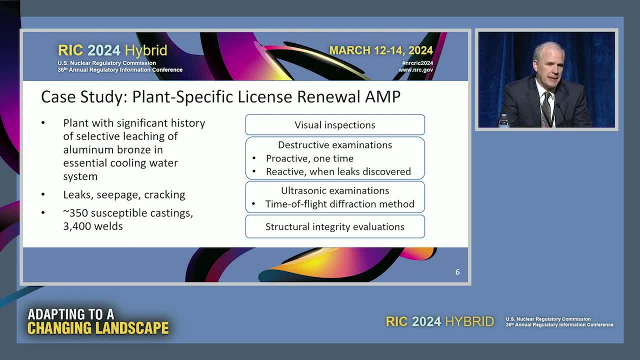 And this included, as you can see, a whole host of approaches taken, from visual inspections on most large population components to more intensive investigations, destructive ultrasonic on a smaller sample size, And so this represents a case which you know happens occasionally, where you know our 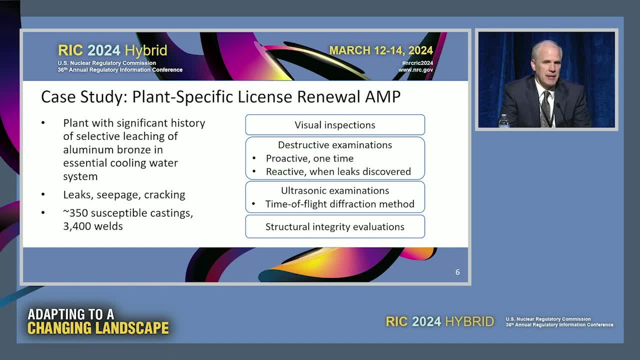 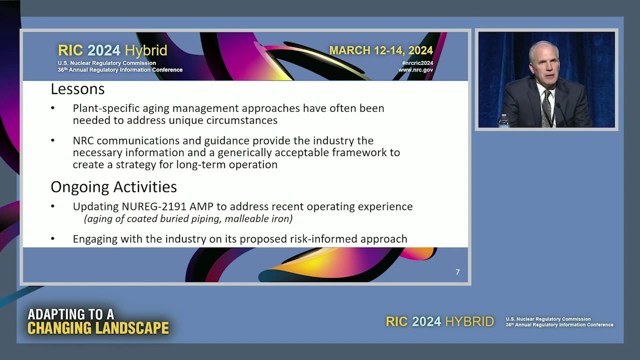 own recommendation. generic recommendation just isn't appropriate And in this case we'll work with the applicant to figure out the appropriate approach. going forward, So broadly, just the takeaways. you know the NRC we provide, you know we've used 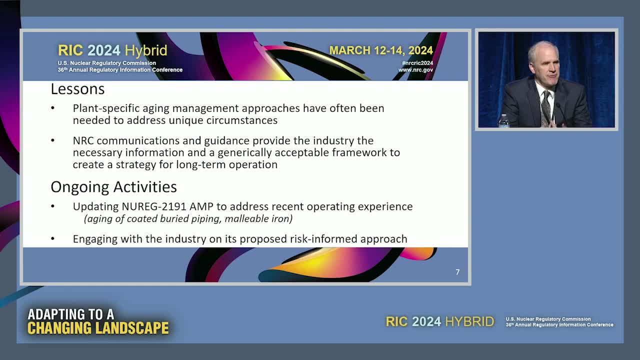 a lot of data. We've used a lot of data. We've used operating experience to refine our recommended aging management approach, and it has evolved over the years. It's become stronger, particularly in the cases where aging degradation is expected, But plant-specific approaches often will still need to be used. 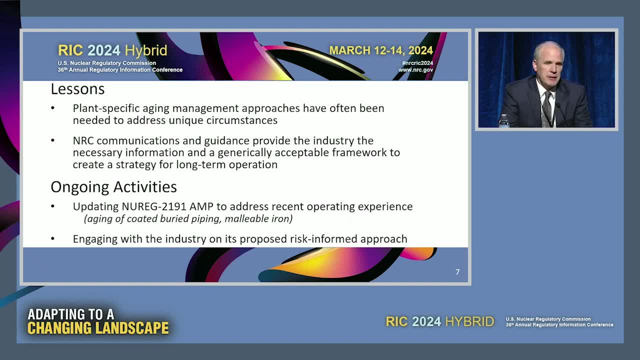 Ongoing activities. as Brian mentioned in his opening, we are currently have a few revisions to this particular aging management program, So we're working on that. We're working on a new program in our GAL report guidance that's out, that's draft that. 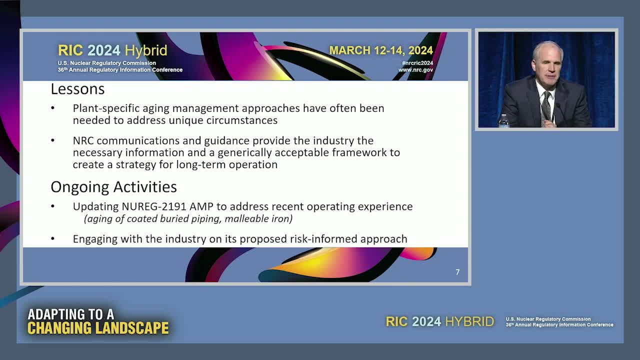 we're evaluating the comments right now And that includes a couple of smaller adjustments to the program to take into account new information that we've learned. And secondly, we have had discussions with the industry, particularly NEI, about potential taking a different look at this program where risk information might be brought in. 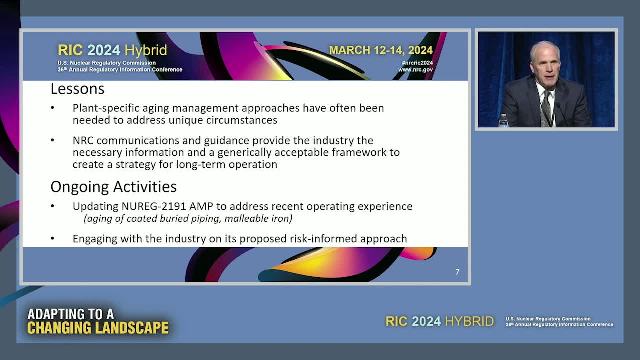 So we've taken into consideration to perhaps focus resources, I guess I'll say, on those areas that are most risk significant. And that's an ongoing conversation we've been having with the industry for the last few years and so that will continue, And so with that, that's it for me. 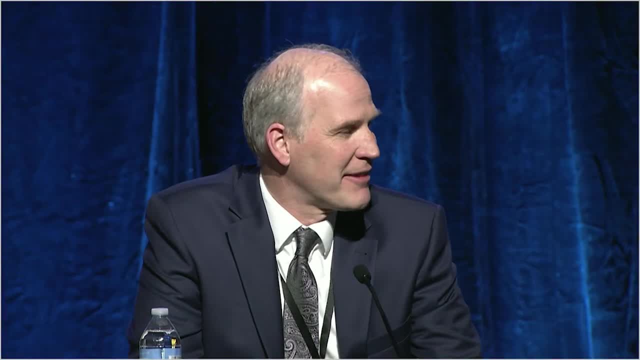 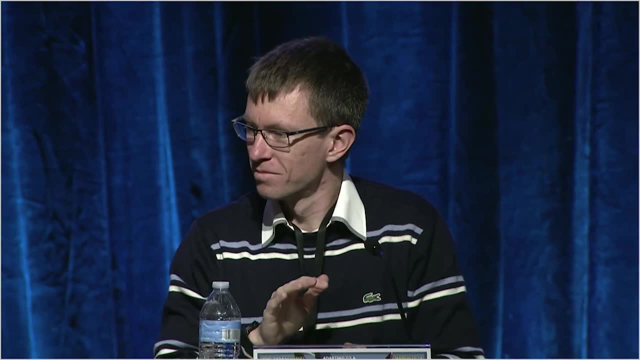 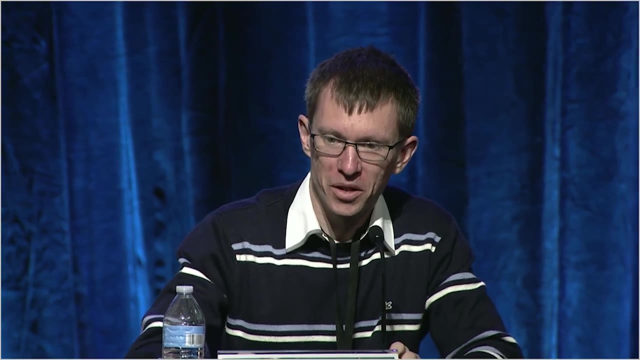 And thank you for your attention and I'll turn it over to Flavian. Thank you, Thanks, Brian. Thank you, Thanks, Brian, Thank you, Thank you, Thank you. So good morning. The topic I'm going to talk about is the degradations we faced in France on some cast. 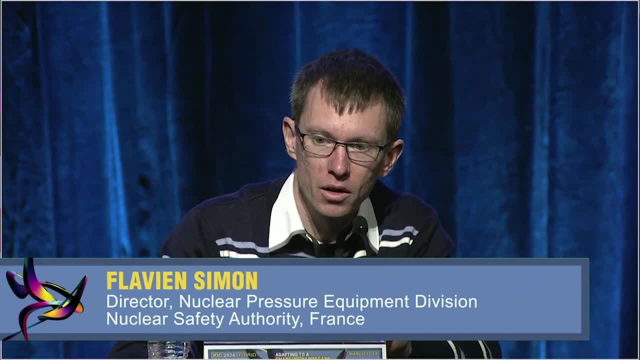 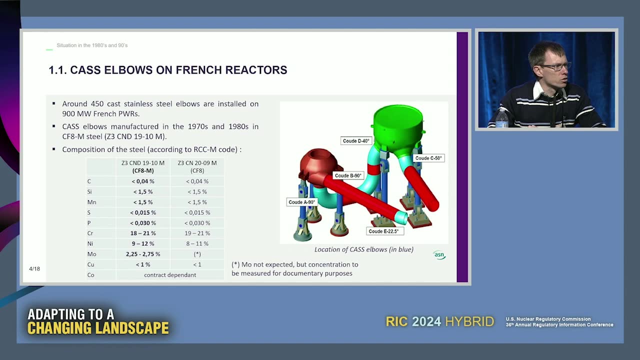 stainless steel elbows of our main current lines. So if I go over here on our oldest type of reactors, which some of you may know are of similar design as some Westinghouse, We have some elbows that are outlined in blue in the figure that were made of cast. 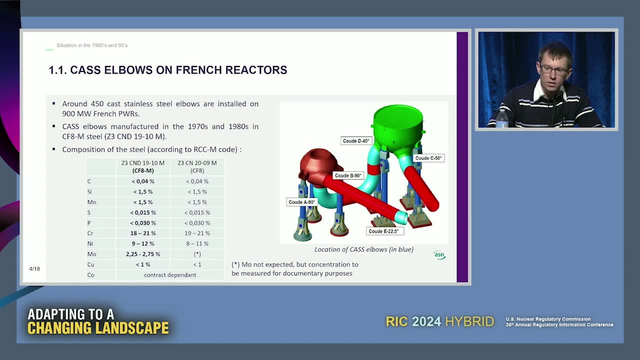 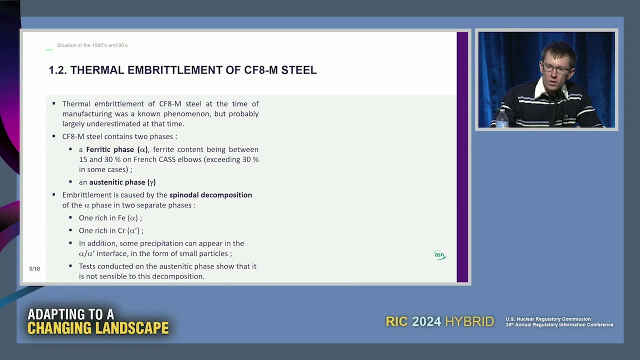 stainless steel in the 70s and in the 80s, And some of them were made in a particular steel with high molybden content that is particularly subject to some thermal edging mechanism, And the phenomenon is called thermal embrittlement. 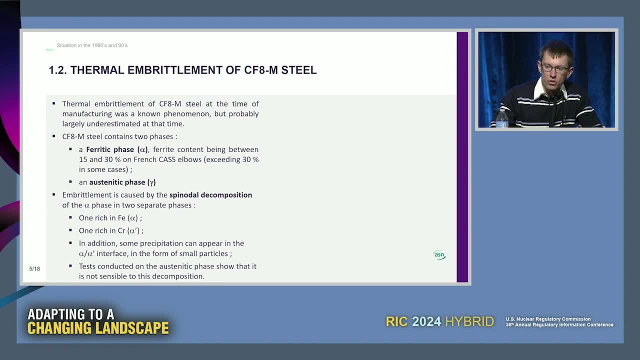 And it is because this type of steel, which is a duplex steel, is made of two phases: One is a non-stainitic phase, the other being a ferritic phase, And the ferritic phase is subject to embrittlement under the influence of the temperature. the 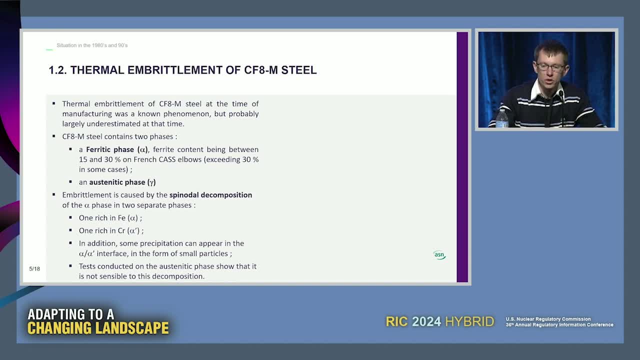 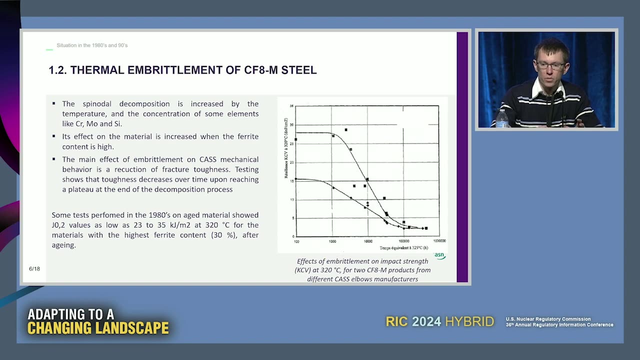 plant is facing during the normal operating conditions. There is, in fact a decomposition of these. There is a decomposition of this ferritic phase in two phases And basically the impact of this decomposition is that the mechanical behavior is modified and the toughness is dramatically reduced over time because of this embrittlement. 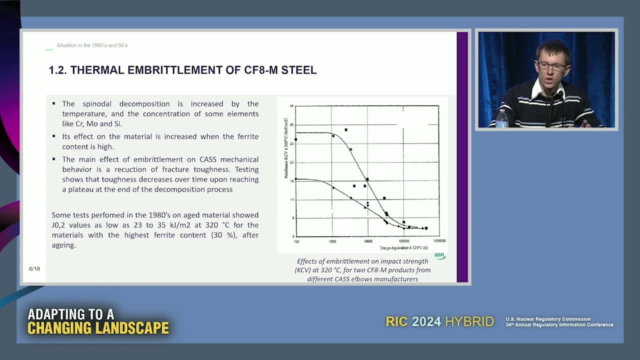 And so the rate at which it occurs is depending, obviously, on the temperature of the plant, And also it's depending on the concentration of some of the chemical elements within the steel, such as chromium, molybdenum or silicium, the elements that have an impact. 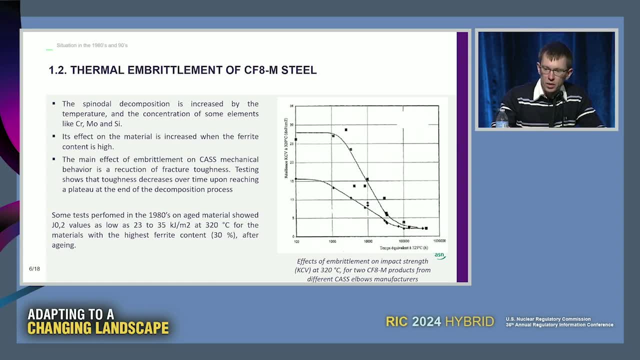 And, as you see on the right, I displayed the impact on sharpie, impact strength, And the values are evolving to a lower bound value that is rich for normal temperature conditions, After maybe 100,000 hours of operation, maybe 200,000 hours, which is the order of magnitude. 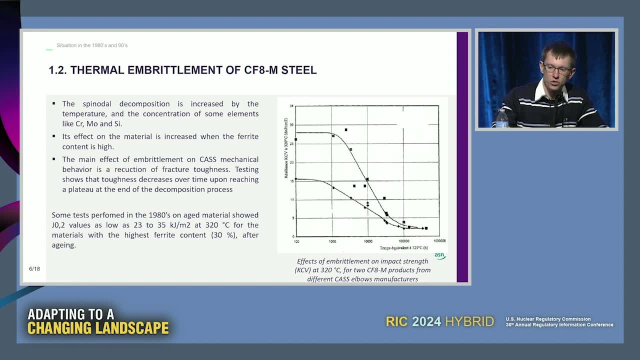 And I gave you also some toughness values that were measured in the 80s on some aged materials, some material that was aged in laboratory, And these were as low as 20 to 30 kilojoules per square meter, which is obviously very. 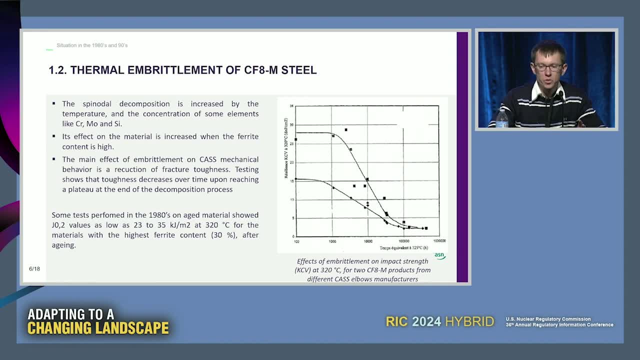 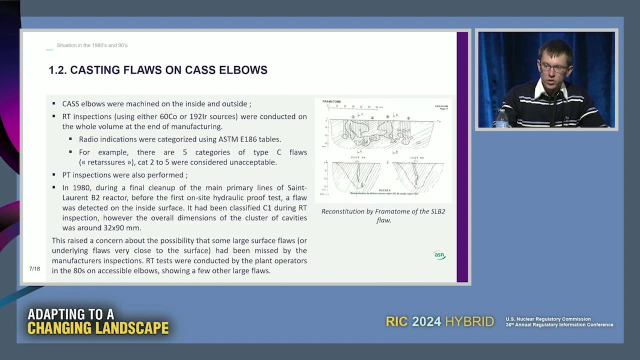 low And the toughness that we expect for currently the EPR reactors. on the main coolant lines it's above 100 kilojoules per square meter on the welds And it's even more for the base material. And the other issue was that in the 80s there were some big flaws that were detected on 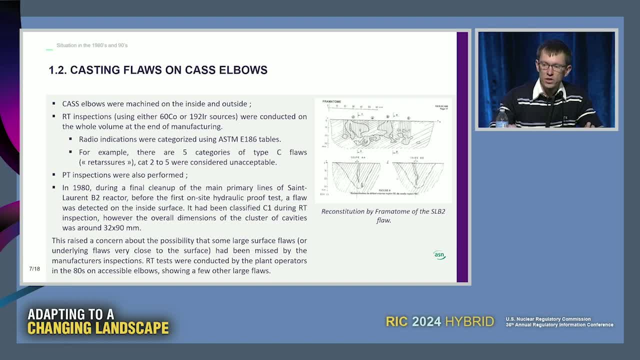 the cast elbows of the main coolant lines. There is a picture on the left. This is the main coolant lines. This is the main coolant lines- And on the right showing one of those flaws that was discovered by Framatome in the 80s. 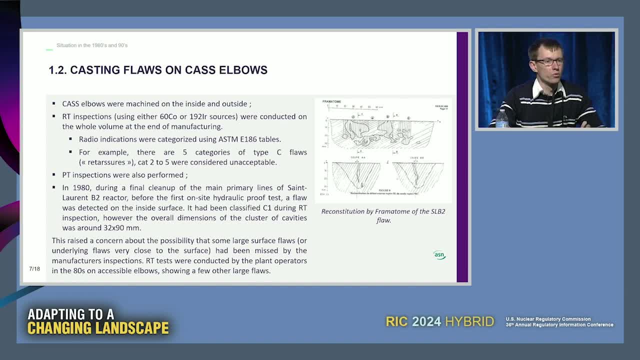 And the problem with these flaws was that they were not found during the non-destructive examinations that were conducted by the manufacturer. They were found by EDF just before the start of those plants. So it raised a concern for the ISN because we were knowing that the material was subject. 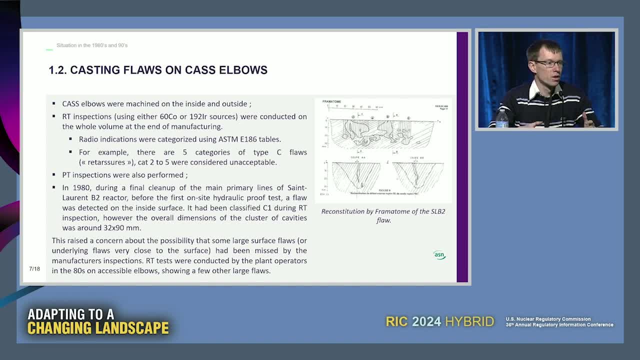 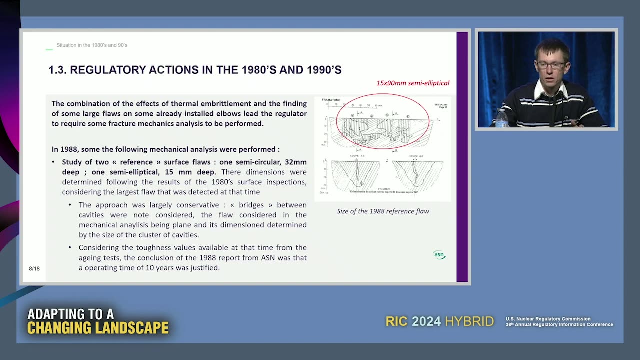 to a degradation that was impacting its toughness a lot And that there could be a risk of some flaws that were not discovered by the manufacturer and kept within the material. So the action of the ISN at that time was to ask our licensee, EDF, to assess the impact. 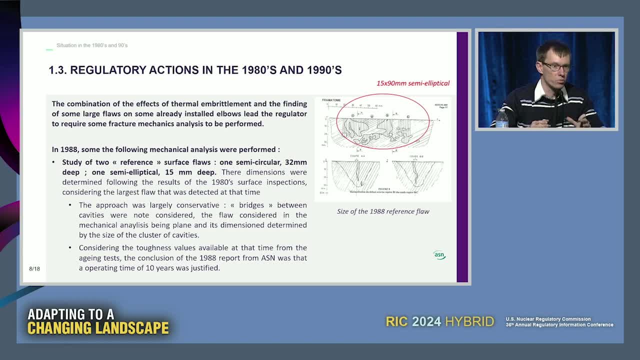 that it could have on the structural integrity of those elbows by doing some fracture mechanics computations, And the first approach was very conservative because we asked them to study the impact what was called the reference flow, and the dimensions of these flows would be a dimension that would cover the size of the biggest flow that was detected in the 80s on. 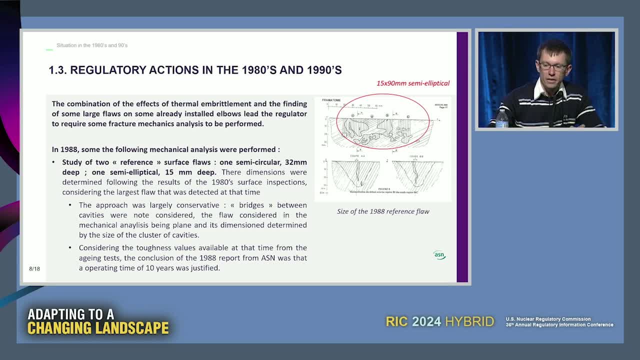 the elbows and the, at that time, the the toughness values they were. they were determined using some first formulas that were designed by edf in order to try to predict the effect of embrittlement, and the conclusions at that time was that an operating period of more than 10 years was. 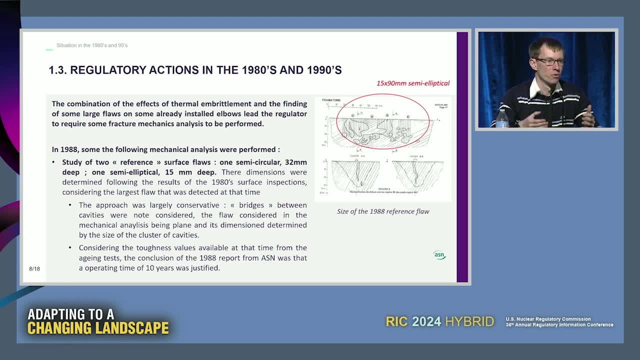 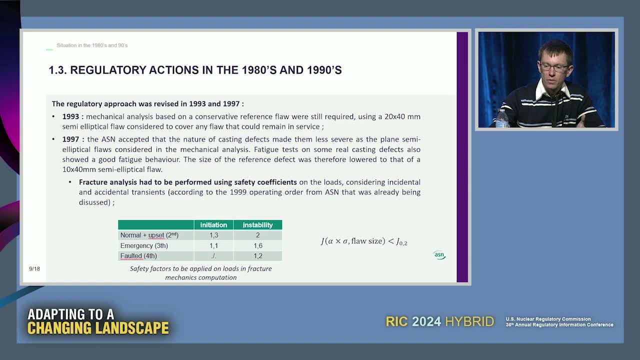 justified. but obviously this is way lower than the, the amount of years we operated the reactor, the reactors now. so there were some further studies that were done and there were two things that were assessed by the- the isn in the 90s. first, considering the, the flow that needed to be, 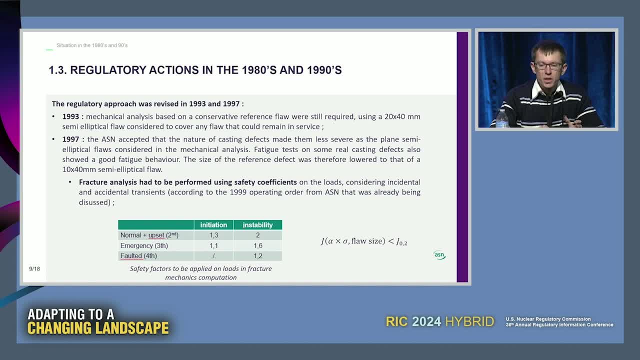 considered and and and. in those fracture mechanics computations, we accepted to reduce the size of this so-called reference flow, and the main reason behind that is that the flows we can expect in a cast material are not as harmful as, for example, a fatigue crack, the fatigue cracks that are used when determining. 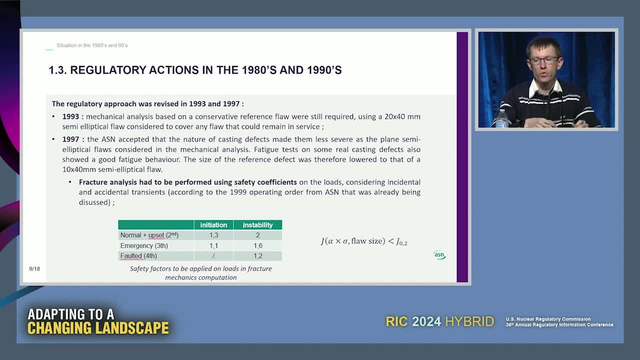 the toughness of a given material. so we accepted to use a reference flow that was in fact smaller in dimension, that was not as harmful as, for example, a fatigue crack, the fatigue cracks that were used in a cast material. so we accepted to use a reference flow that was in fact smaller. 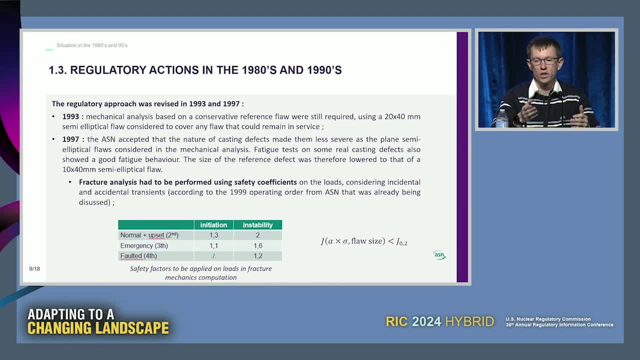 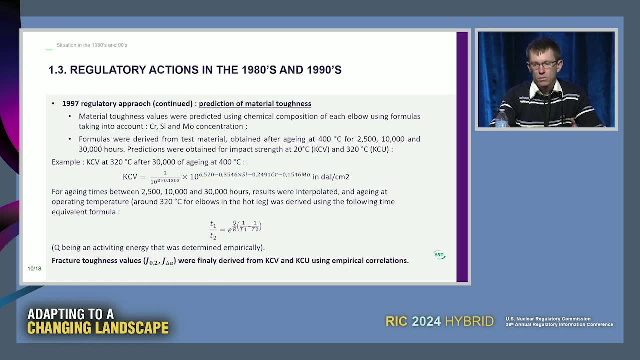 than the, the, the flows that were observed in some of these elbows and the. the other aspect was that isen asked edf to improve the way fracture toughness was predicted under the effect of embrittlement. so i gave in in the presentation some examples of the formulas that were used in 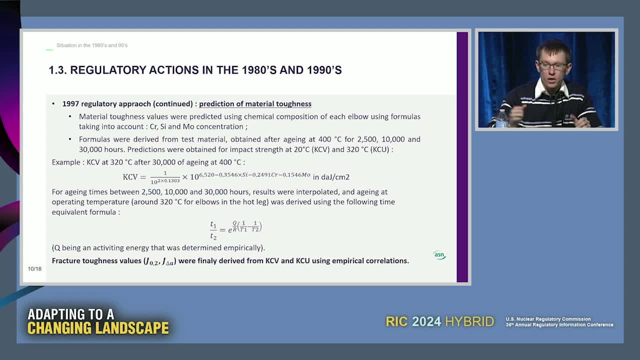 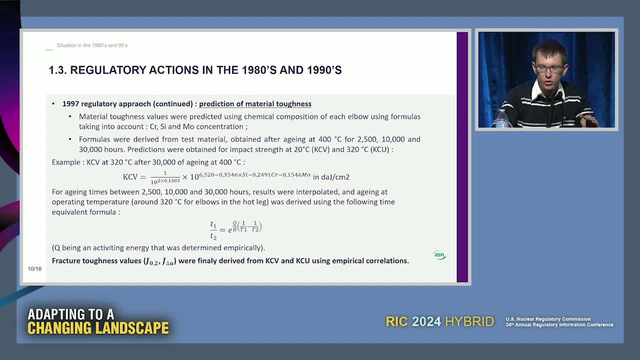 they were derived from tests that were done in the 1990s and was aged in the laboratory at different temperatures and for different aging times, And the principle behind those formulas being that EDF could predict some values for sharpie impact strength and then using some empirical correlation. 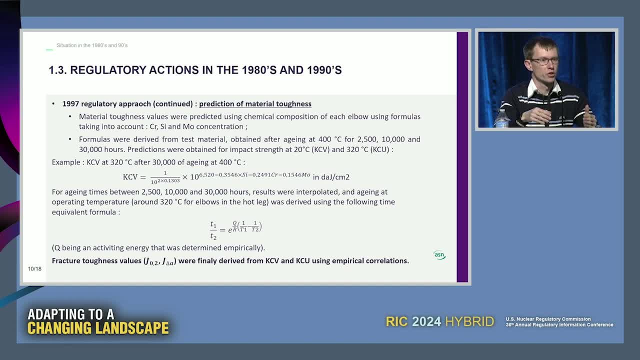 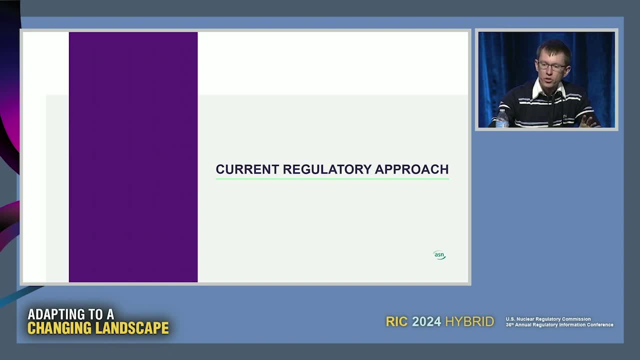 try to predict the toughness of the material based on the predictions on the impact strength. So that was the initial approach in the 80s and in the 90s. The issue with that approach was that the formulas that were used at that time 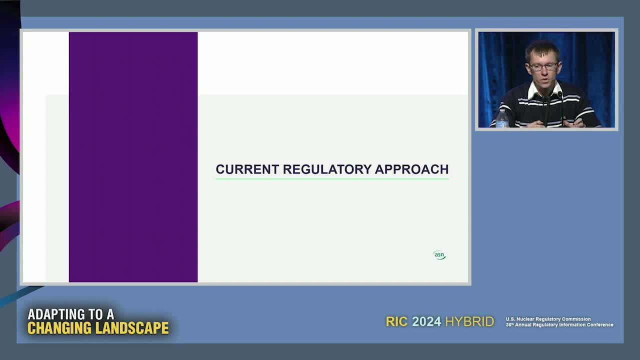 they were not taking into account test material that was representative enough for long-term operation, And in the 2000 and 2010s we had reactors that were reaching 30 and even 40 years of operation and the question raised by ISN was: 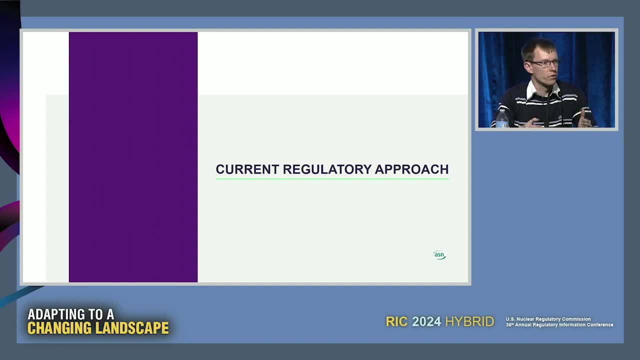 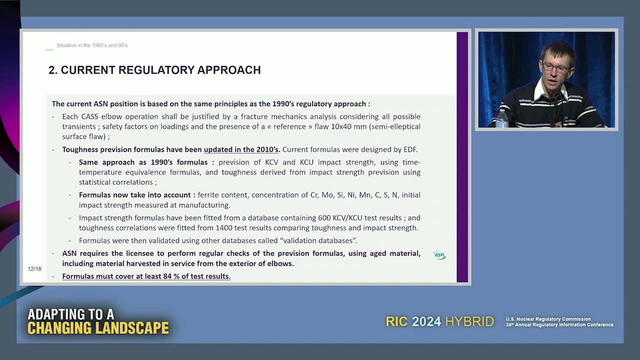 okay, can we reliably predict the toughness of those materials? Okay, can we reliably predict the toughness of those materials up to maybe 60 years of operation? because we were starting to think about those 60 years of operation for the French fleet, And so ISN asked EDF to launch a very important program. 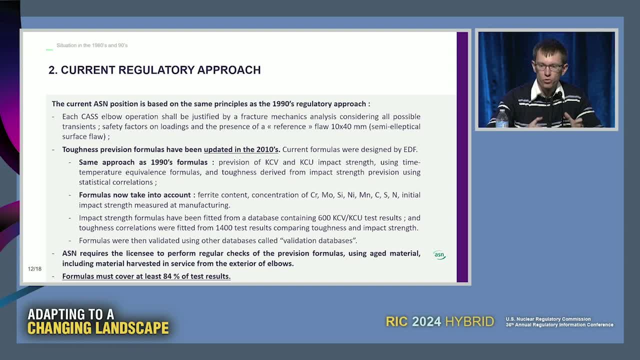 in fact to try to revise those toughness provision formulas, to update them, taking into account those extended timeframes for operation. So they conducted some tests on more than about 600 materials. I mean samples of materials that were either harvested from some elbows that were in operation. 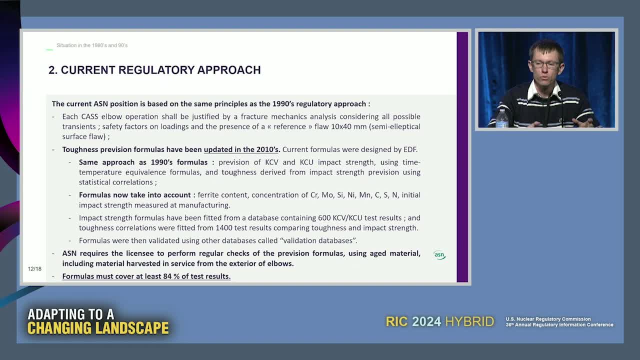 or also some. they used also some material from the manufacturer that was aged in the lab, And so, with this bigger database, they updated the formulas taking into account the number of materials that were used in the lab, And so they did some tests on more than 600 materials. 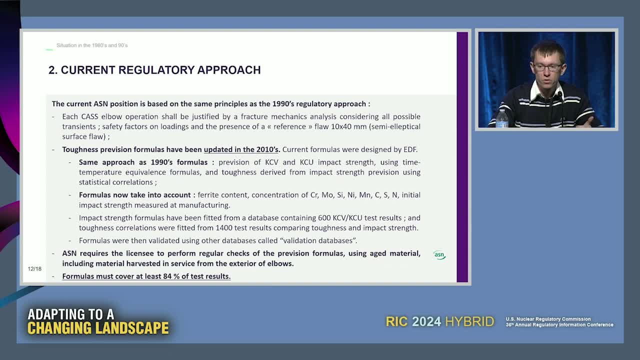 And so they did some tests on more than 600 materials. And so they did some tests on more than 600 materials. a lot of input parameters, one being ferrite content, because the ferrite content in the steel is impacting a lot the final toughness. 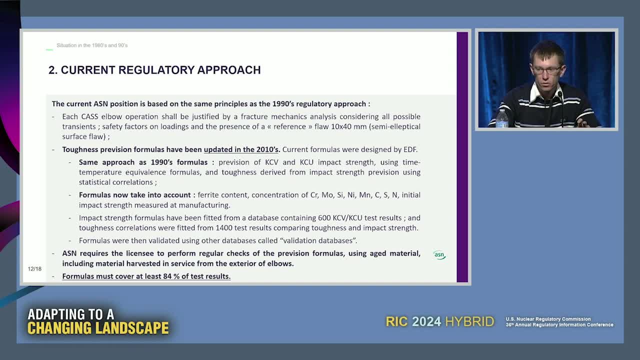 but also the concentration of many chemical materials that was available from the manufacturer, And so currently we have formulas that take into account all this manufacturing data and that is at least supposed to predict the fracture toughness with a coverage of more than 80% of the test results. 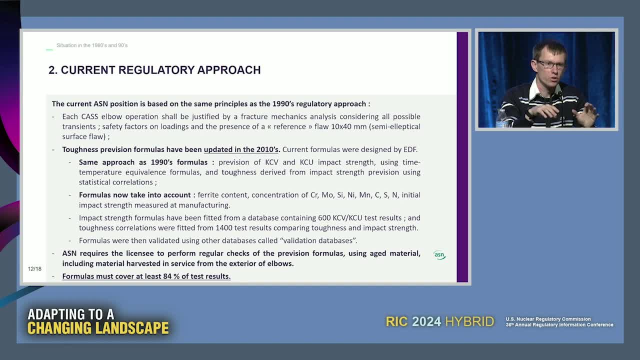 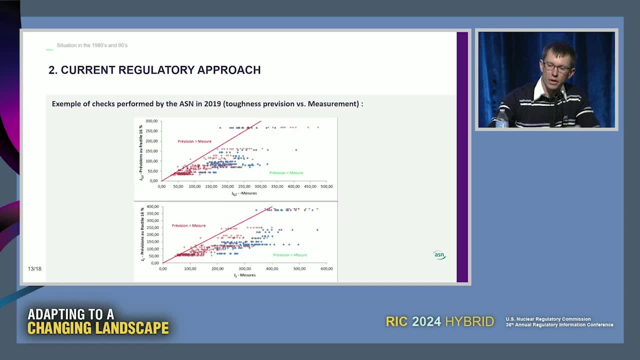 This value of 80% of the test results of 84% being the result of the statistical approach we use in our fracture mechanics computations. So at that time ASN did its own assessment using the test material that was provided by EDF, comparing it to the results of those formulas to check that, in fact, 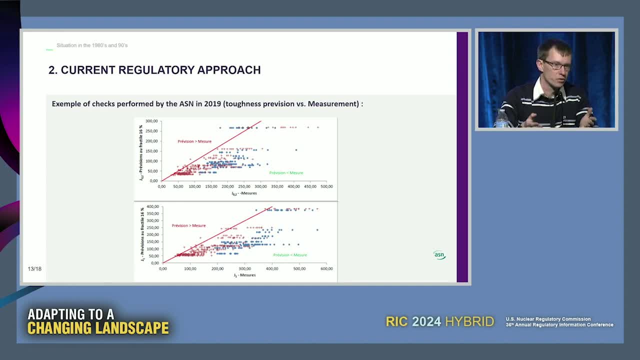 we were indeed covering more than 84% of the results, So the results were quite satisfactory. The database was also covering some samples that were aged up to 200,000 hours, which was enough to cover up to 60 years of operation, And so with that there were some new fracture. 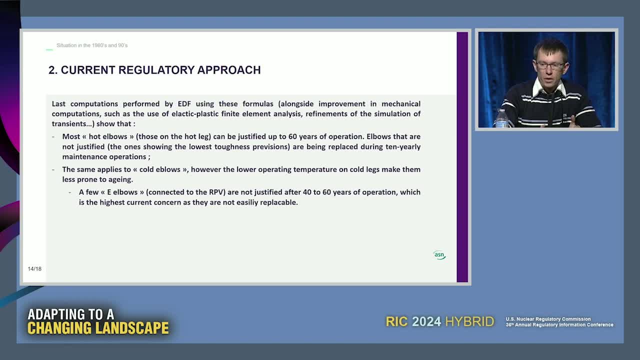 mechanics computations, Thank you. And there were some other computations that were performed and that showed that most of the elbows that are on the hot leg, that are the ones that are subject to the highest temperature, could be operated up to 60 years of operation. And the same demonstrations were done on the 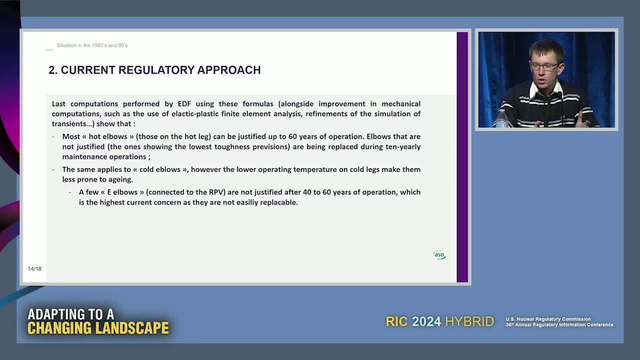 other elbows that are exposed to colder temperatures, And most of them were also justified. The highest content could not pass those fracture mechanic tests and therefore should be replaced before this 60 years time frame. This is the highest current concern for the ASN because 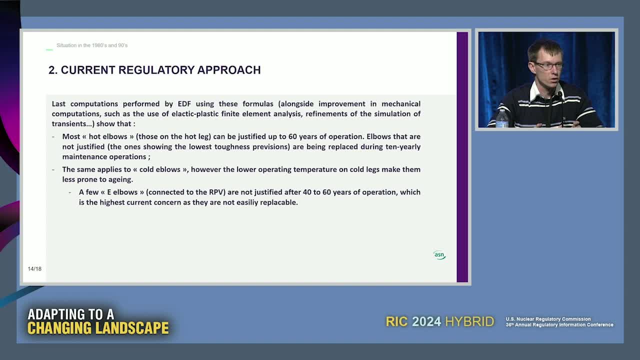 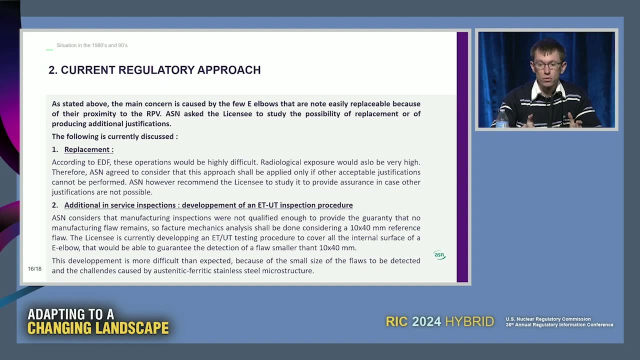 some of these elbows are not easy to replace, especially the ones that are directly welded to the RPV, due to high-dose constraints, And so our current perspectives on that is first to study the opportunity to replace some of these elbows. It is kind of easy. I mean, it's never easy, but kind of easy. 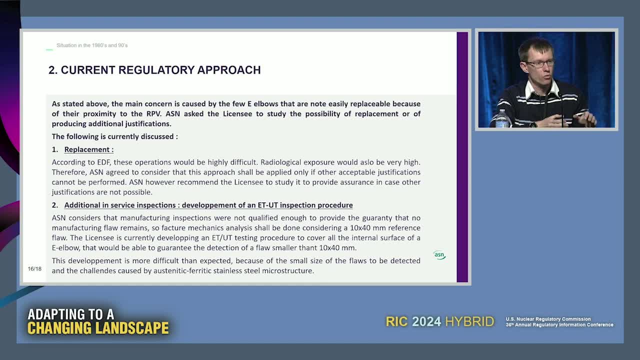 to do for some of them that are not close to the RPV. It's way more complicated to do on the other case. So that's something EDF- and we agree on that- doesn't really want to do. So the other perspective is to improve. The other perspective is to improve the work. 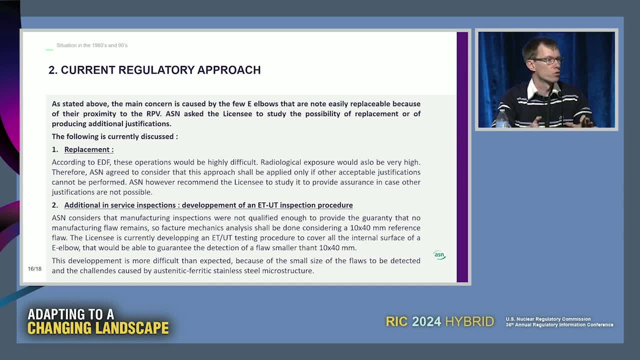 that we do as a company is to improve the way we inspect those elbows to make sure that there are no flaws that would threaten their structural integrity. Even though the toughness is low, if you don't have big flaws, the issue is not as high, The problem being that it's 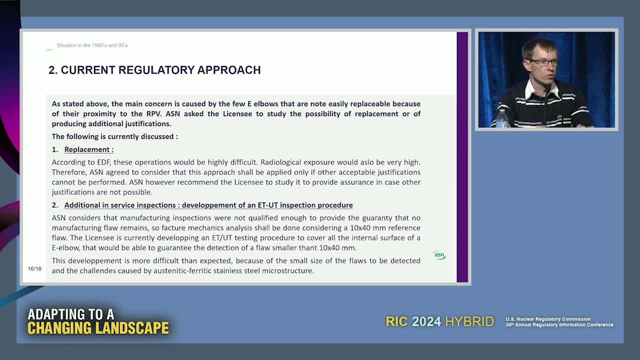 not easy to inspect cast stainless steel because of the structure. For example, UTE waves penetration is not very good, So there is currently some research to try to develop a way of inspecting the steel And think about the challenge In terms of the technical aspects of the GP和i. 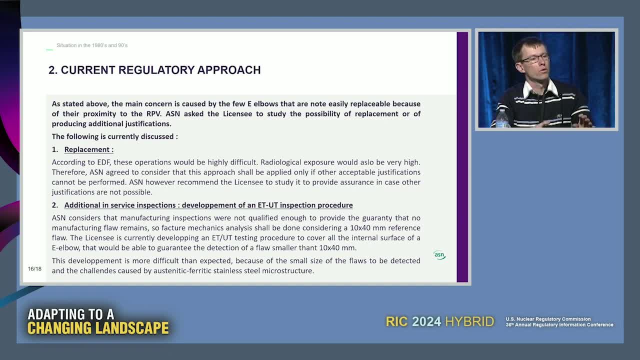 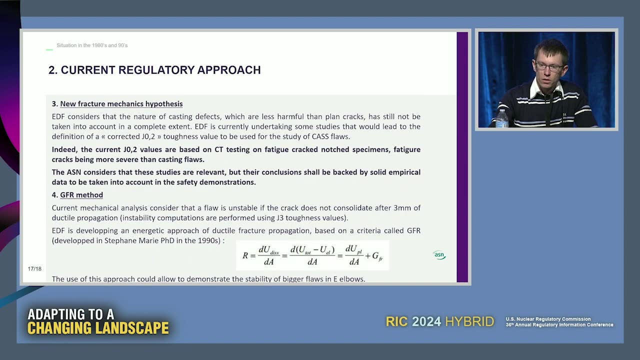 some process, that would at least be good to inspect the first 10 to maybe 20 millimeters from the inner wall, because that is the part that is subject to the highest stresses, for example during a low-key accident, And other perspectives being being reviewed at the moment by EDF and the ISN are using some new 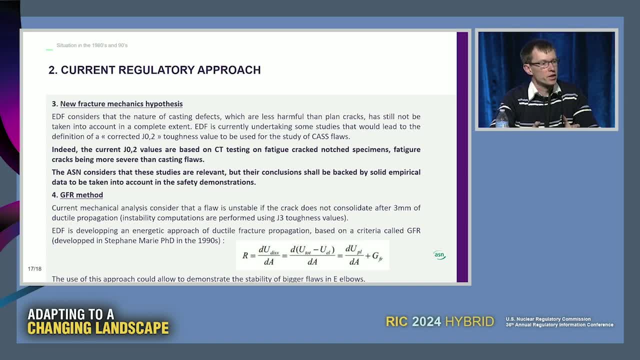 fracture mechanics, hypotheses that would be less conservative, that would take into account in a more precise way the constraints that are generated by those flows and indeed, at the moment, we are only using some toughness values that are determined on some standard test samples that are in fact assessing the 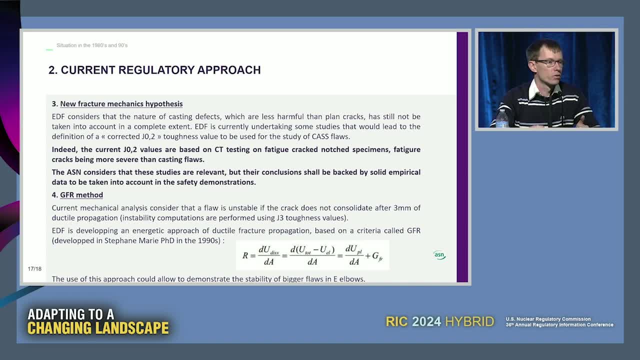 toughness. when you have a crack, We know that you have a crack. when you have a crack, We know that you have a crack. when you have a crack, We know that the type of flows that we have on cast stainless steel are not as harmful as 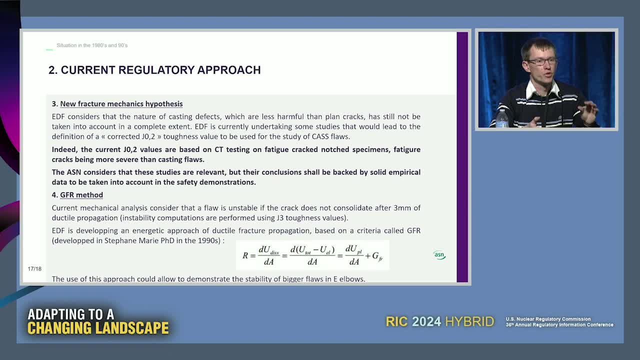 cracks, but it's very difficult to know what is the precise difference and how to quantify it. So this is some ongoing research. At the moment, ISN still ask for some conservative fracture mechanics assessments. This is one perspective also. So just to say that this in order to wrap this up, this is 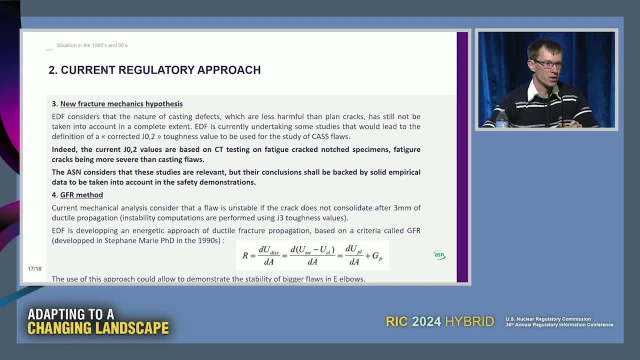 not a new degradation issue that we are facing. In fact, we were already aware of it since the 1980s. But the longer you operate the plants and the more difficult it is to justify that you still have some margins in the case of a. 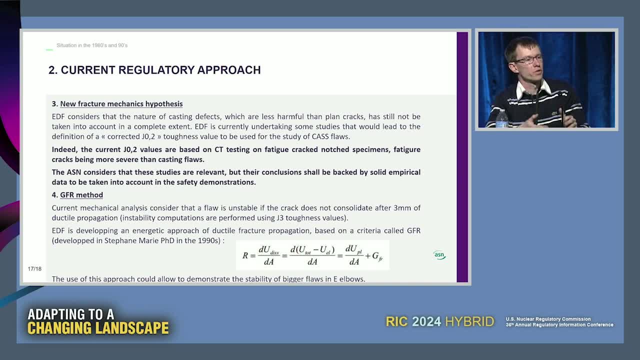 degradation that is slowly decreasing the toughness of your materials. So the longer we operate and the more precise the justification or methods have to be. And this is the goal of ISN is to make sure that even if you go to the plant and get into more precise physical models, fracture, mechanic methods, you're still 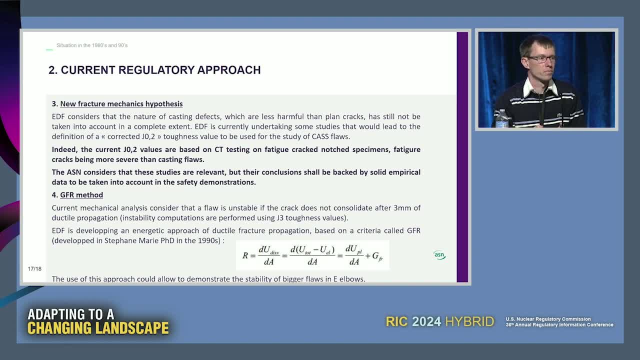 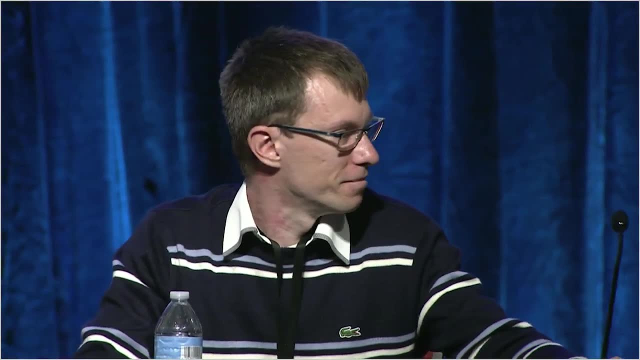 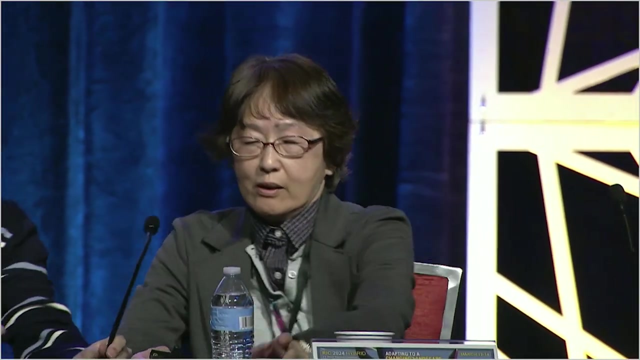 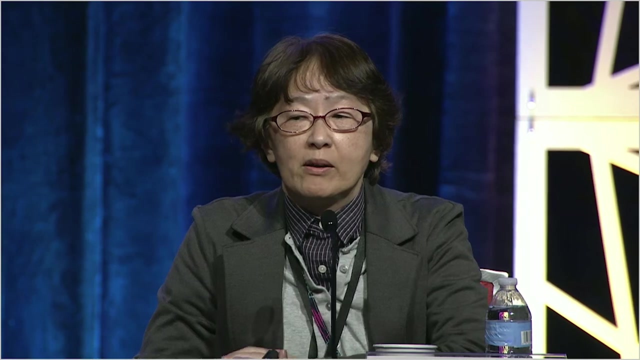 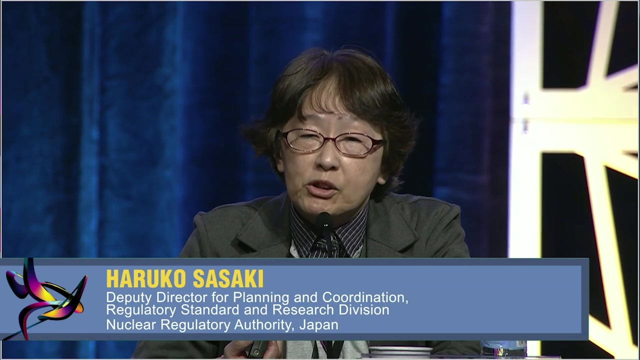 conservative enough in order to maintain a high enough safety. I mean safe enough operating conditions, And I think that's it So. thank you for your attention. Good morning everyone. My talk has two kind of topics. The first one is current regulation revision in Japan And the second one is recent topics related to long-term 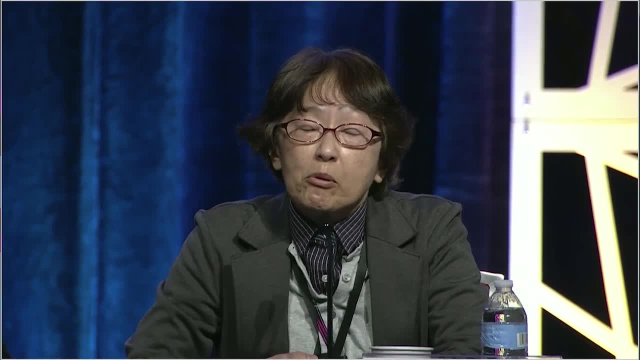 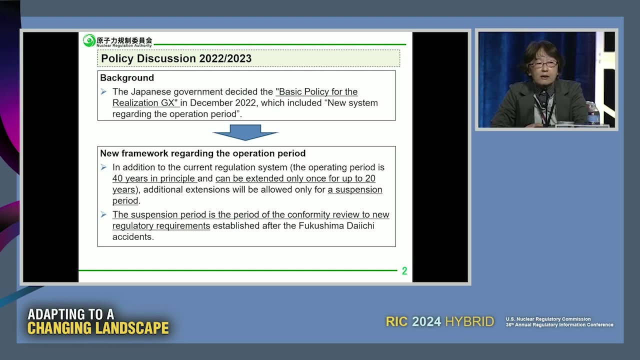 operation. Before Fukushima accident, there is no limitation of operation period. But after Fukushima accident, there is no limitation of operation period. But after Fukushima accident, Japanese government defined the limitation as 40 years originally and could be added maximum 20 years by another approval. 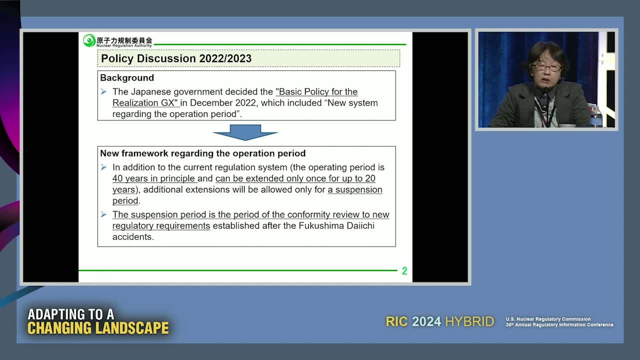 However, 13 years passed from Fukushima accident, Only 12 PWR nuclear plants are operating, and some PWR plant and every BWR plant has been stopped during more than 10 years. So Japanese government made the new policy and the act related to nuclear reactor was revised last year. 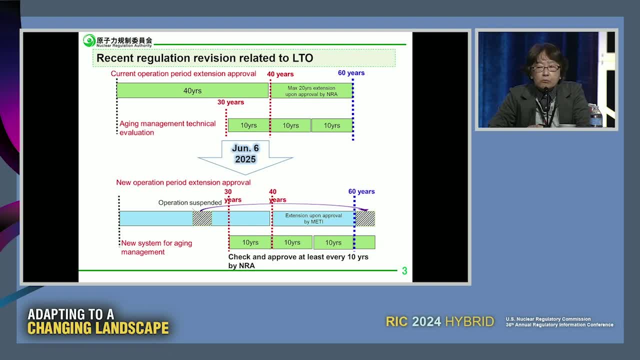 Current regulation period as mentioned before and after 2025, new operation period will be started And the new operation period, operation suspended period, can be added after 60 years. Operation suspended period means the period of conformance review And operation period will be reviewed and approval of the Ministry of Economy, Trade and Industry. 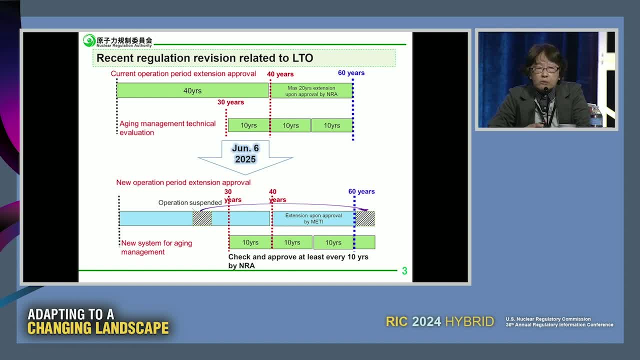 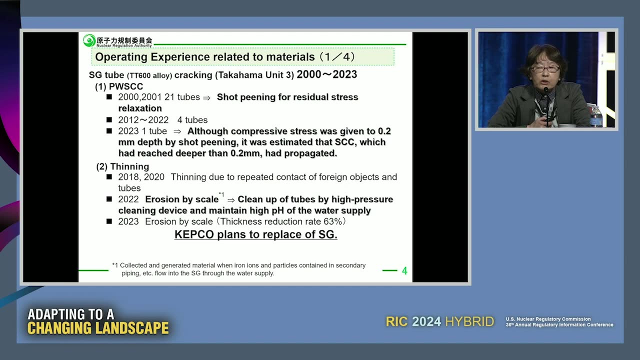 Of course, new system for aging management will be done by NRA, as similar as before. Next is operating experience. First case is NRA. This is steam generator tube cracking at Takahama, Unit 3.. The tube material is TT600 alloy And there are two kind of technical issues. 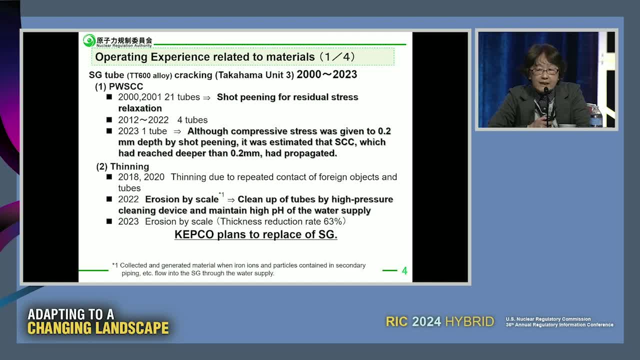 First one is PWSEC. In early 2000, PWSECs were found in 21 tubes And the licensee conducted short peeling for residual stress relaxation. During 10 years there was no indication. it's good, But during our next 10 years PWSECs were found in 4 tubes. 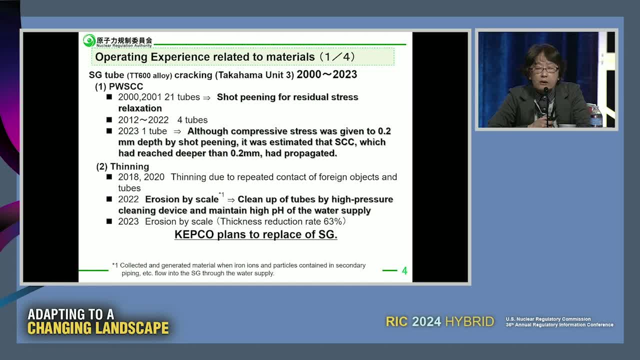 And last year more than one tube Licensees. investigate the cause and estimate that compressive stress was given to 0.2 mm depth in 2020's short peeling, But estimated that SCC, which had reached deeper than 0.2 mm, has propagated. 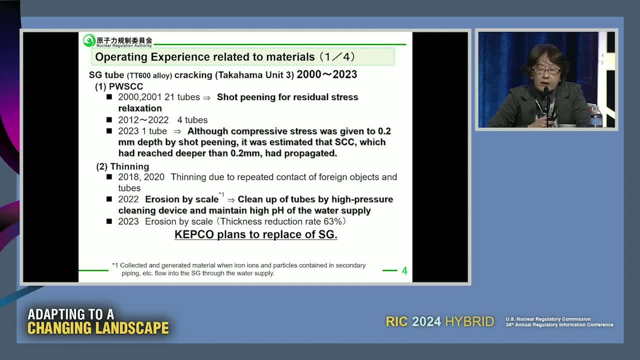 And second issue is thinning. In 2018 and 2020, thinning due to repeated contact of falling object and repeated contact of tube and tube were found, And in 2022, erosion by scale was found. The scale came from water supply. 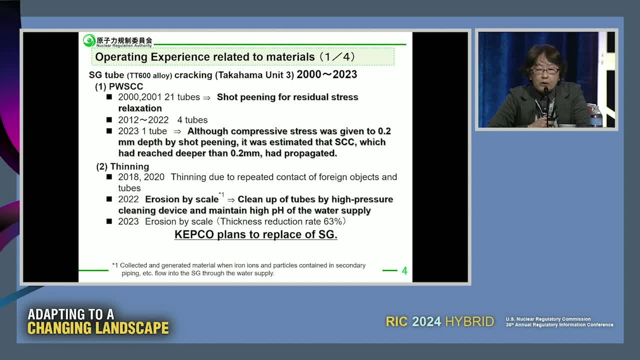 And licensee cleaned up of the tube to reduce the falling material, reduce scale and maintain high pH of the water supply to prevent a new scale. But, however, in 2023, erosion by scale was found again. Currently to replace of the SCC. 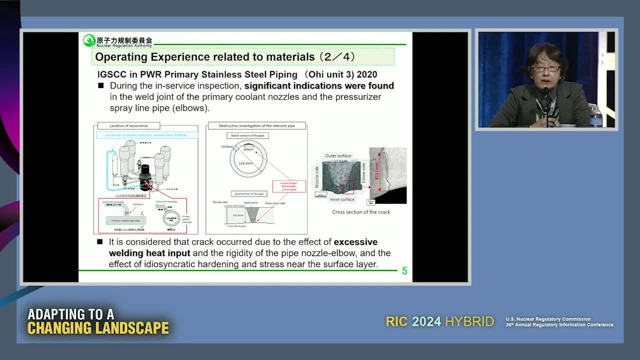 So next one is IGSCC in PWR primary stainless steel piping at OE unit 3.. In 2020, significant indication was found on the surface of the pipe. This is a photograph of the cross-section of the clack. The size was: 3.6 mm depth and 6 mm length. It's very big clack for us and we were very surprised And the licensee investigated the cause and estimated that the cause was excessive welding. heat input and surface of the pipe was hardened and the clack was. 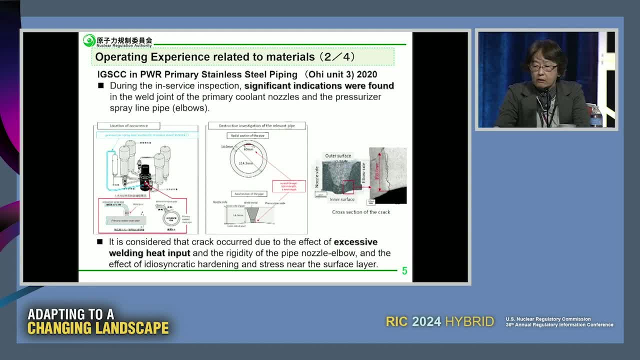 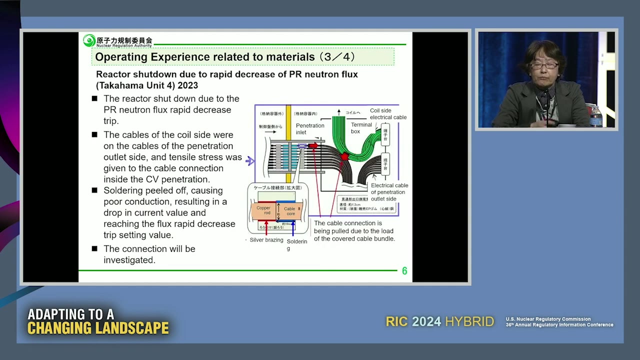 occurred and propagated, Sorry In this case. further investigation is conducting now and we NRA hear from the licensee the result of the investigation every year. Third one is reactor shutdown due to rapid decrease of PR neutron flux At Takahama unit 4.. 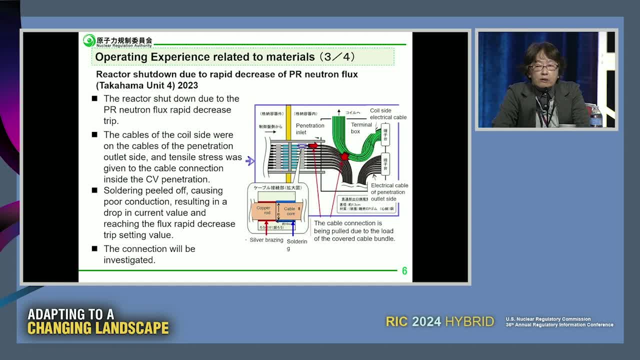 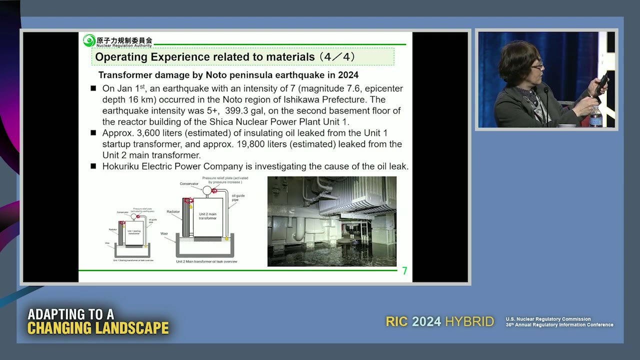 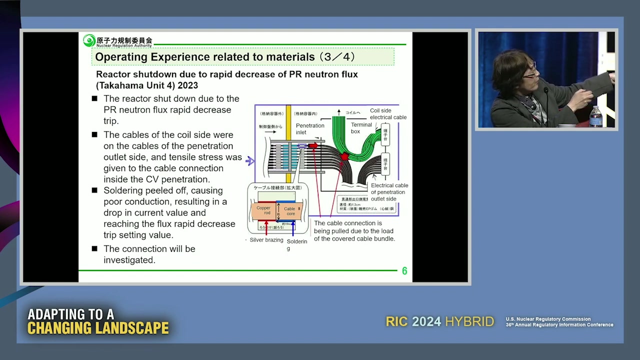 Last year the reactor suddenly shut down and the licensee found that, sorry, connect cables, sorry cables, put on the other cables and cables, ah sorry, cables are pulled and soldering peeled off and the cables disconnected. Of course this case is, ah, non conformance of the construction. 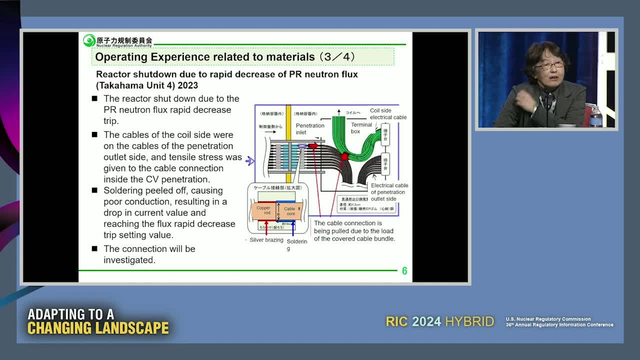 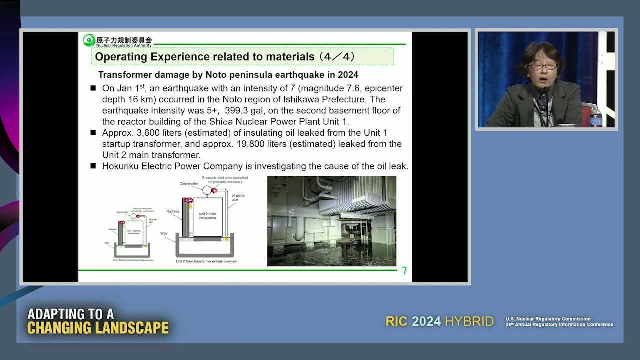 but why now? It takes more than 30 years from construction. so we think there is possibility of the degradation of the material, such as soldering, and the licensee will conduct the investigation of the penetration after replacement. Fourth case is transformer damage by Noto Peninsula earthquake. in 2024.. On July 1st this year, earthquake has occurred. it was magnitude 7.6. And the Seca nuclear power plant is located in the Noto Peninsula And in the plant two transformer was were damaged by the earthquake. 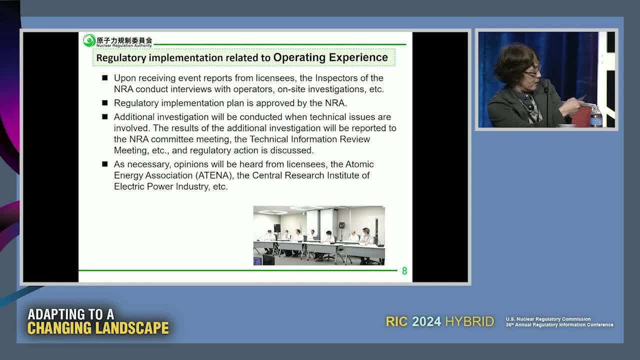 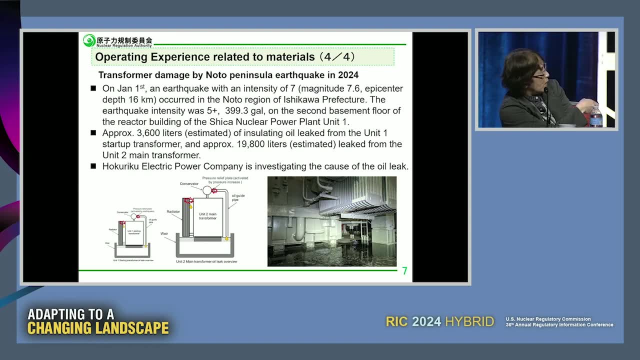 And, ah sorry, Connective pipe was damaged and insulation oil from the transformer. This is a photograph. at the time These transformers were designed as a seismic class C component. according to Japan Electric Association guide, Seismic class C is almost same as commercial grade, but Japan Electric 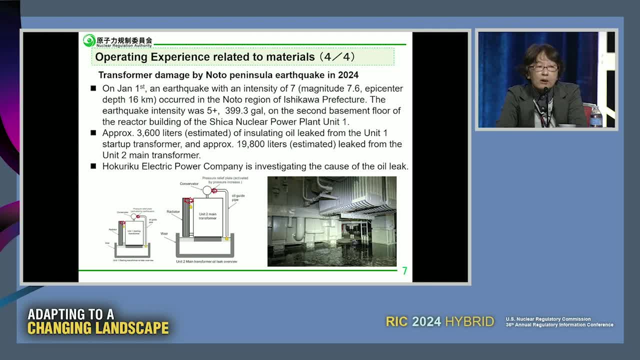 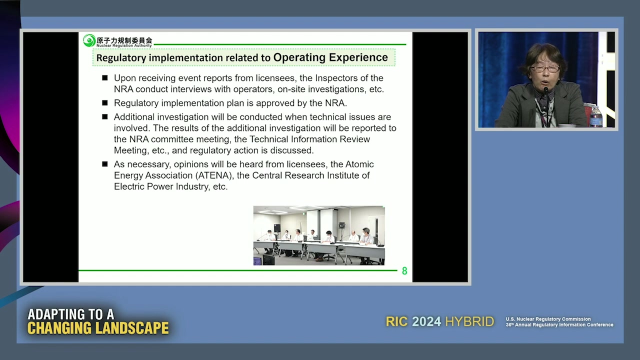 Association calls required to resist the 500 gallon earthquake. There is no measurement device around the transformers, So Hokuriku Electric Power Company is now simulating the earthquake intensity to investigate the cause of the oil leak. The NRA committee: experience is reported to the NRA. 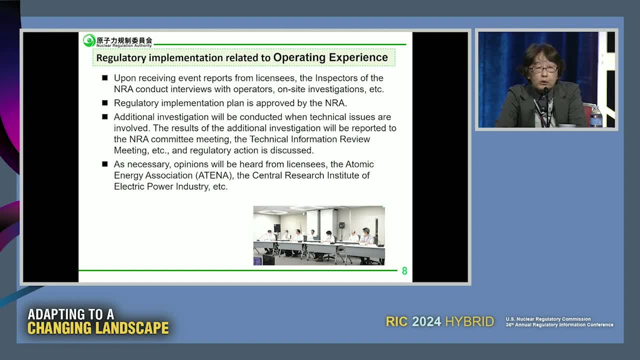 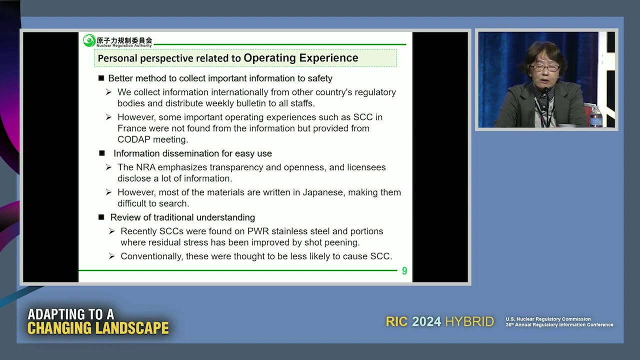 committee meeting. It is held once a week and the regulatory implementation plan is approved by NRA. Sometimes further investigation is required. Regulatory NRA committee meeting or sometimes reported to technical information review meeting and regulatory action is discussed. This is final page of my presentation and 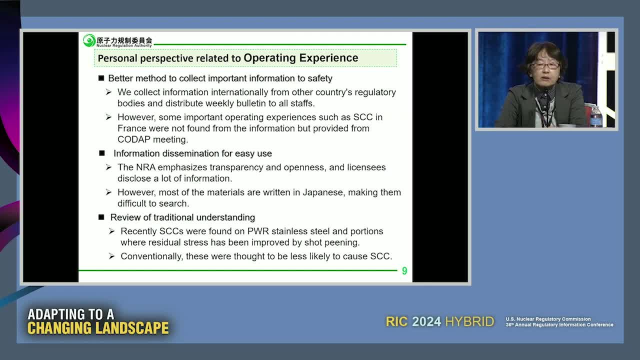 this is my thought and maybe question. We collect important information. We collect information internationally from the other countries, regulatory body and international organization, but some important operating experience were not found from the information but provided from international working group such as CODAP. Our collecting information method is: 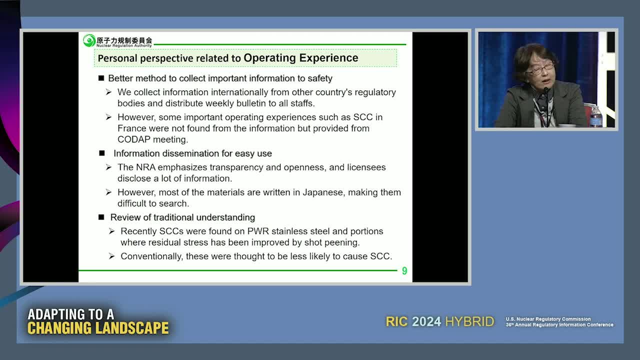 not adequate. In fact, I myself is a member of the collecting information team, so maybe my fault. And the second is related to language barrier. The NRA emphasizes transparency and openness and licensee disclose a lot of information, including data, photograph, figures, But most of the materials 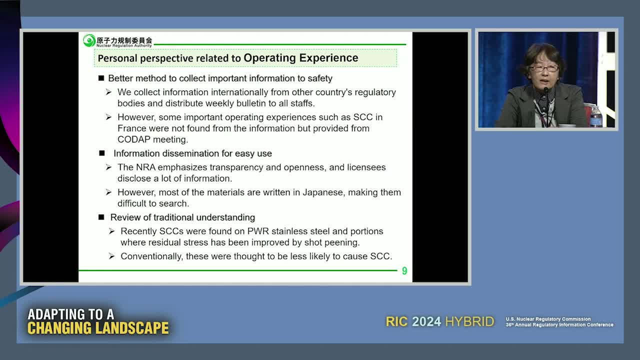 are written in Japanese and it is difficult to provide to the other countries. Third one is related to traditional understanding. Recent topics shows us that sometime it is necessary to reconsider the traditional understanding. So this conference is very good opportunity for me to share our experience. 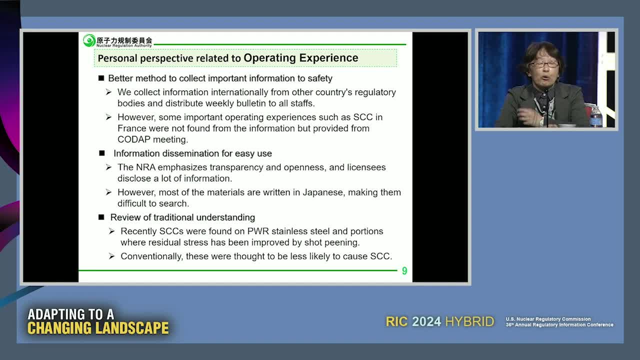 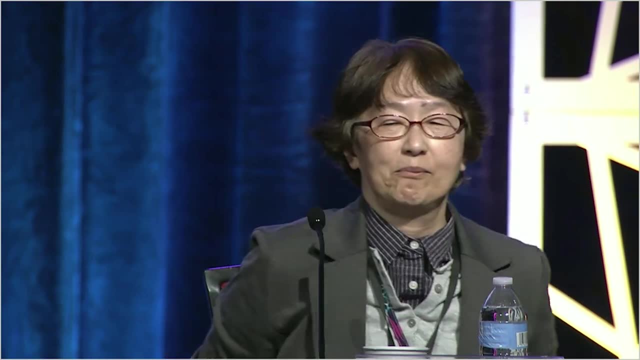 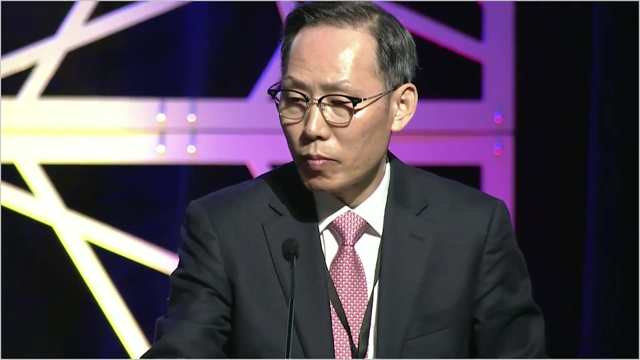 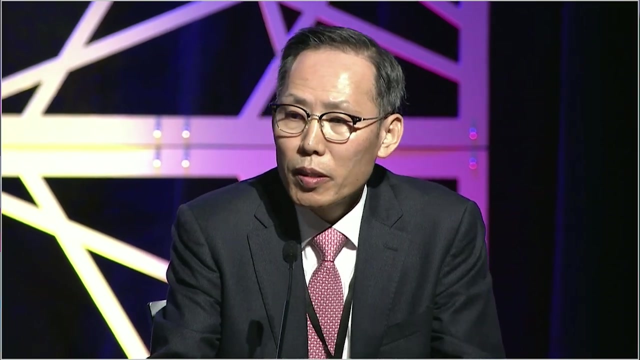 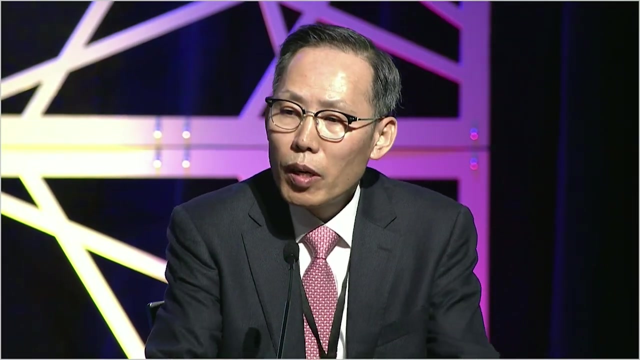 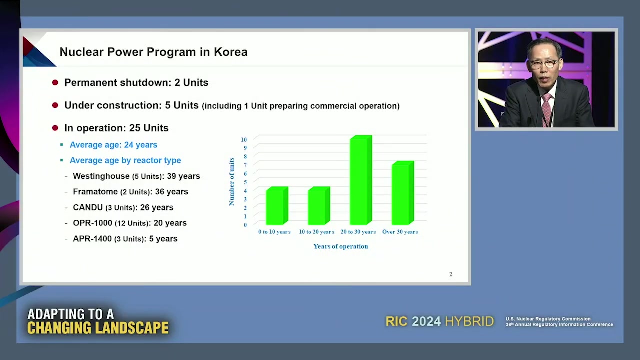 and I hope you provide me good idea or good thought related to these questions. Thank you so much. I am very pleased to share current experience on aging degradation in Korea with you. As of March 2024, two nuclear power plants were permanently shut down. 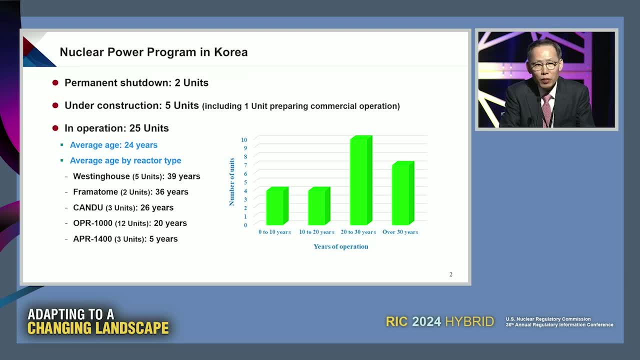 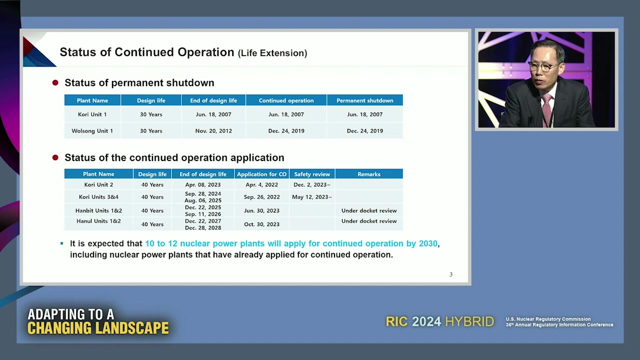 in Korea and five units are under construction and 25 units are in operation. The average operating year is 24 years. Seven of them are operating more than 36 years. This indicated that aging management is becoming more and more important in Korea. The upper table. 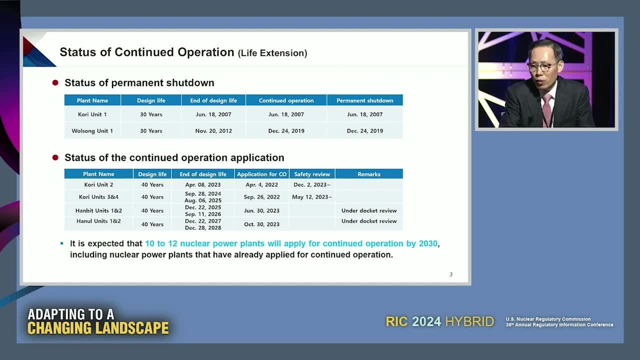 shows the status of permanent shutdown in Korea. Korea Unit 1 was operated for 10 years beyond its design life and Wolsong Unit 1 was operated for less than 10 years beyond its design life. In any case, they were permanently shut down. 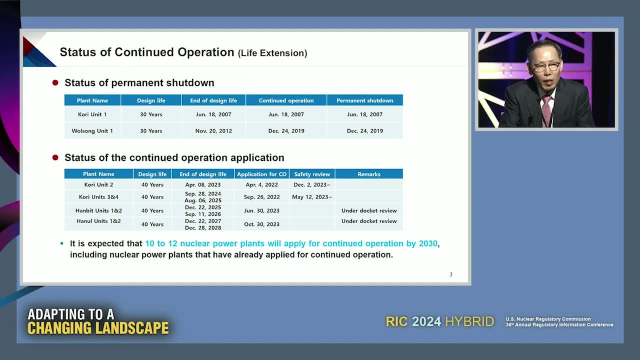 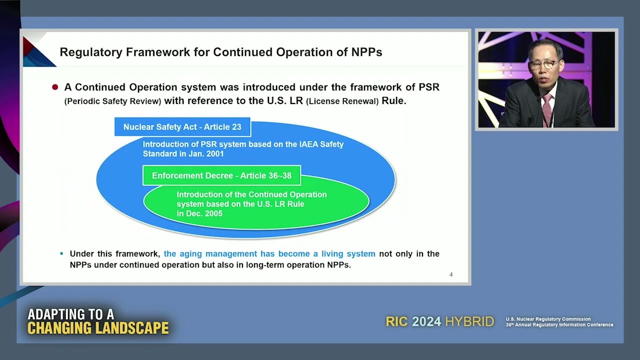 for political reasons, not safety reasons. After changes in energy policy for continued operation, seven nuclear power plants operated for continued operation these days. It is expected that 10 to 12 nuclear power plants will operate for continued operation by 2030.. This slide shows. 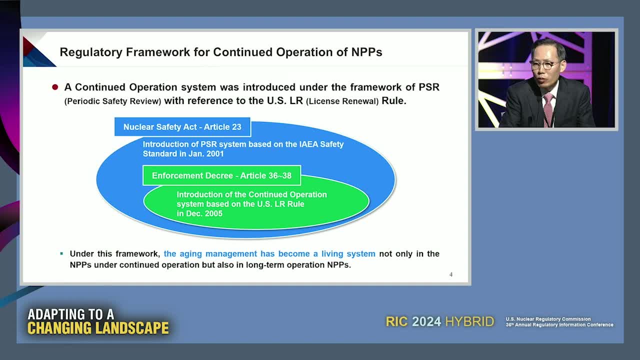 a regulatory framework for continued operation in Korea. The continued operation system was introduced under the framework of PSR periodic safety review with reference to the US license renewal rule. The PSR system and the continued operating system were introduced in 2001 and 2005. 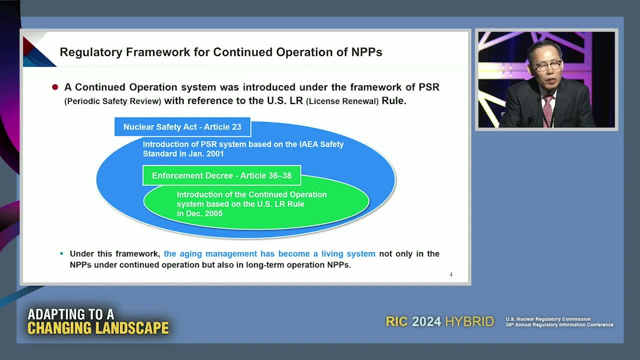 respectively. In PSR system, as you know, the safety assessment should be conducted at regular intervals, typically every 10 years. Under this framework, the aging management had to be implemented during the operation of nuclear power plants, as well as during the continued operation. 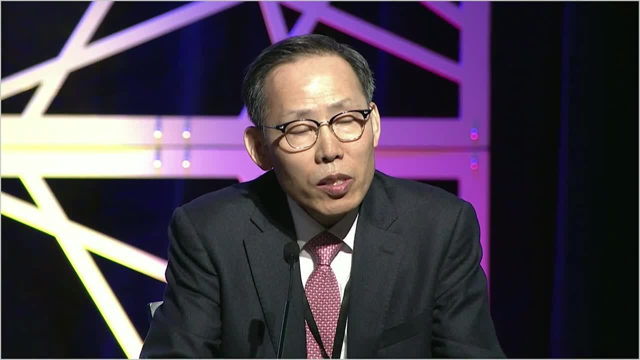 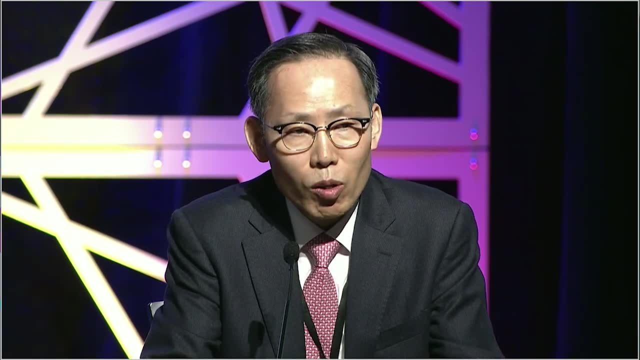 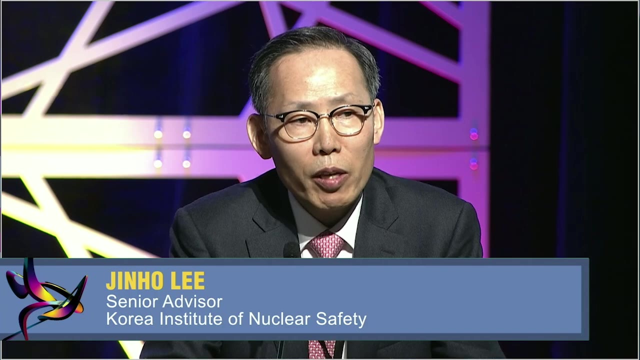 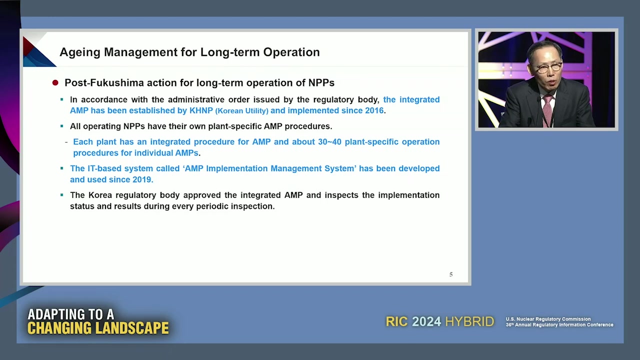 beyond its digital life. In this respect, I think that I can say that the aging management has become a living system in Korea. In order to reflect Fukushima lessons learned from Fukushima accident, the Korea regulatory body issued an administrative order requesting implementation of 50. 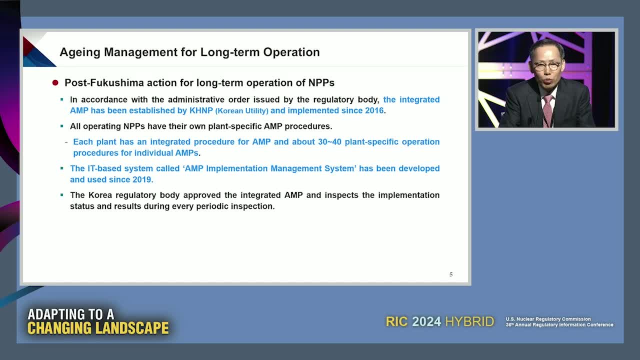 action items. One of the action items is to develop and implement an integrated aging management program. In response to this order, the Korean utility KHMP developed an integrated aging management program Through that each nuclear power plant has one integrated AMP procedure and about: 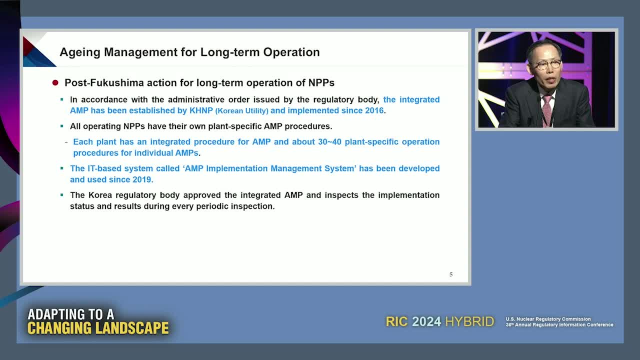 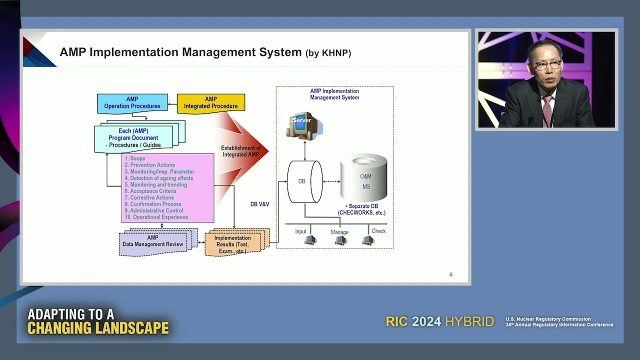 30 to 40 individual AMP procedures. The licensee also developed the IT-based system called AMP implementation management system. The Korea regulatory body approved the integrated AMP and inspects its implementation status and results during every periodic inspection. This slide shows a conceptual diagram of the IT-based 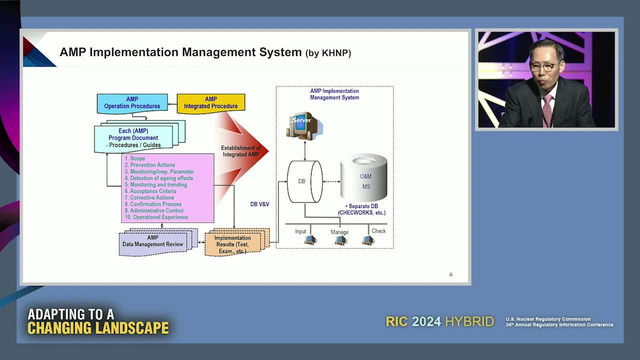 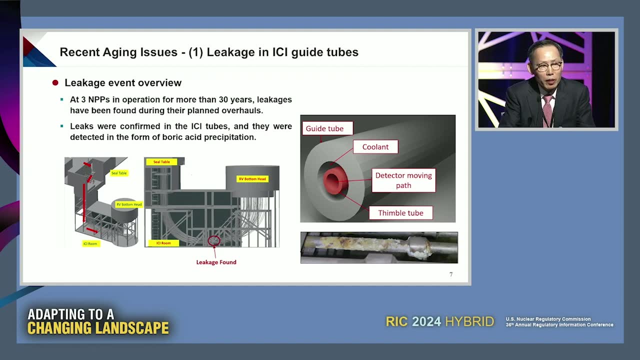 AMP implementation management system. So far, I introduced briefly the Korean regulatory framework for continued operation. Now I'd like to introduce recent aging issues. The first one is the leakage in INCO instrument guide tubes As three nuclear power plants in operation for more than 30 years. 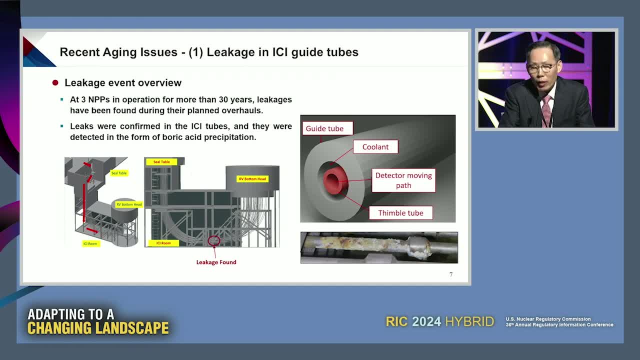 leakages have been found during their planned ovaries. Leaks were confirmed in the ISRI tubes and they were detected in the form of boric acid precipitation. Boric acid deposits were found in one curved section and found in several horizontal joint areas of ISRI. 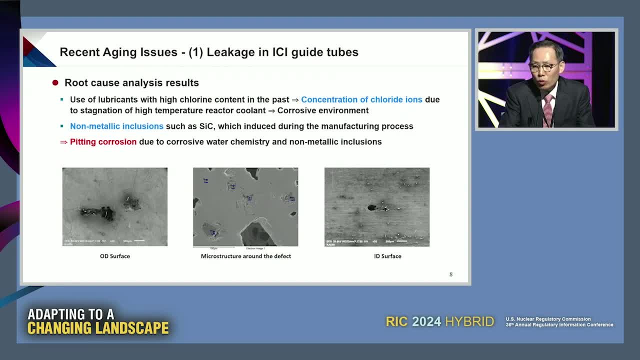 guide tubes. Through root cause analysis, it was found that the high chlorine content lubricant was used during seal table maintenance in the past. The concentration of chlorine ions was intensified due to stagnation of high temperature reactor current, and it is so that this created. 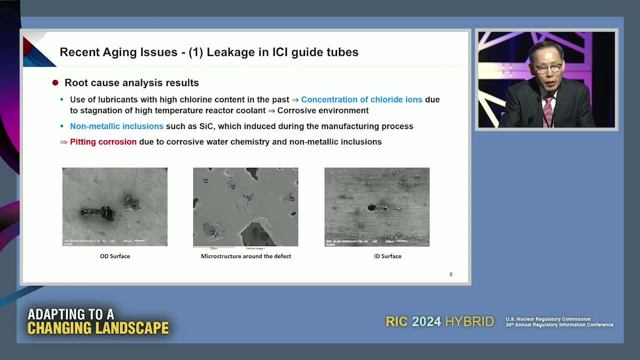 corrosive environment. In addition, microstructure analysis showed non-metallic inclusions such as silicon carbide. It was found that these non metallic inclusions were introduced during the manufacturing process. From this it can be concluded that the root cause of ISRI guide tube. 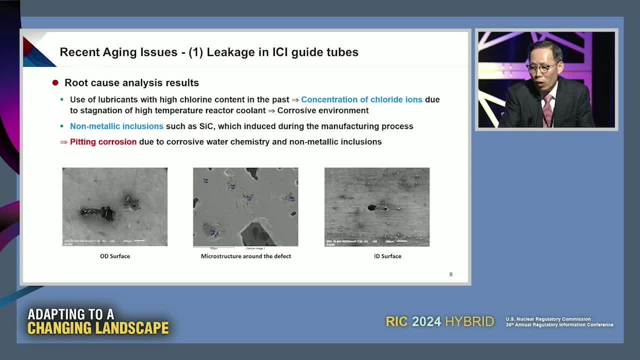 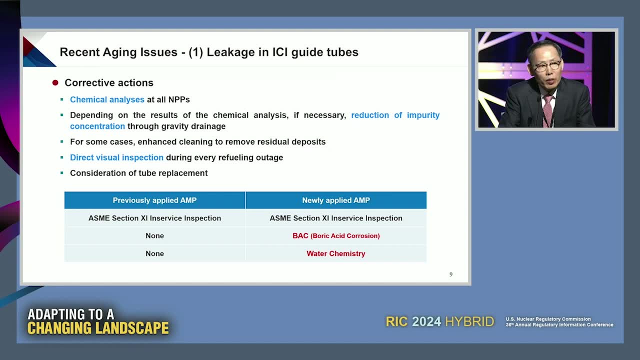 leakage is due to corrosive water chemistry and non-metallic inclusions. There are measures such as chemical analysis at all nuclear power plants and reduction of infiltrate concentration through gravity drainage and direct visual inspection have been taken as corrective actions. In addition, the previous 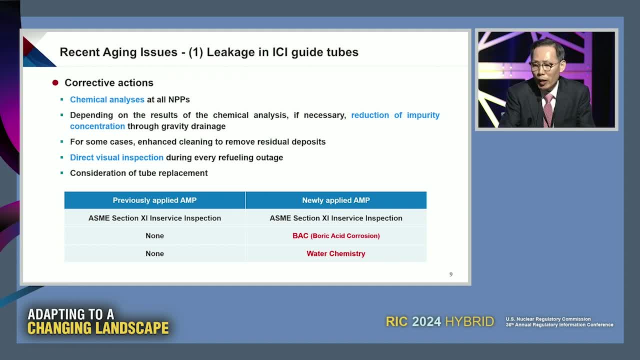 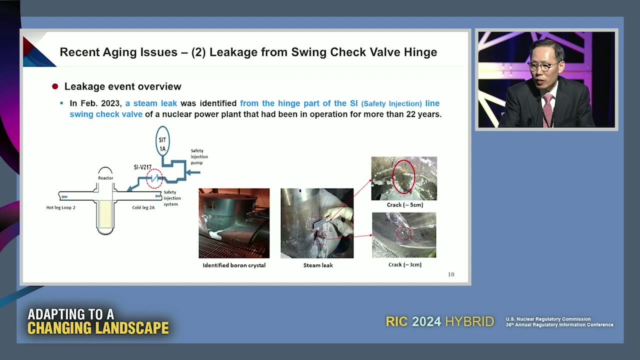 existing AMP was improved by conducting effective BAH boric acid corrosion program and by conducting local water chemistry analysis. The second recent aging issue is leakage from swing check valve hinge. In February 2023, a steam leak was identified from the hinge part of the safety. 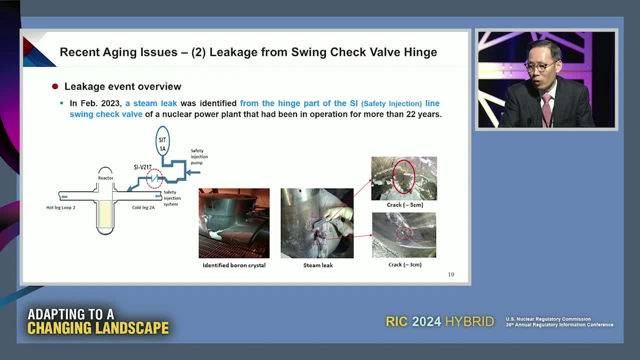 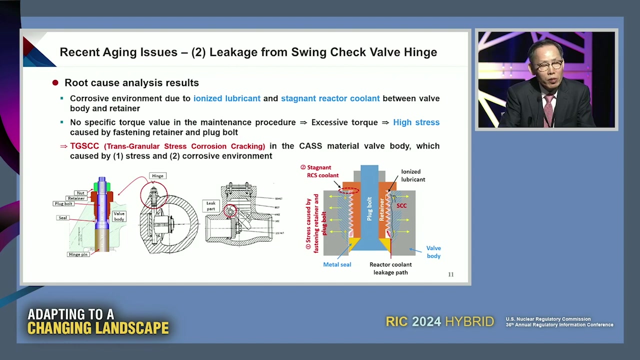 injection line swing check valve of a nuclear power plant that had been in operation. The left picture shows ICS line safety injection line and check valve. Steam leaks and cracks were found in the valve body near hinge. Through root cause analysis it was: 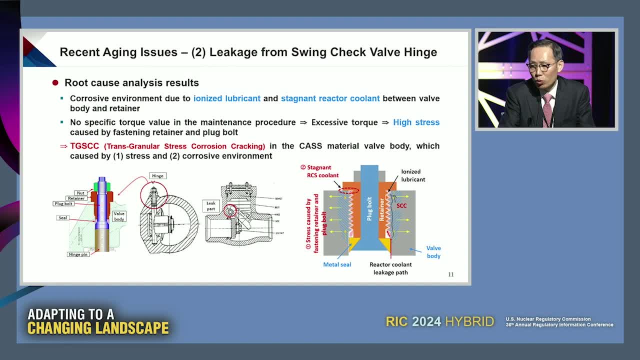 found that corrosive environment was created due to ionized lubricant and stagnant reactor current body and retainer. In addition, it is thought that excessive torque was applied because no specific torque value was not provided in the manufacturing process in the past. It is thought that 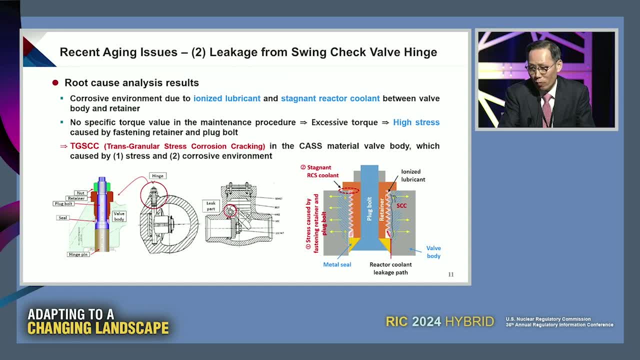 high stress was caused by facing retainer and frog vault with excessive torque. Through this, it was concluded that the root cause of leakage is TGSCC: transgranular stress, corrosion, cracking caused by stress and corrosive environment. The measures, such as visual inspection. 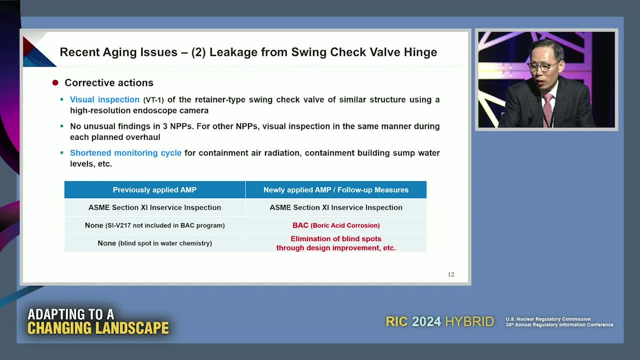 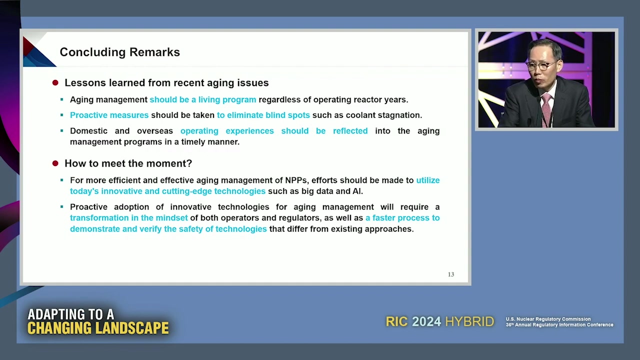 using high resolution endoscope camera and shortened monitoring software have been taken as corrective actions. Also, some improvement of the design to eliminate the blind spot through the design improvement was also taken. As a concluding remarks, I would like to mention lessons learned from today. 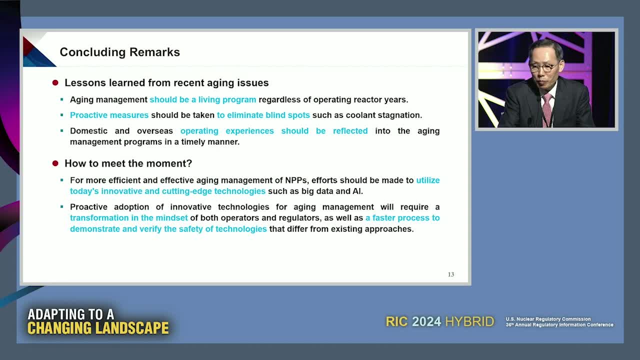 Aging management should be a living program. Projective measures should be taken to eliminate blind spots. Operating experiences should be reflected into the aging management in a timely manner To meet the moment. efforts should be made to improve the quality of the technology, Also the mindset. 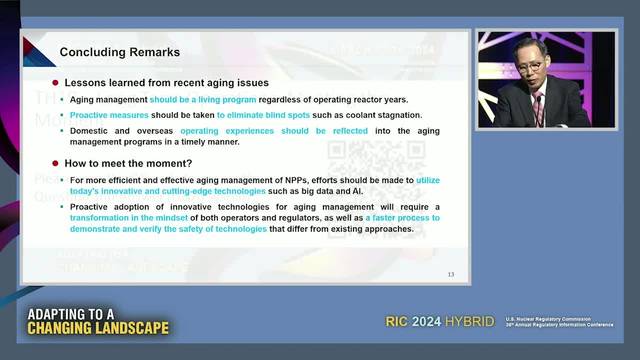 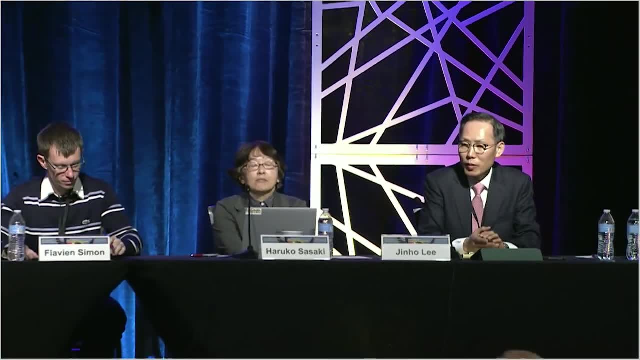 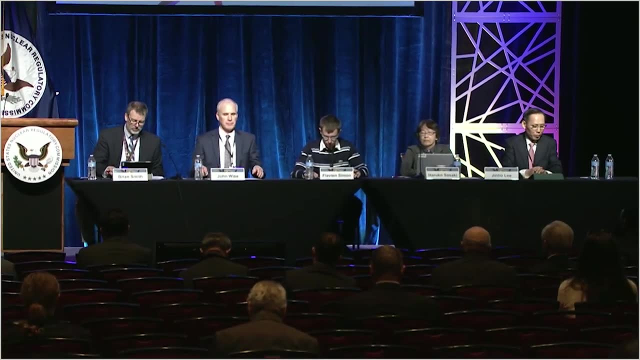 should be changed at the same time. Thank you for your attention. All right, Thank you, panelists, for the nice presentations. I think there's kind of a common theme throughout all of those is that each of the agencies appears to be like learning over time. 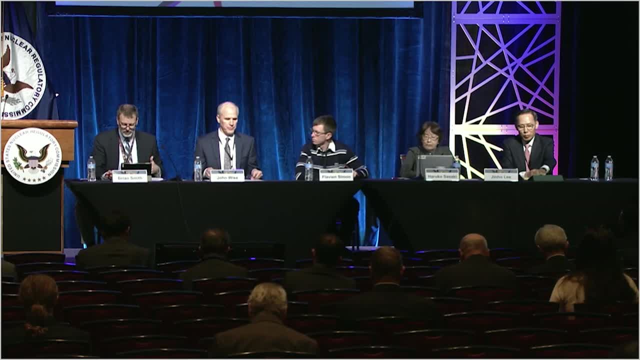 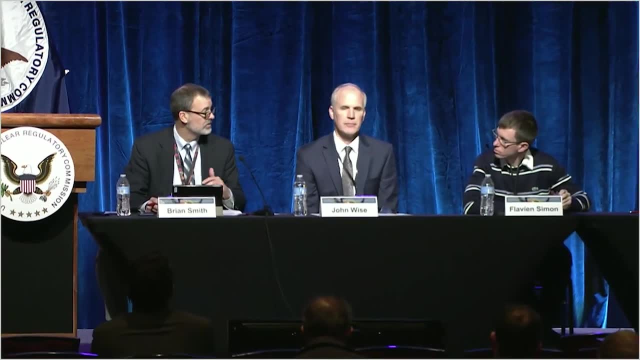 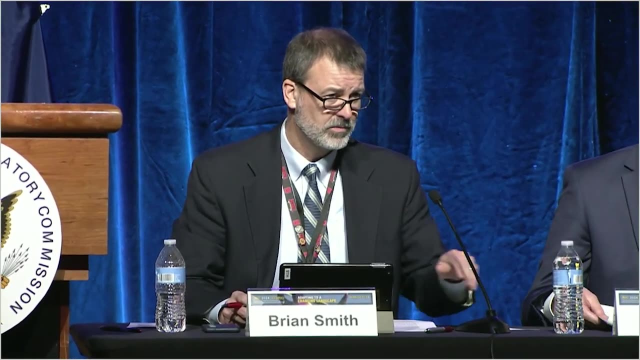 evaluating operational experience and then adjusting their guidance and requirements over time to reflect that what they've learned, as well as working with licensees to address site-specific issues. So, all right, we have plenty of time for Q&A, so please submit your. 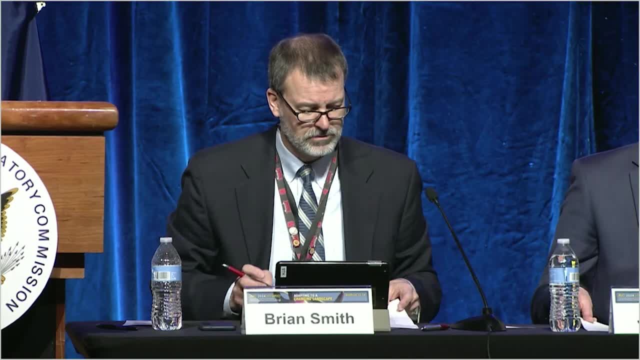 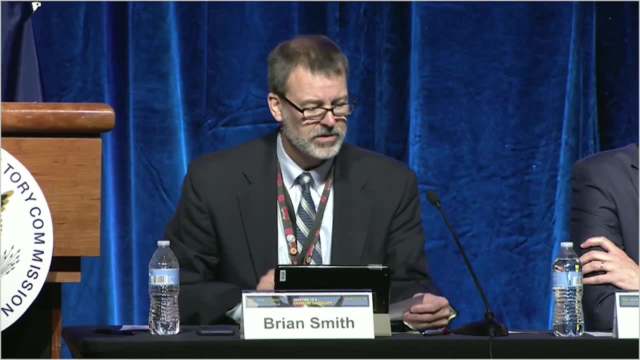 questions. We do have a few pre-written questions here that we want to go through some of those first before we get into some of the audience Q&A. And so the first question which we'll try to ask each of the panelists to address: 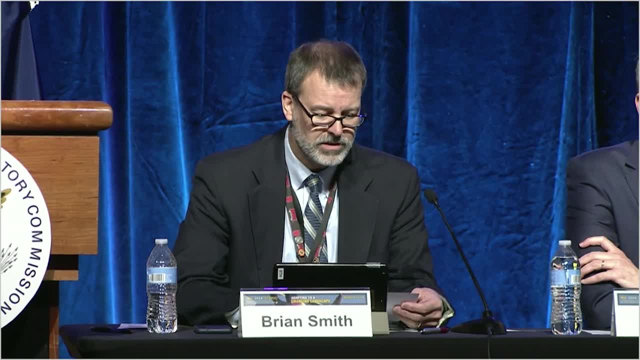 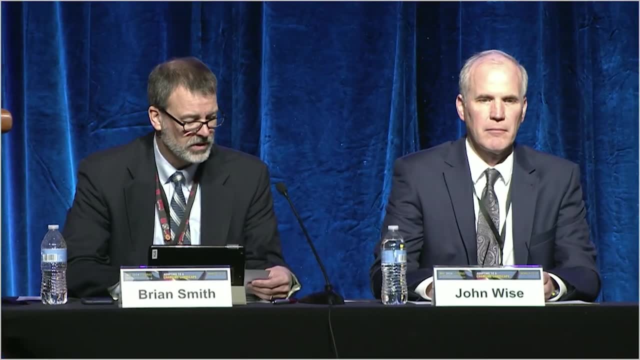 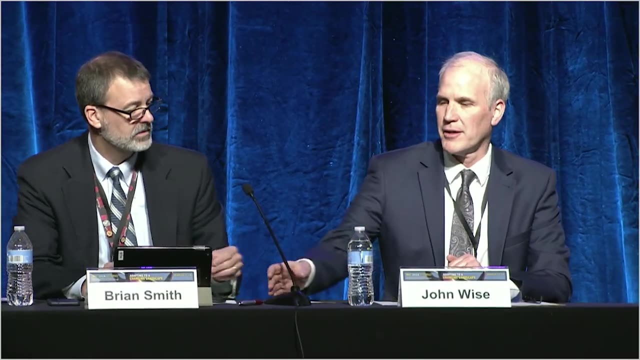 is when a new or unexpected aging issue arises at a plant in your country. what is the role of the regulator in assessing its implications for the entire industry And what is the role of the plant or industry? John, do you want to go first? 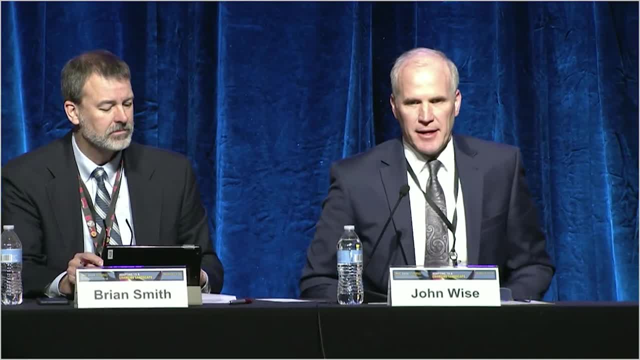 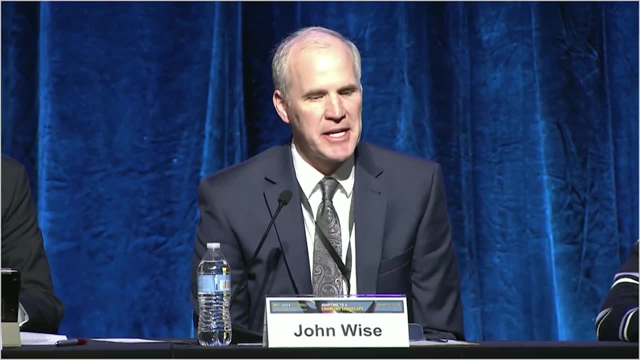 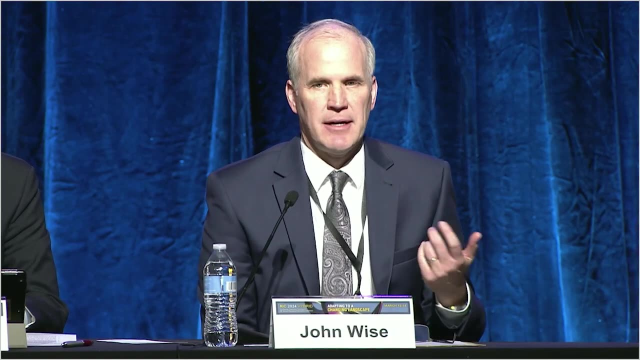 Sure, and I guess I'll be brief because I think I'm going to expand on just some of the same themes as I went through in my presentation. But the NRC has an operating experience program and we have an internal instruction that guides that program. And for those that want, 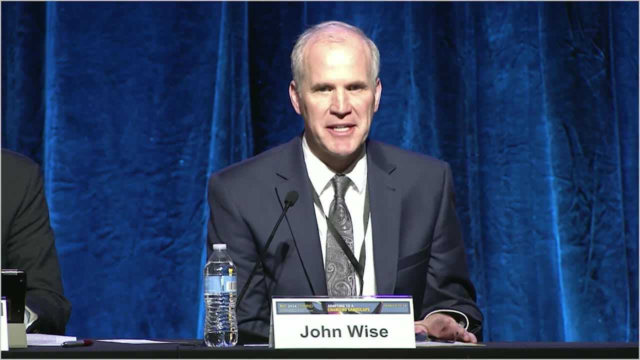 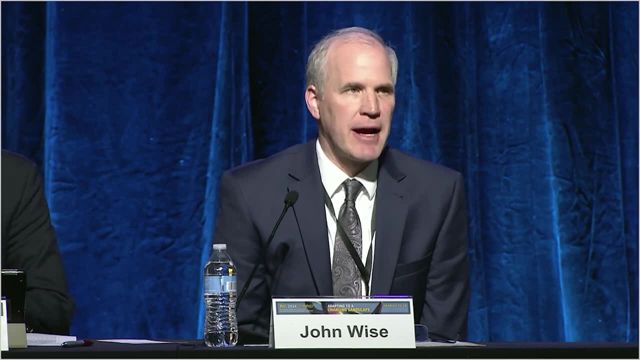 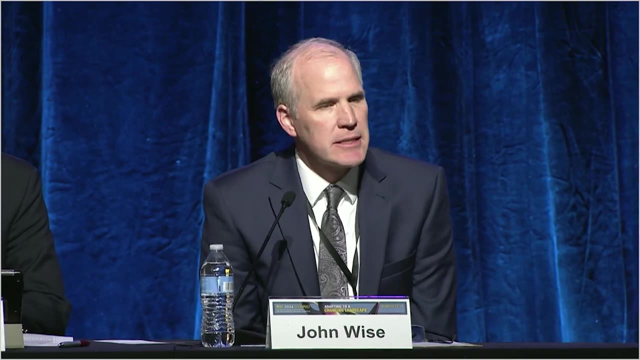 to look it up, it's LIC 401,, I believe LIC 401.. And it's available publicly. And what that program does is it basically describes the process by which the NRC collects, evaluates, screens the safety significance of issues. 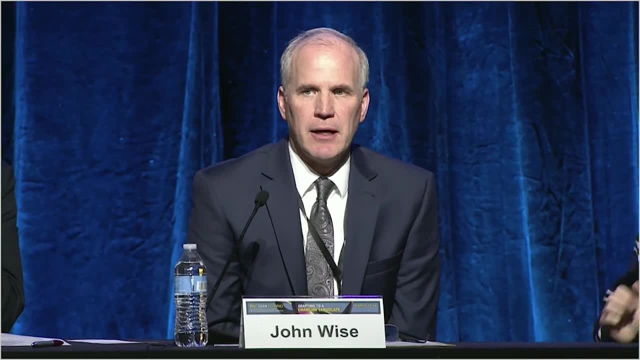 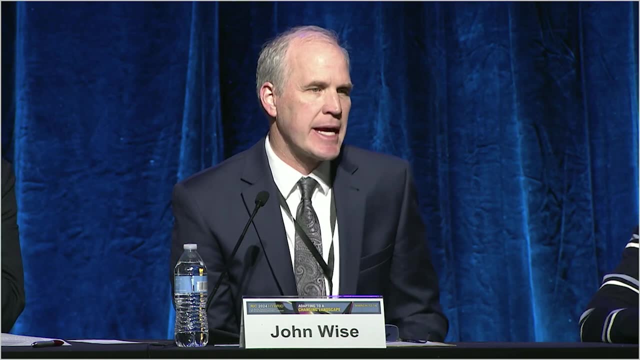 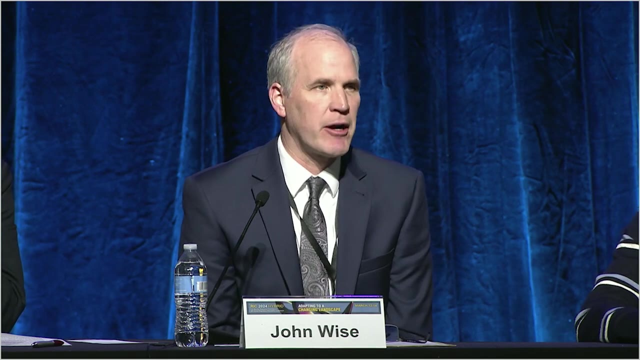 and ultimately identifies actions. And those actions could be anything from, as in the case of my presentation, simply issuing communications to the industry to ensure that they are aware of the issue and they can apply that experience as appropriate at their plant. But the actions could. 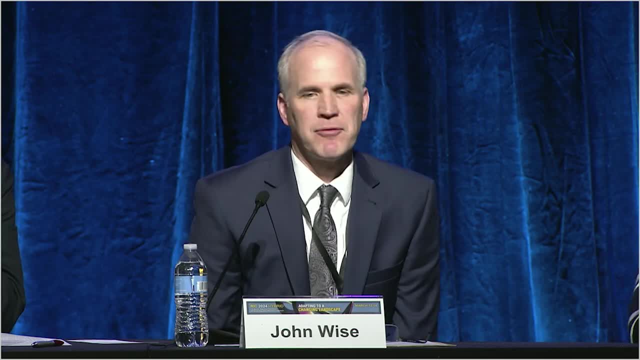 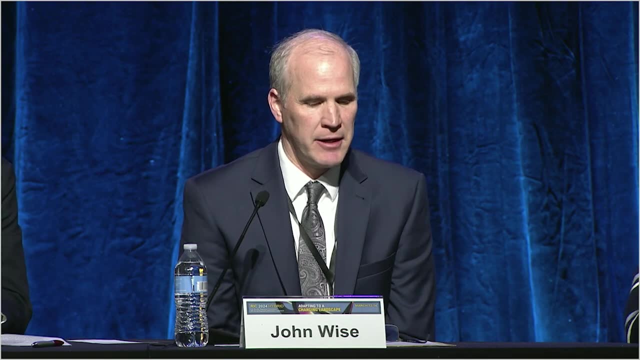 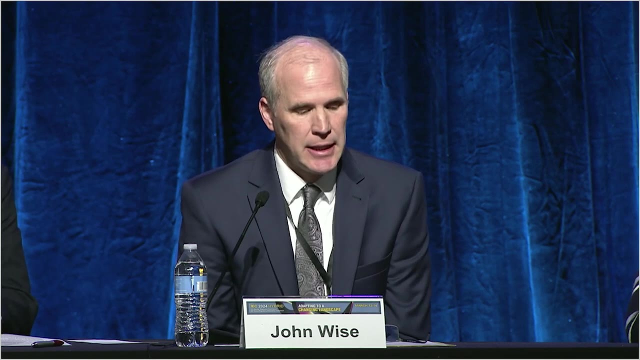 also become something more broadly than that. For example, very time sensitive high safety issues, There could be a regulatory action, something as extreme as, say, an order where there's an expectation the plant take an immediate action, But longer term, the same process. 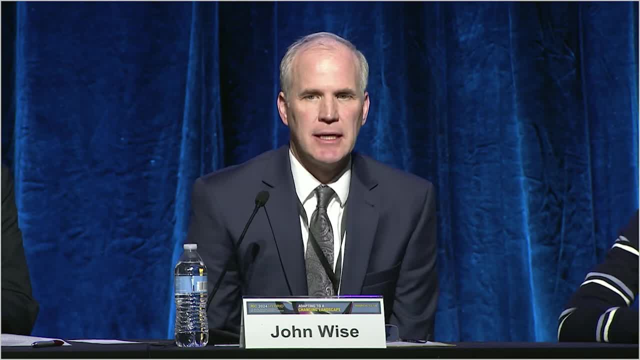 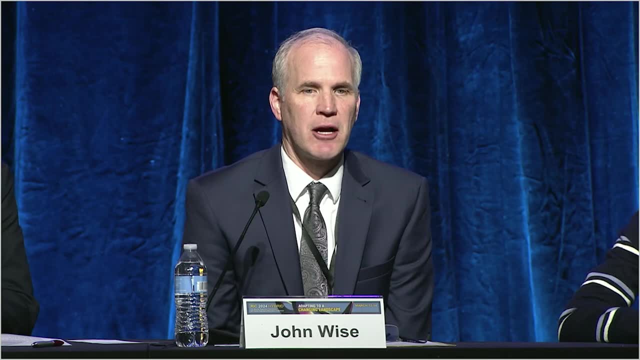 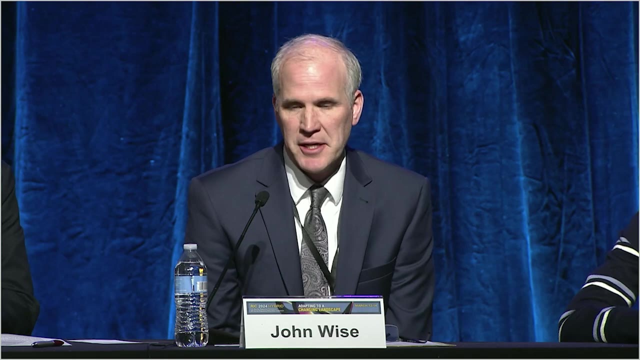 I'm describing our operating experience review process directs us to look at our broader programs. Does that operating experience cause us to revise our should, cause us to revise our guidance, Or is rule change in a rule justified, Or change in our inspection program? 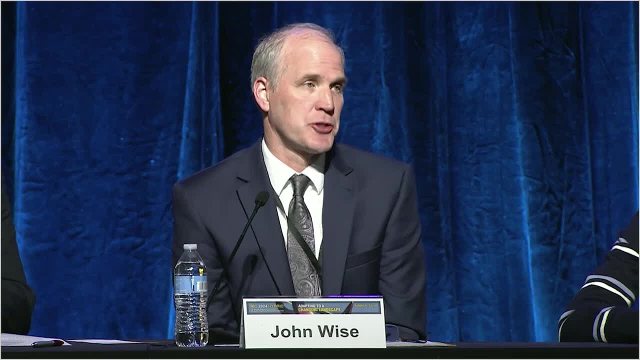 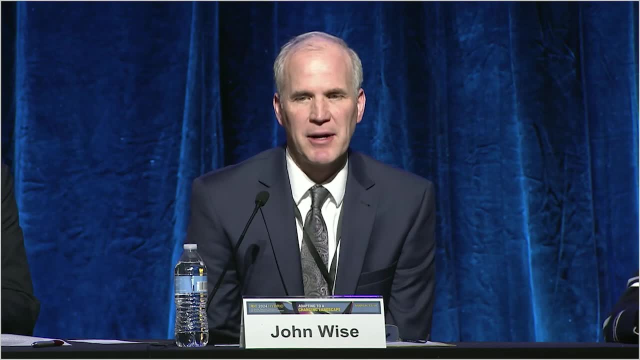 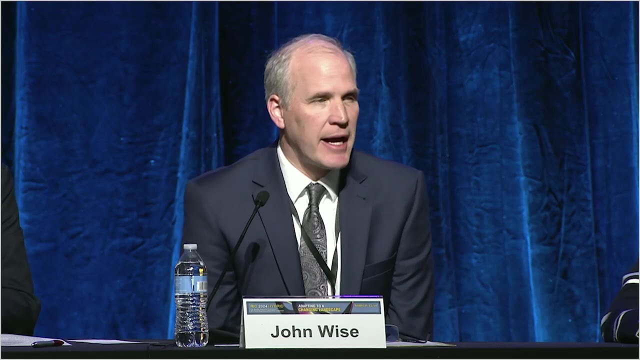 Or even longer term change in our research program. And so by this process, you know again we call it the LIC 401 or LIC 401 process. it kind of guides the staff through all of those steps, But outside the NRC. 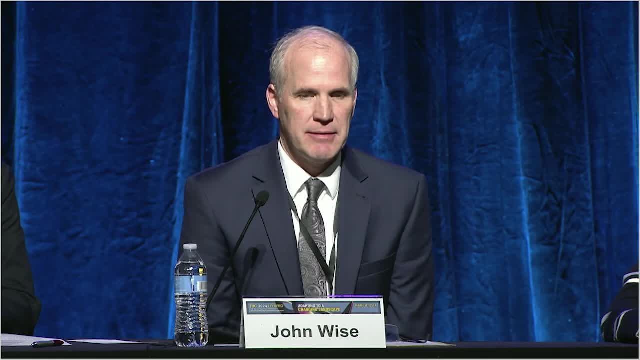 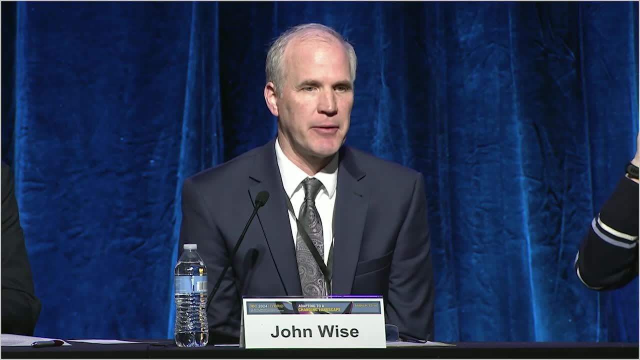 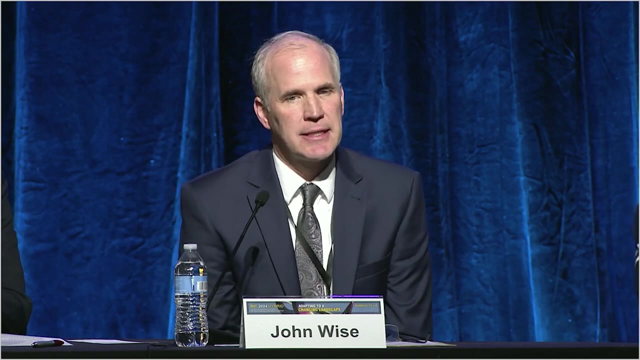 you know we have. there is the plants in some sense do the same thing. right, And the plants have. there is requirements that plants evaluate operating experience. But on their part, when they experience operating experience, the expectation is that they. 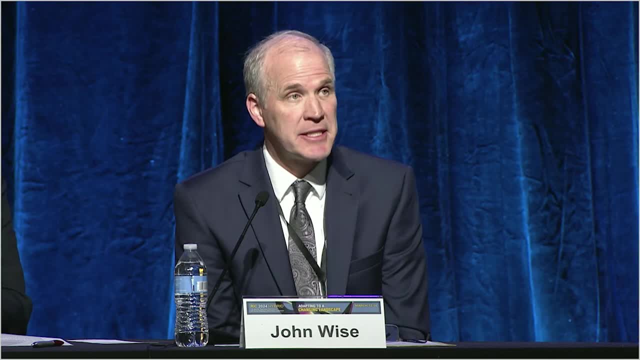 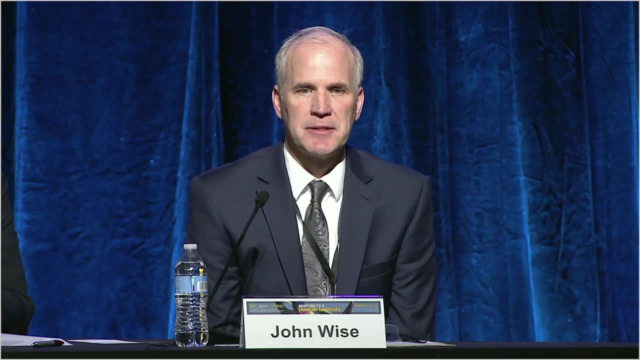 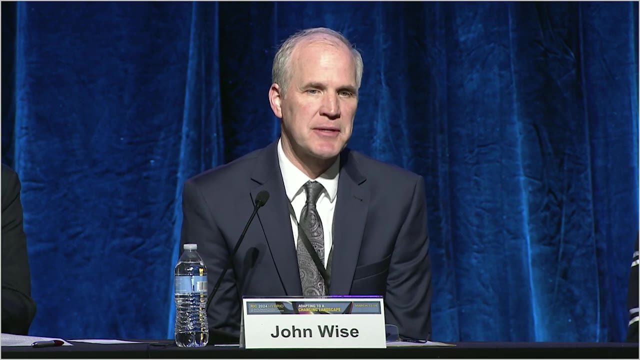 themselves also make that decision whether or not that experience needs to be shared with the broader community. And they do that principally, as most of us know the different programs that are involved, such as the INPO program, to share operating experience outside of your plant as appropriate. 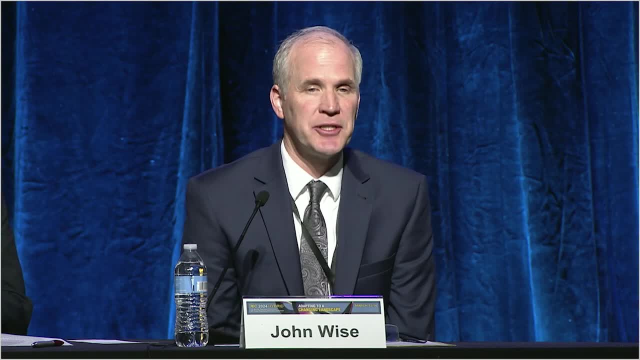 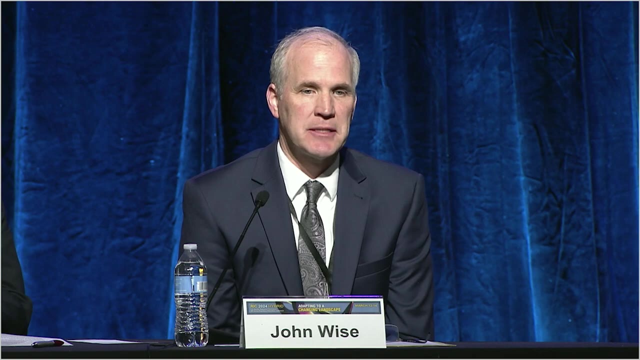 And so, as part of our licensure renewal review, we actually do take a look at that program from the aging management perspective. It directs the staff to look at the applicant's process just to ensure that long term aging issues too, are evaluated and, as appropriate, 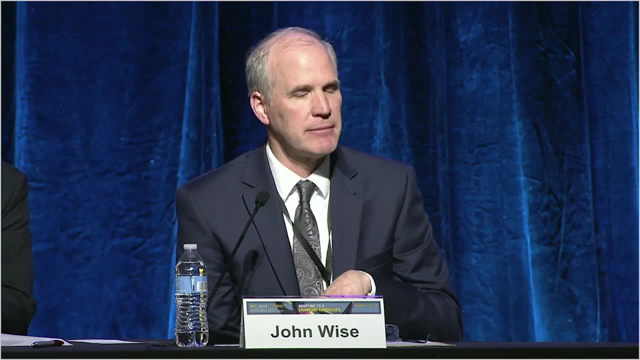 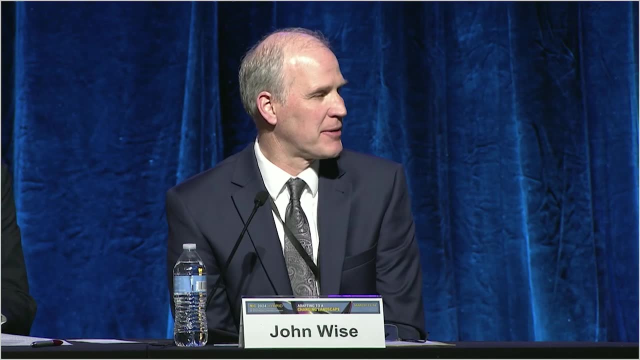 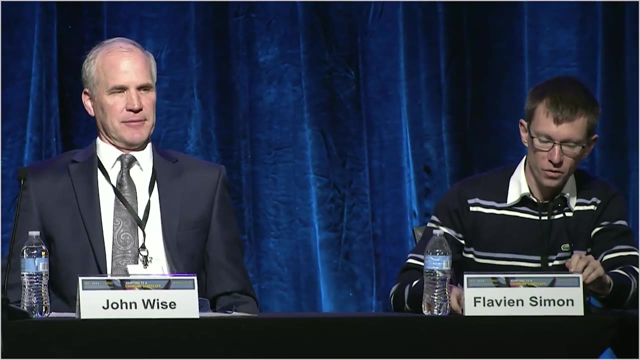 you know, not only evaluated for at their plant that experience, but also pushing that experience out to the broader industry. With that I guess I'll just turn it over to any of my other panelists. So first there is something particular. 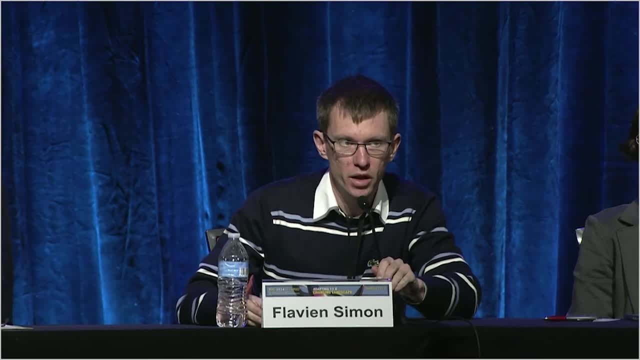 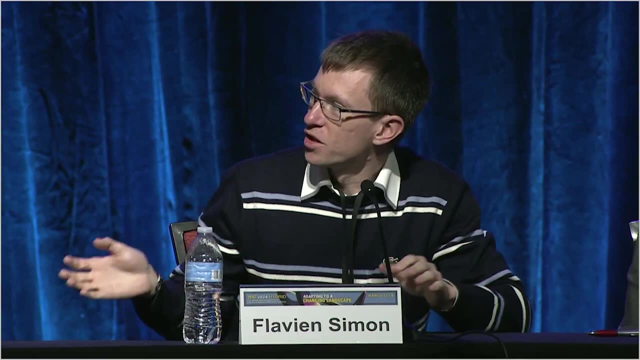 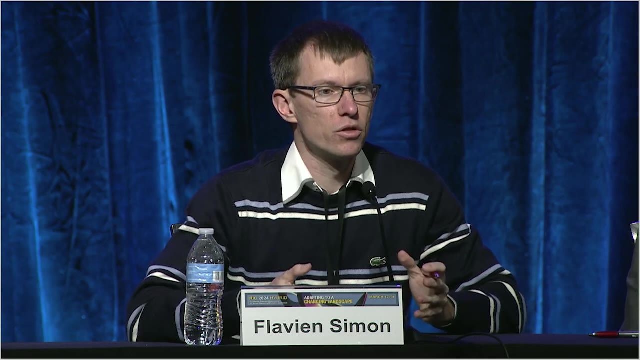 in France, because we have 56 operating reactors but we only have one licensee. So this makes the landscape a bit different from what it is, for example, for NRC or other regulatory bodies. So the discussions will be one-to-one. 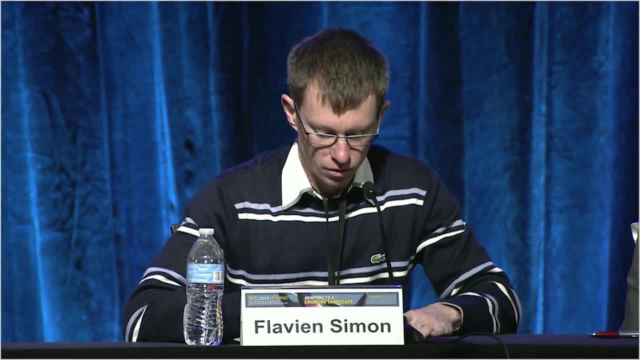 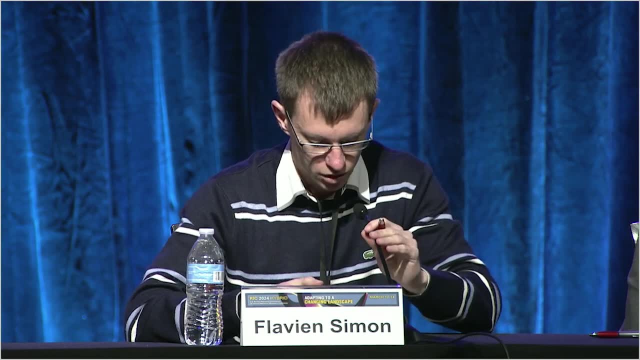 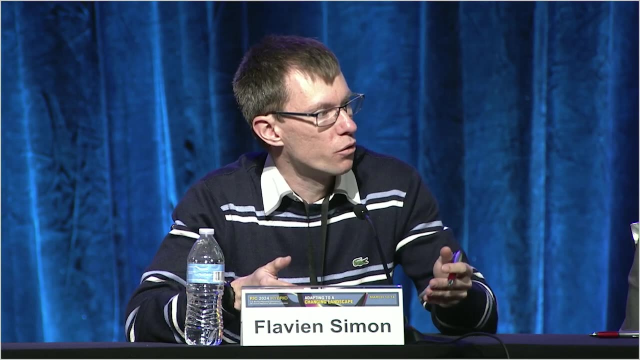 between our licensee and the ISN, And I would say that the licensee's responsibility would be to take actions in order to assess the issue, First to understand its causes, then its implications on the safety of its plants and, after that, to take the correct 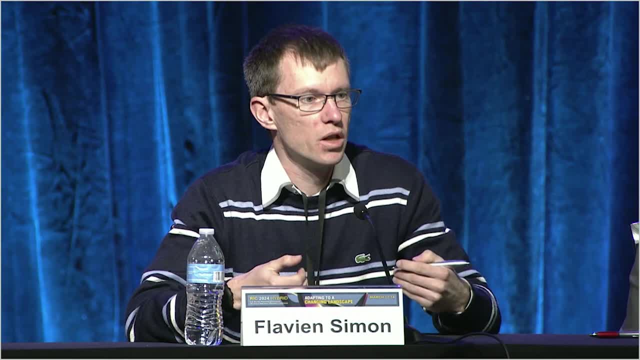 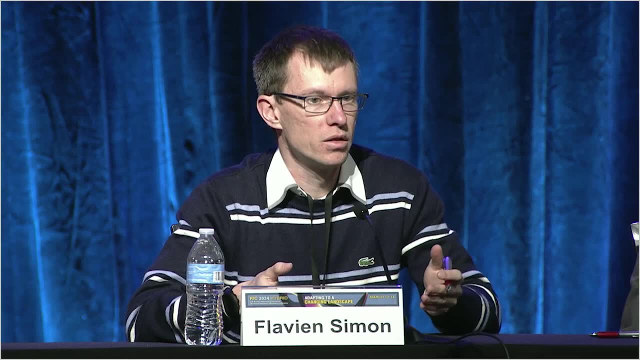 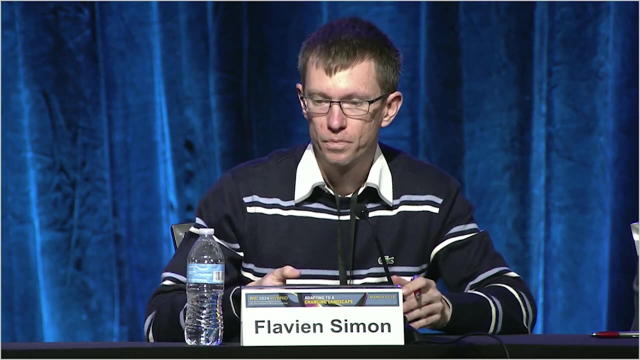 mitigation actions, And the role of the ISN would be to make sure that these actions are appropriate And, if not, to make the licensee take the appropriate actions. So maybe it's a bit simplified to what you have to do in order to. 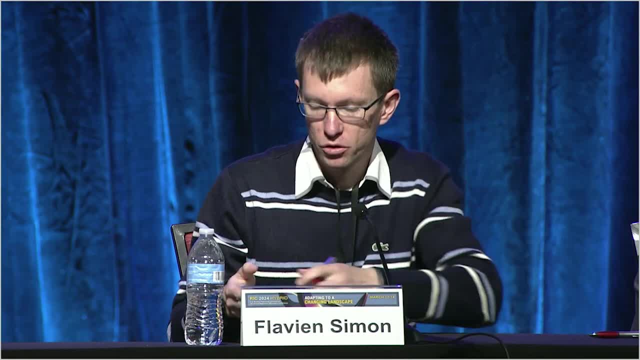 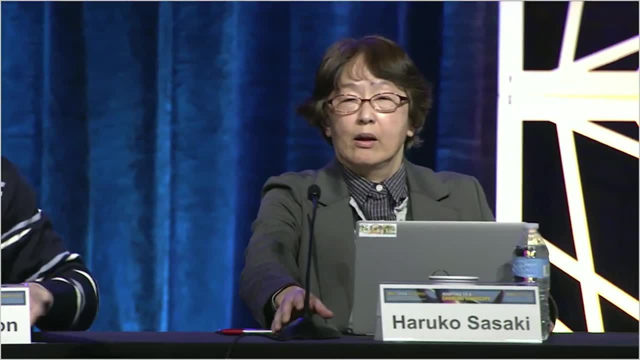 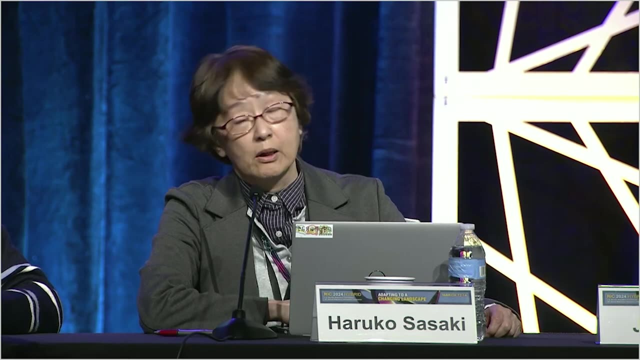 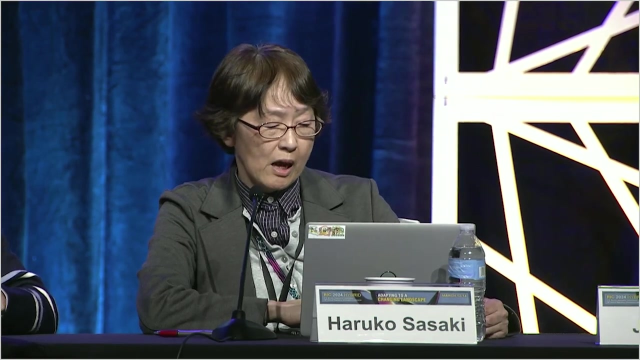 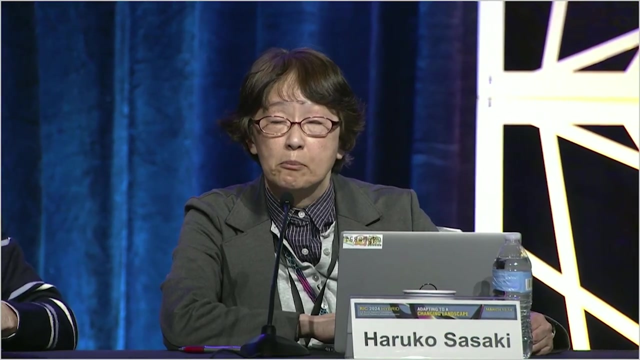 share the information that occurs on a particular plant to the other licenses. Of course, the licensee and industry are required to investigate the cause, But NRA is very active and plays a good role in assessment to identify the safety impact And if the aging issue is. 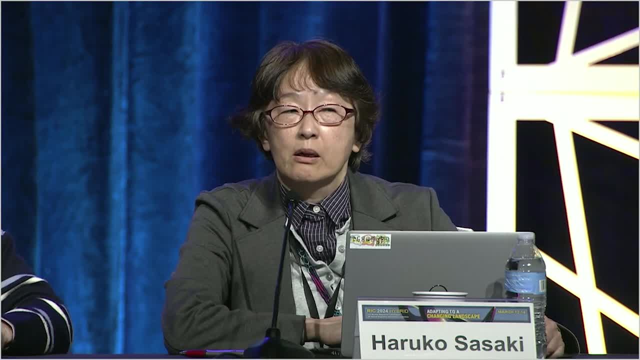 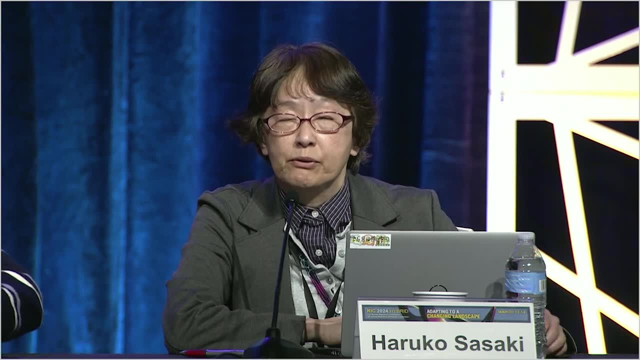 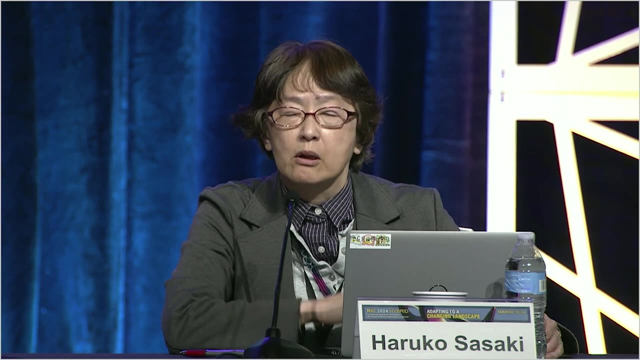 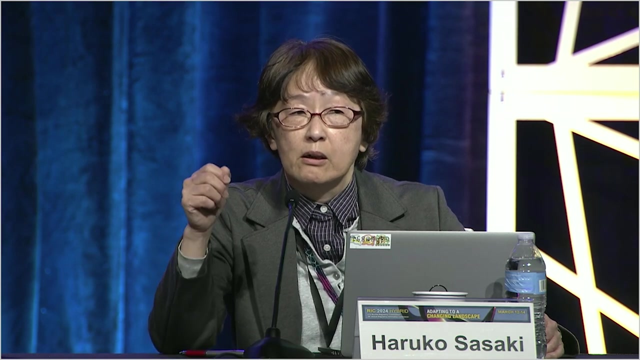 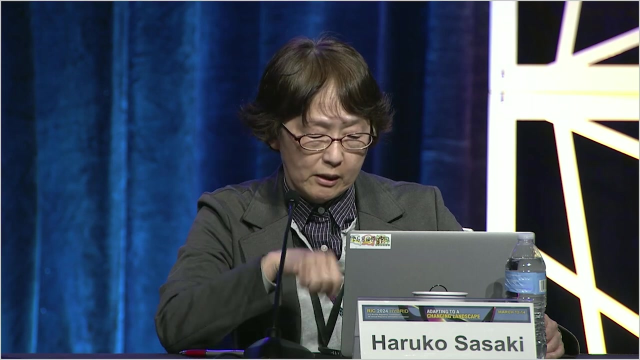 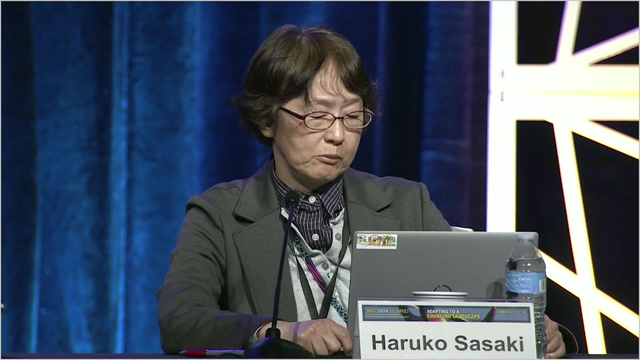 very important to safety. NRA will use a back-fitting system, because we have a back-fitting system and revise the requirement and after that the licensee has to allow the new requirement. And recently Atomic Energy Agency Atena had actual action in response to. 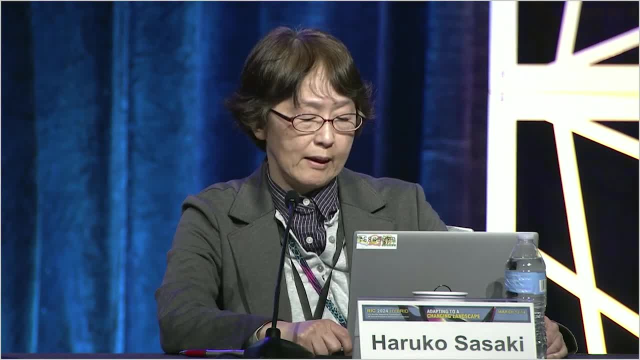 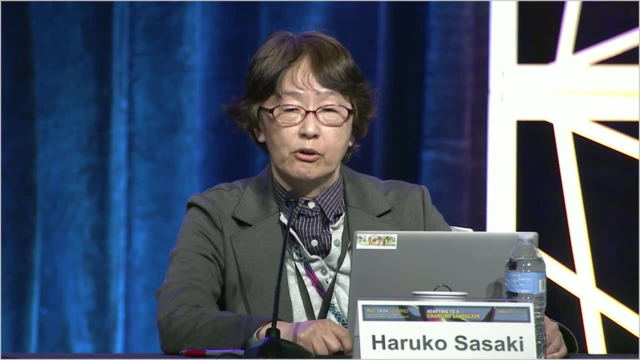 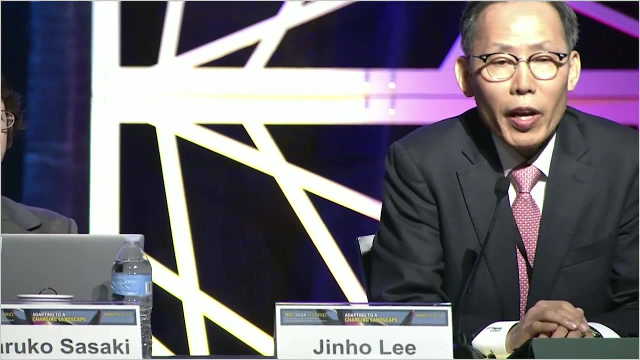 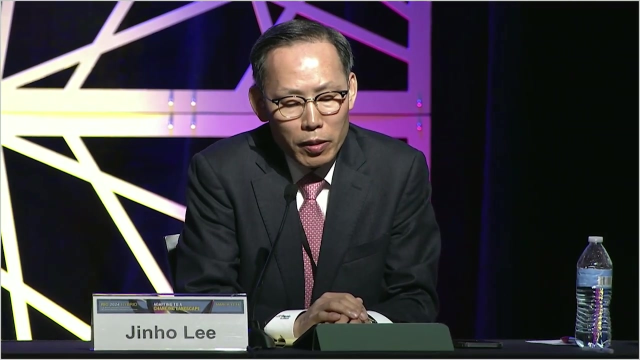 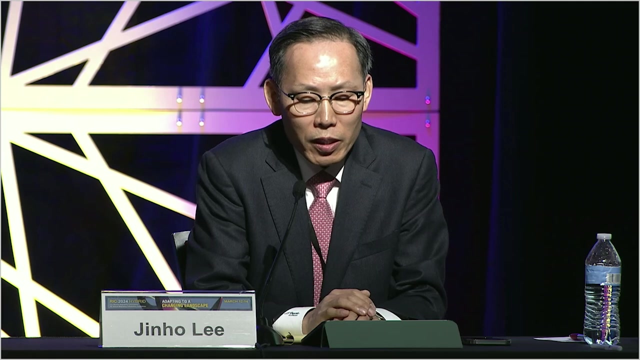 regulatory request or expectation from the NRA. This is recent activity from the industry. I think in Korea and the world a typical role and approach of regulators is almost the same. Their role is to investigate similar cases home and abroad, identify aging mechanisms, inspect other. 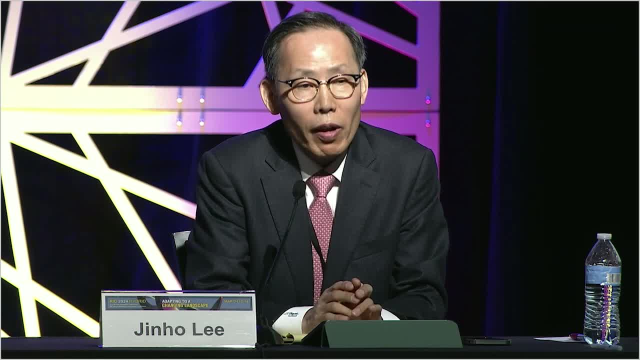 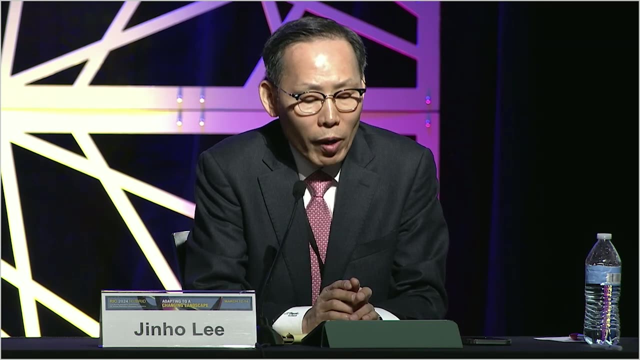 related nuclear power plants and take corrective actions. The typical role of the licensee and industry is to take the necessary measures and to disseminate the operating experience at home and abroad. However, when a new expected aging issue arises, it is not easy to find the root cause. 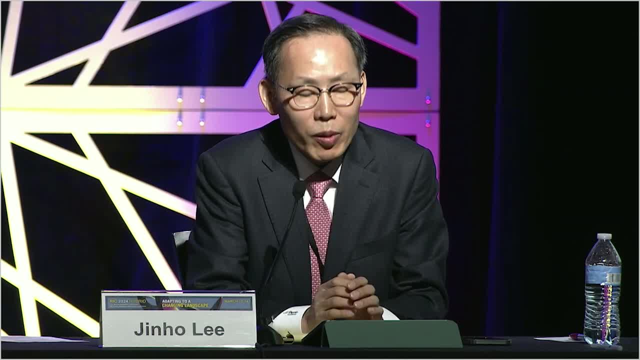 in a short period of time. Therefore, I think that it is important for regulators and operators to conduct R&D appropriately to their respective roles And, in parallel with this, I think it is necessary to continuously find and eliminate blind spots through mid- and long-term R&D. 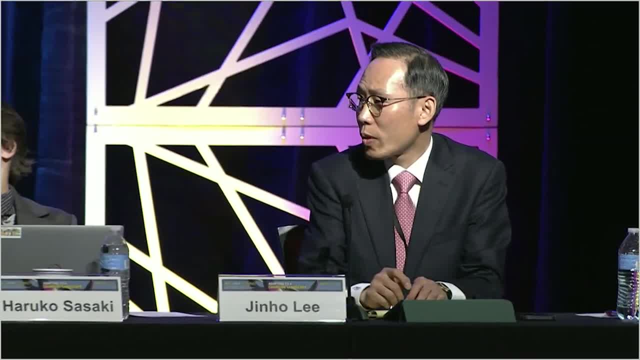 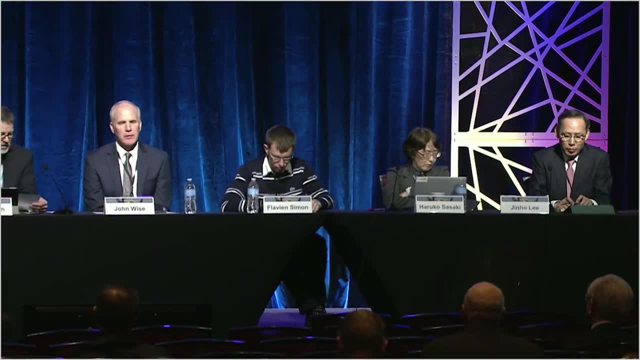 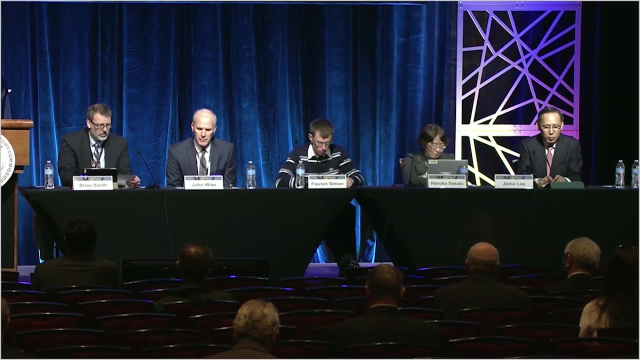 Thank you. So another question that I think most of us on the panel here might be able to answer is: as nuclear power plants operate for longer periods, what challenges do you see in preparing for and mitigating new or more significant aging mechanisms? We'll start with Blavian. 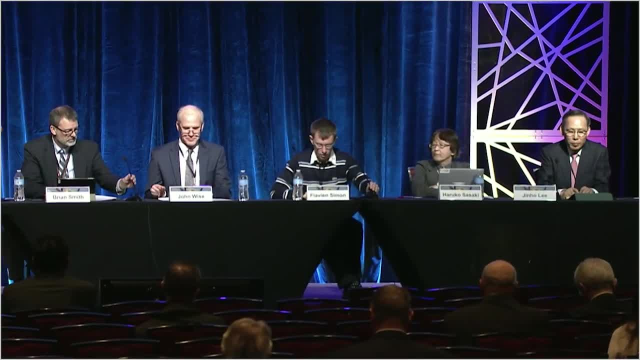 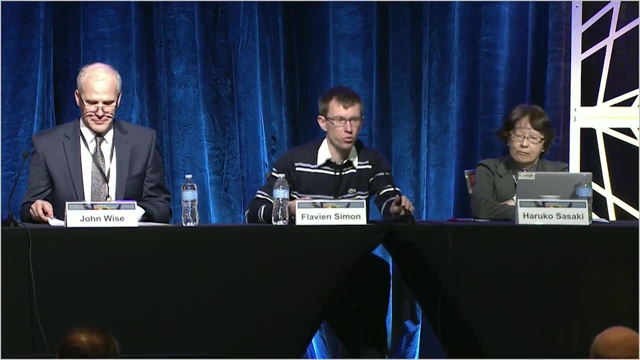 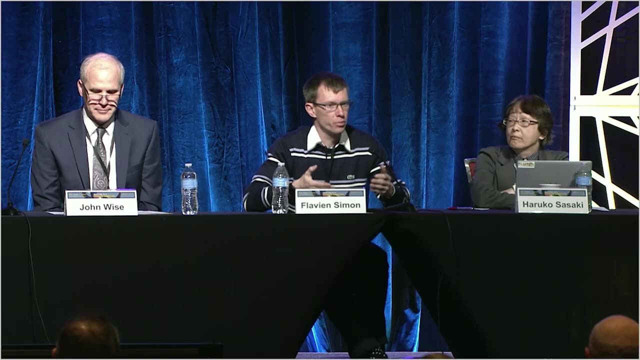 You want to take that one. One of the biggest challenges- and it may also be particular to France- is that we have a standardized type of reactors, So there is always the possibility of an aging mechanism appearing and quickly impacting a lot of reactors and therefore threatening. 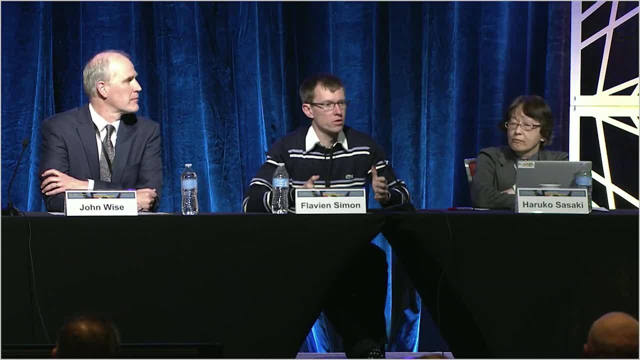 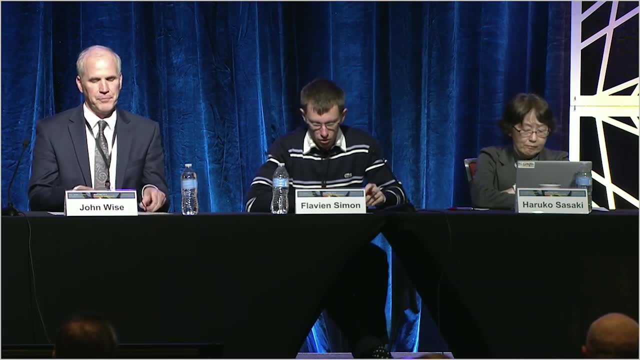 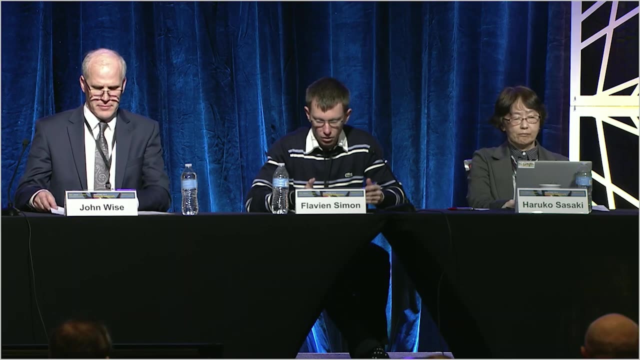 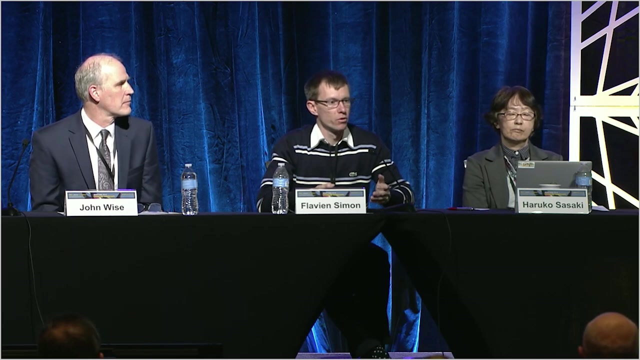 the electrical power supply, which obviously makes things a bit more difficult, especially if the regulator is not directly concerned with energy production. So I think this raises the importance of inspection in order to detect the more quickly, in the more reactive way, those new aging mechanisms. 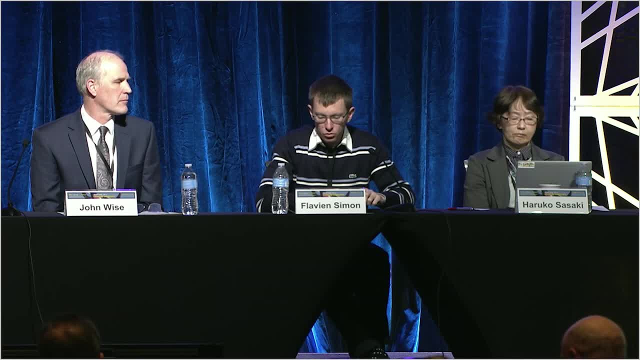 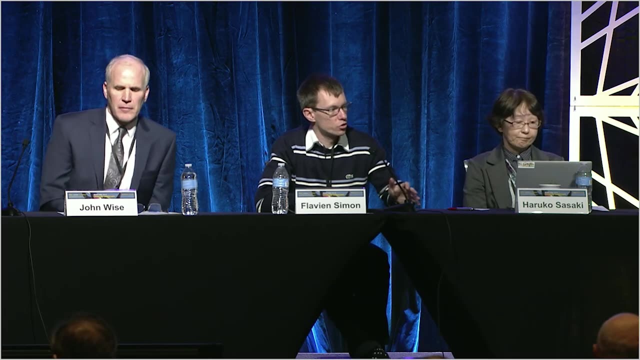 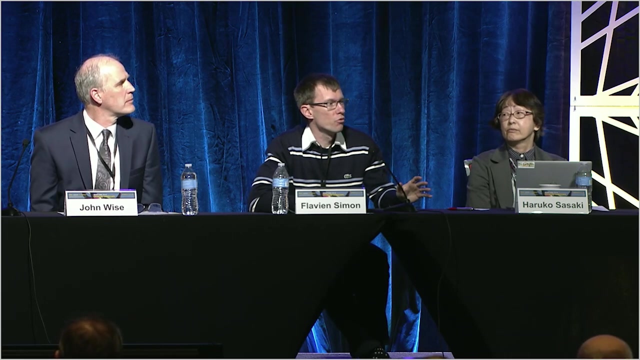 It is very important to be able to detect them quickly in order to take reactive actions. For that, I think, we need first, obviously, to take into account French operating experience, but also international experience, as you have pointed out in your presentations. I think this is very important. 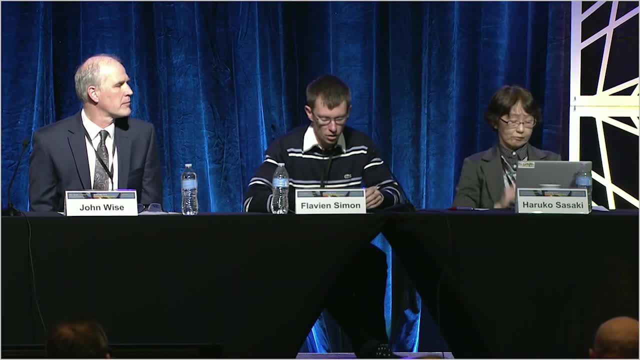 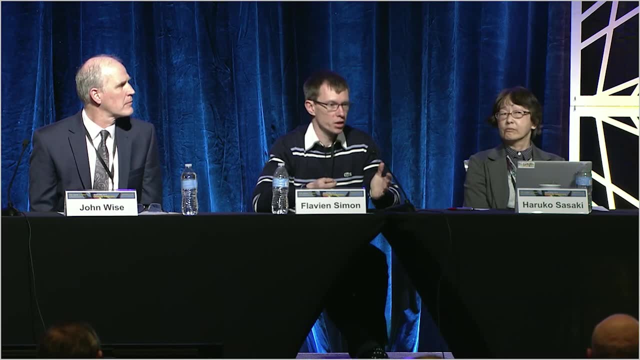 We may not always be reactive enough to share some information. Another important thing is that there will always be some things we can predict, but there will also sometimes be some things we are not able to predict. What we faced in France with the discovery of SCC. 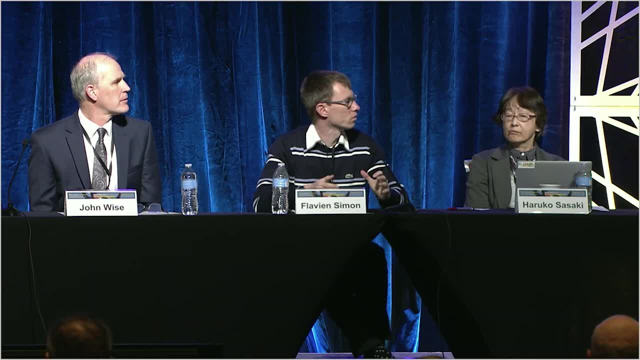 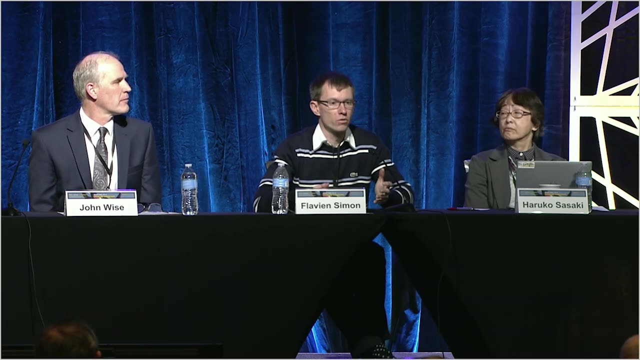 impacting a lot of reactors, sometimes with a high number of cracks affecting some safety significant pipes. it was completely unpredicted, So our inspections also have to take into account the risk of finding something in some systems that are not believed to be protected by some non-degradations. 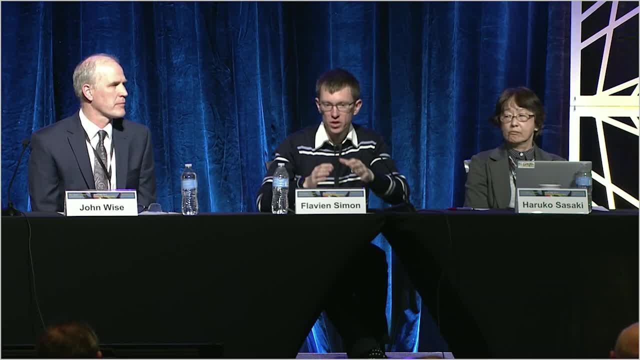 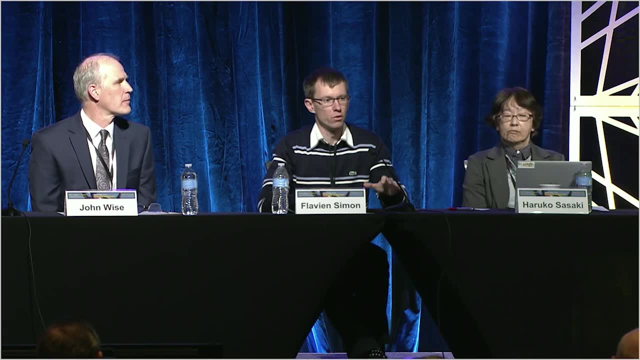 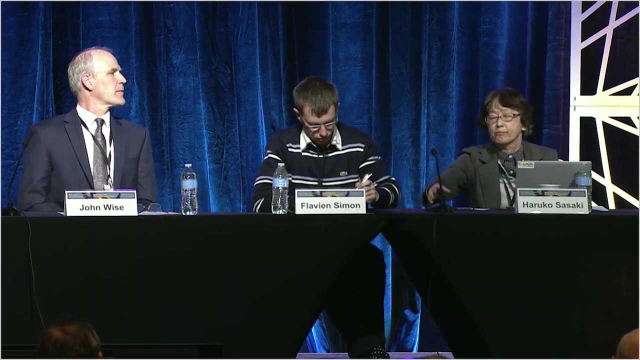 So I think the challenge would be to have the appropriate inspections done on the risk, on the parts that are concerned by some risk, but also to have a few inspections, the right amount of inspections, on some other parts of the plants. So my thought is similar to Flavien's. 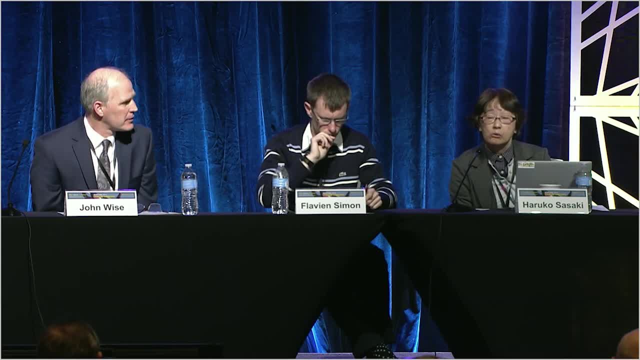 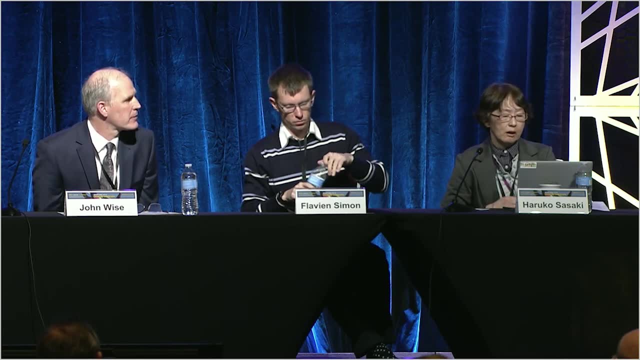 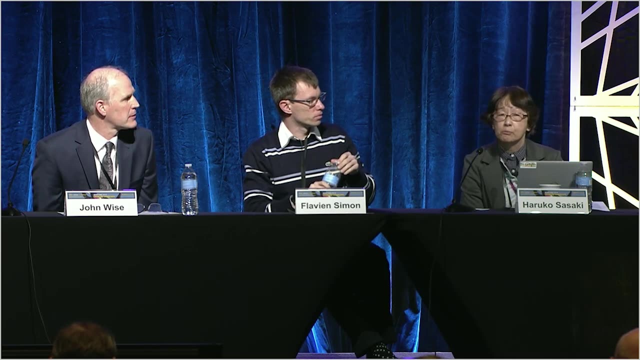 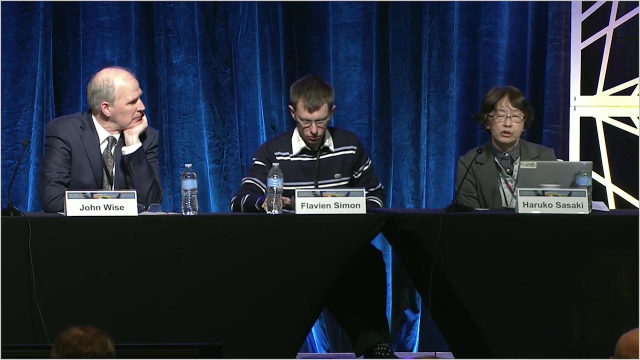 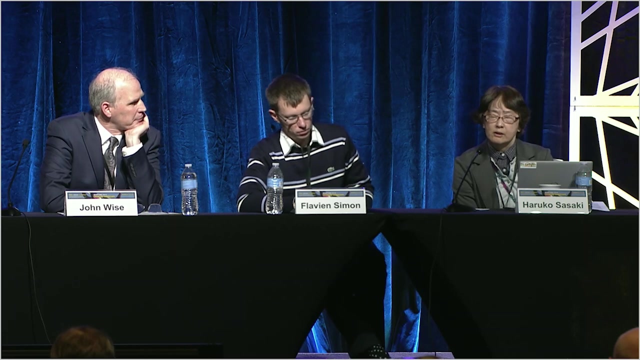 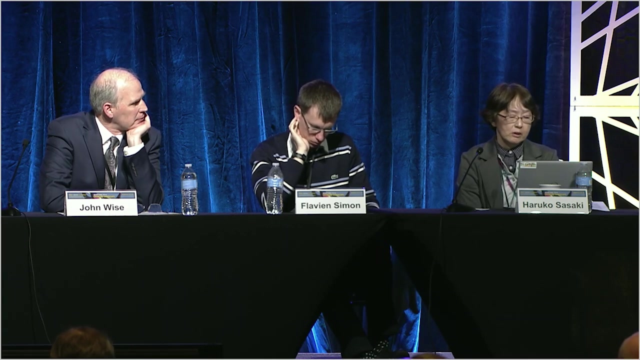 I think it's very difficult and unknown technical issue. Important is important. operating experience sometimes came from the service inspection but it is necessary to reconsider traditional inspection program because I don't know that that is appropriate to the LDO. So I think the safety research 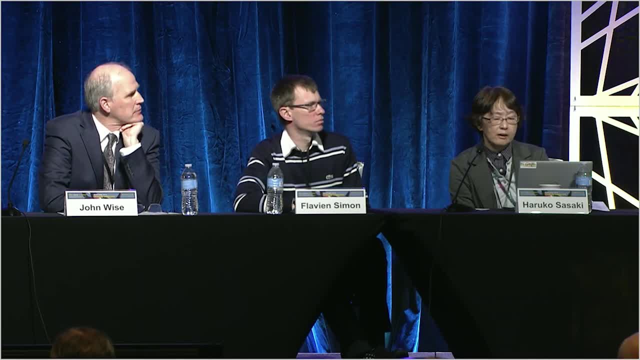 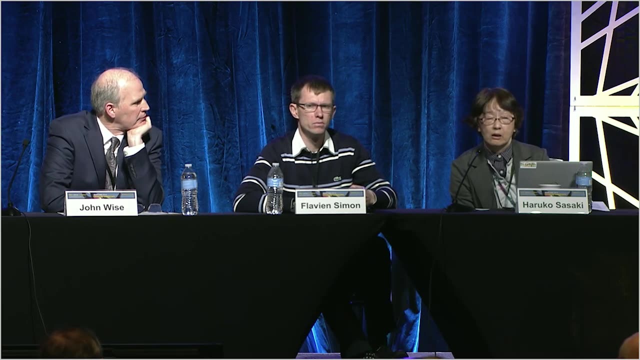 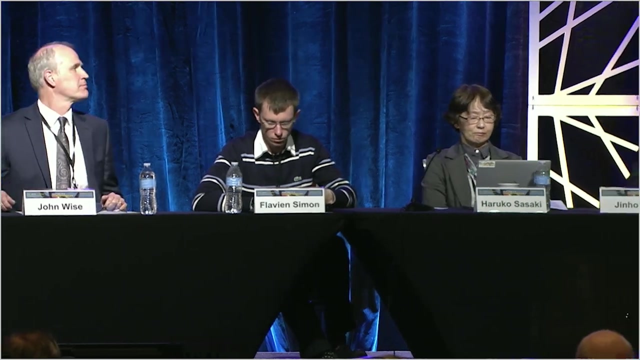 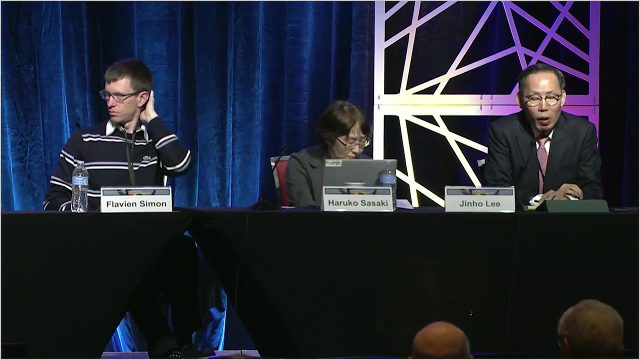 is important to take LDO into account and NRA has many kind of safety research. I think it is very effective to find the unknown technical issue. In Korea, the situation is different from other countries in that nuclear power plants are continuously being built. However, 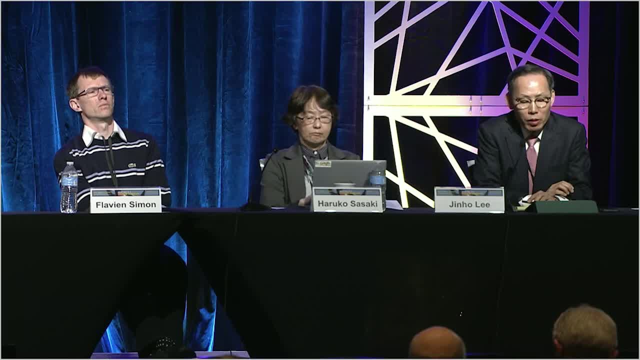 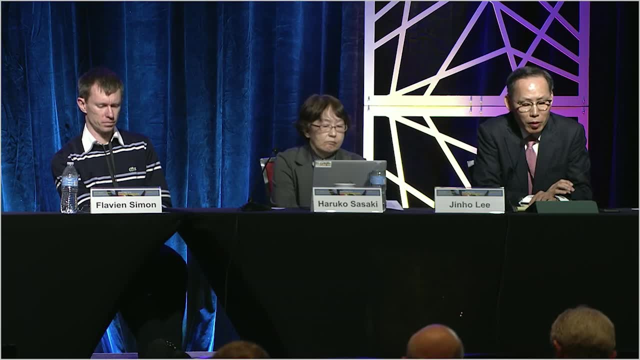 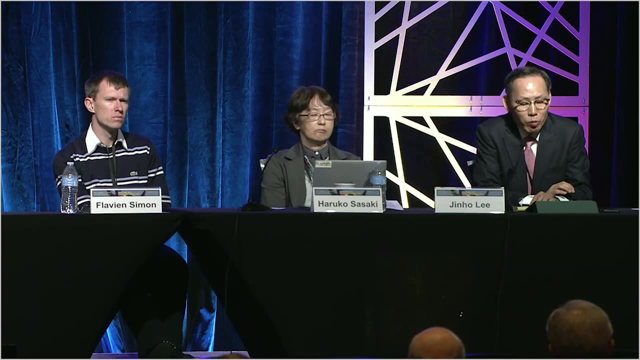 this is not only has advantages, but also have disadvantages. Recently, in Korea, applications for construction permit operating license- many PSRs have been rusting together To focus on safety significant issues, including new or more significant aging mechanisms. we need to establish streamlined and more efficient process. 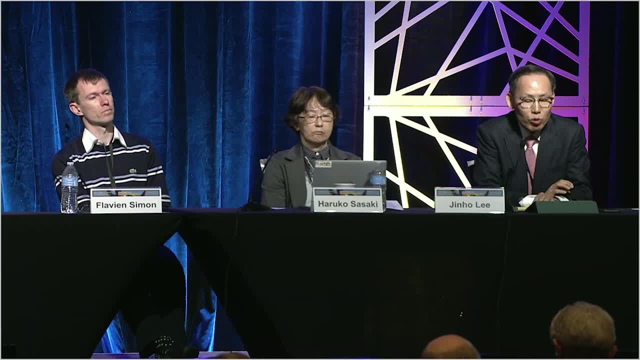 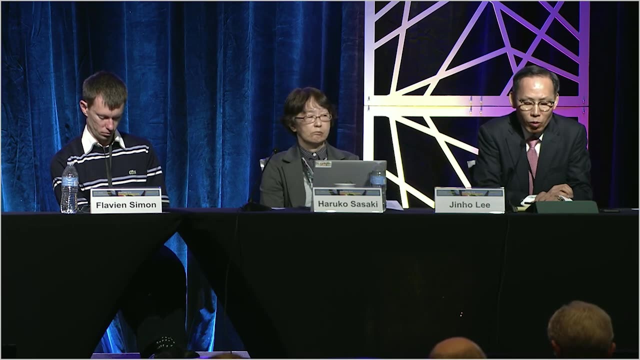 I think that this is the most challenging one in terms of the review process. In the technical perspective, I think that the most challenging one is to identify unknown aging mechanism in a timely manner. This is because unknown aging phenomena continue to appear even though a large amount of data is. 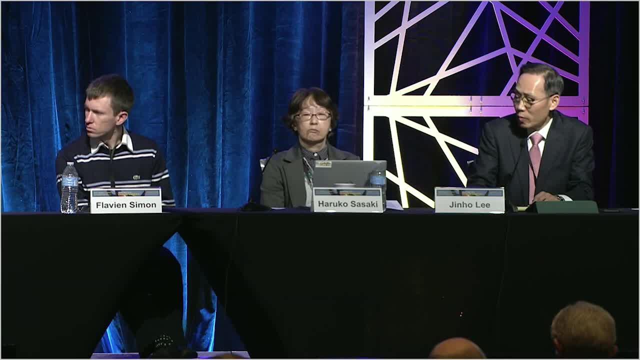 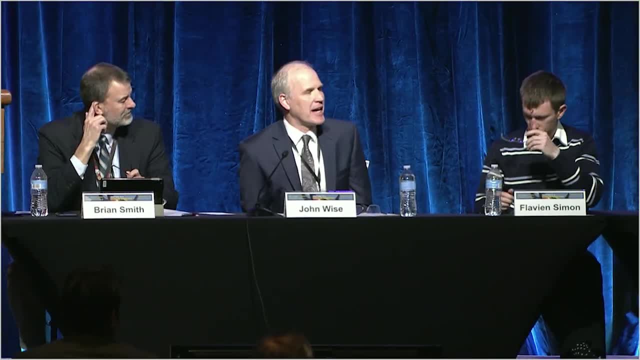 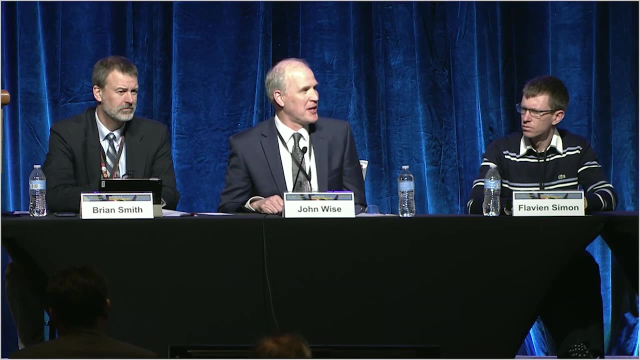 accumulated. So I was just going to expand, because I think you have seen some common themes here: This idea that we don't know everything, and how do you develop an inspection program when unknowns may or are very likely to emerge. So we talked about 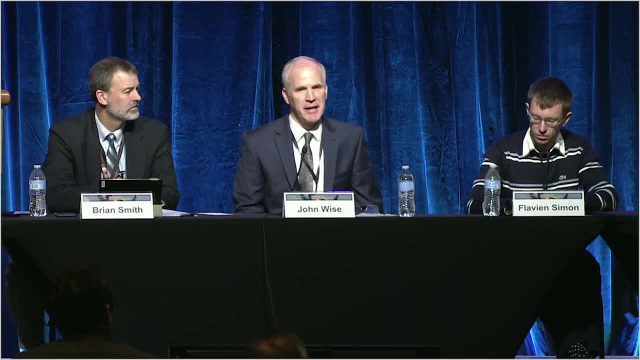 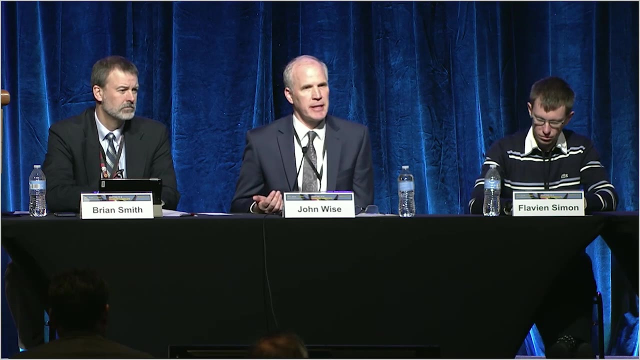 some different aging mechanisms that were brought up in this panel today that emerge after quite some time. So, if a you know, we're all always looking to be more efficient in our inspections, As in regulators, we're often presented with proposals to take a more risk informed approach to our inspections. 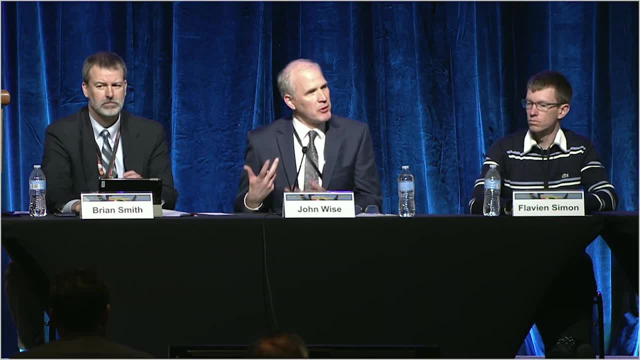 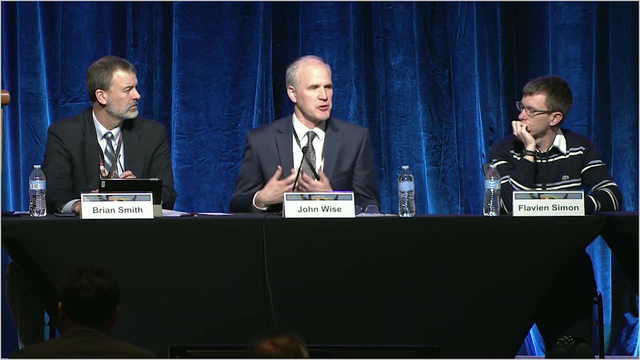 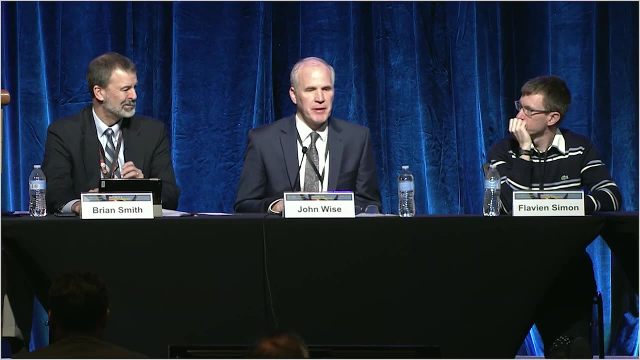 Don't spend so much time looking at the components where the past evidence of failure just isn't there, for example. But what the struggle of the regulator is is how do you handle the unknowns as well as the fact that some of our components have a 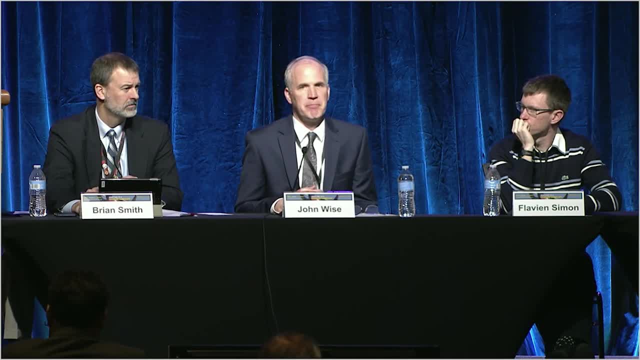 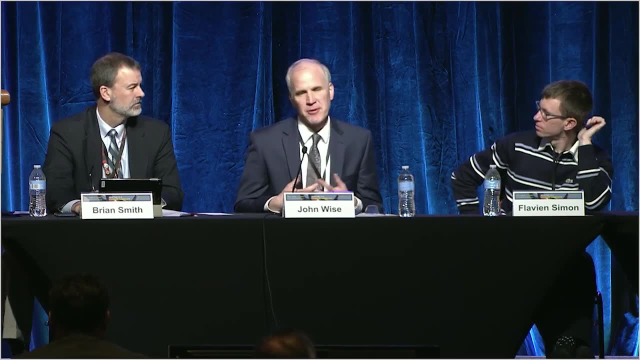 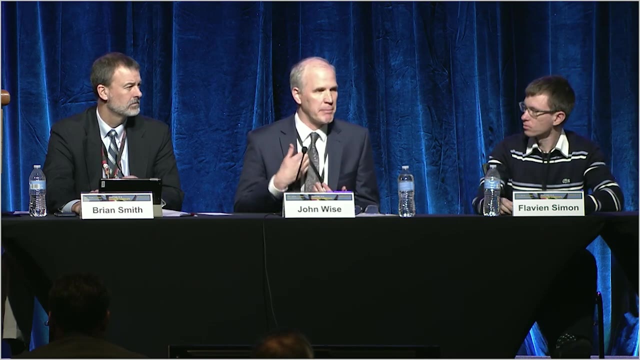 very good operating history, with no failures, because there was a very rigorous inspection program in place. So if you have a very rigorous inspection program- for example, an ASME code program that looks for evidence of degradation and directs repairs in a timely manner, you simply may not have. 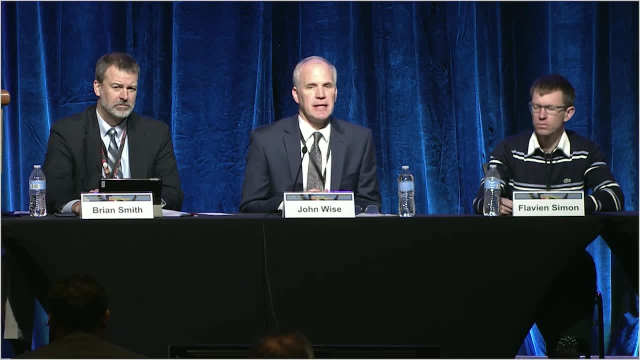 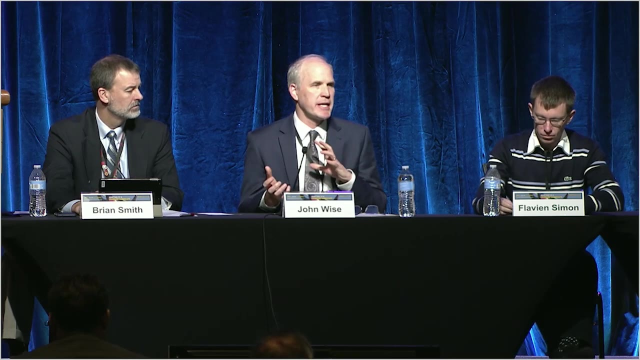 a population of components that have experienced a failure And that can be challenging because that doesn't show up as a high PRA number, for example, as a susceptibility risk, And so, as a regulator, when we're presented with again making more targeted or efficient use of inspections. 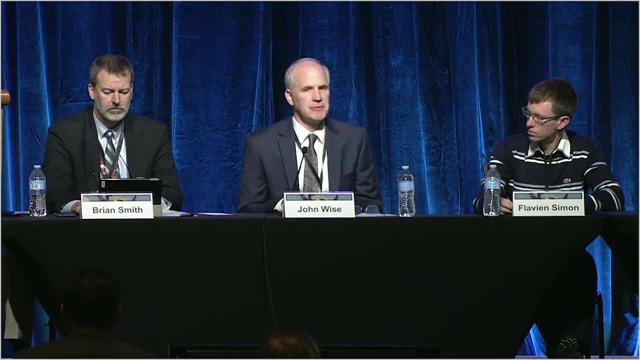 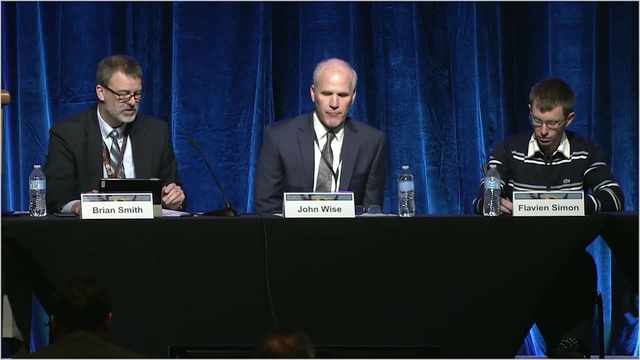 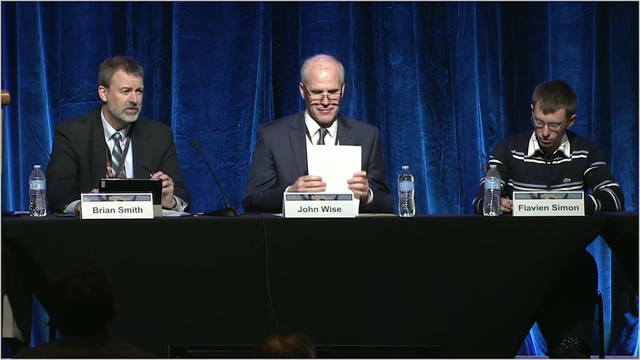 we always have to sort of keep these things in mind and that's a challenge. Thanks for those responses. So multiple panelists here have mentioned risk just in that response, And risk and being risk informed and using risk insights has been discussed a lot in this RIC. 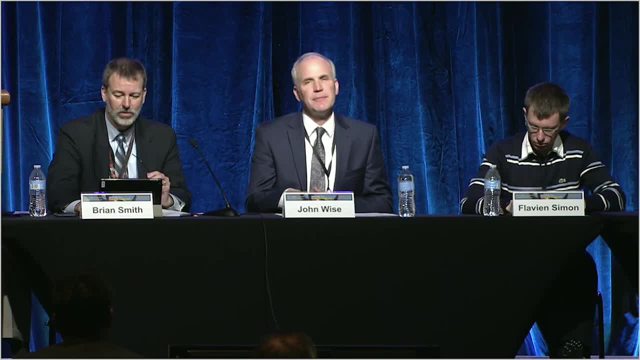 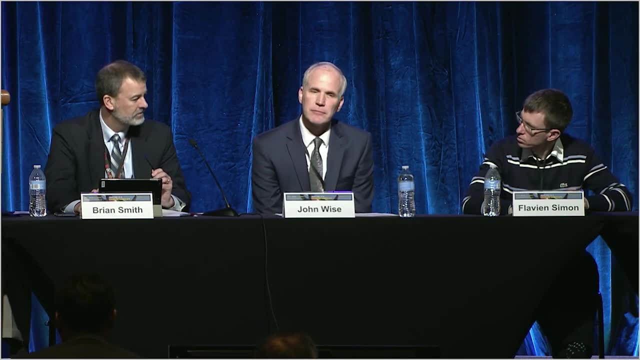 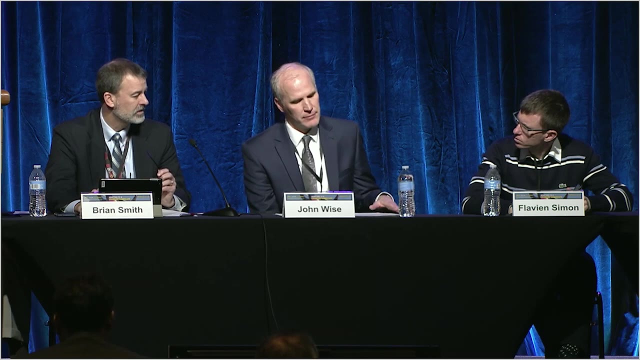 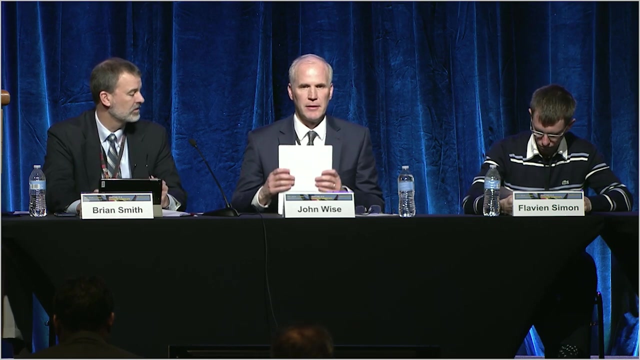 and for many years back as well. We've gotten a couple questions related to risk from the audience. so long term operation a lot of times focuses on passive components. How can we incorporate risk into license renewal or long term operation and aging management programs? Is there anything going on there? 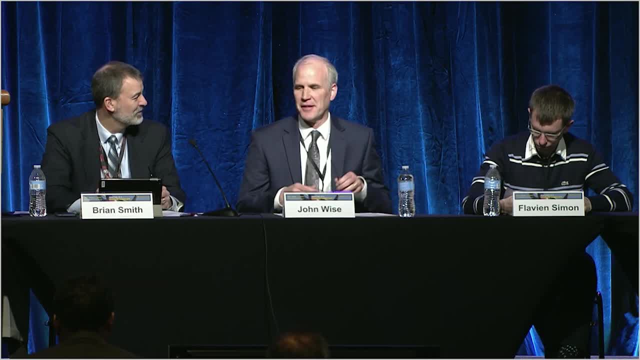 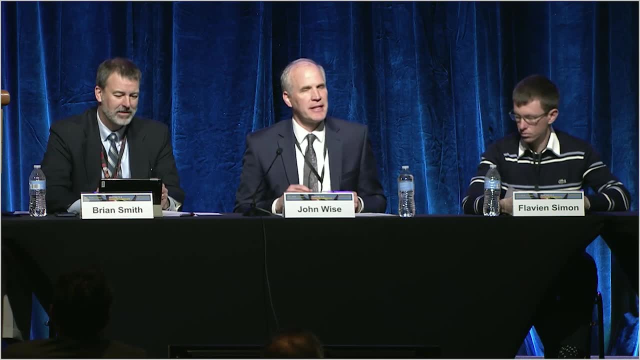 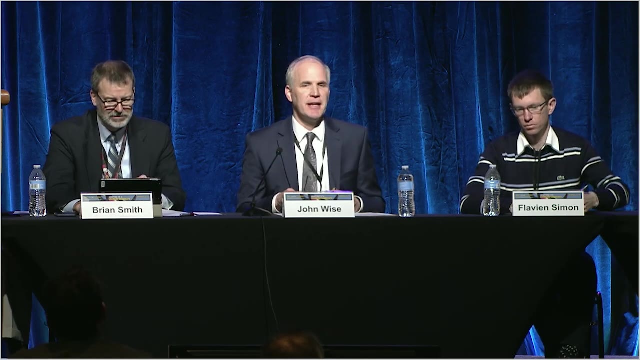 I know, John, you're actively in the middle of evaluating how to use risk. Yes, so I guess I'll. at the NRC, we're kind of addressing risk in a couple thinking of risk in a couple of different manners. at this time We're thinking about risk in terms of 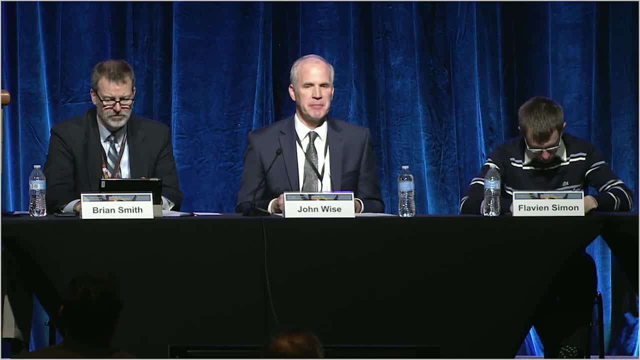 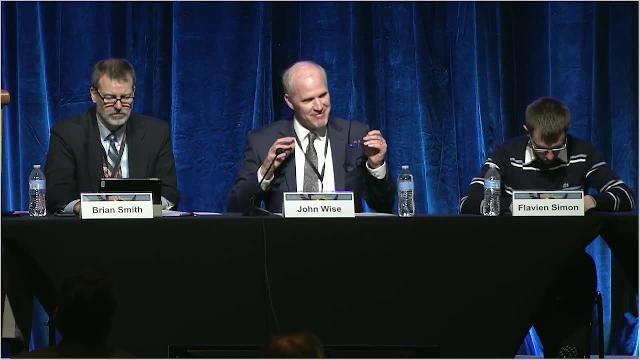 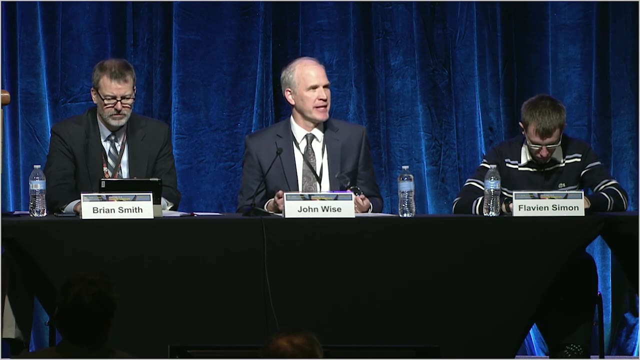 we can use risk information to determine just how thorough- I guess I'll say or deep- of a review the regulator does like. how in depth do our own regulatory reviews need to be for those systems that may be more or less risk significant? and that's an ongoing discussion we're having. 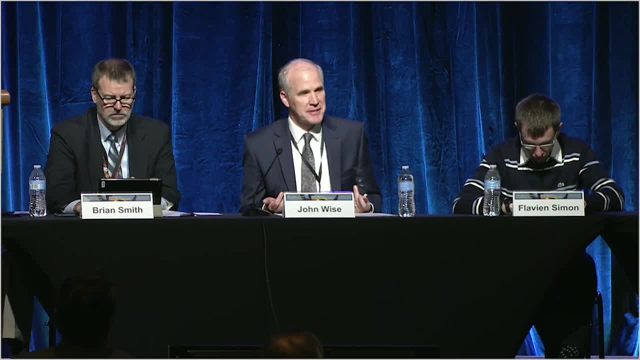 with the industry now and we are adjusting our processes right now to try to, you know, tailor the level or depth of our renewal reviews based upon the risk significance of systems. but, on the other side, another way of thinking about risk is just as I discussed in a previous response. 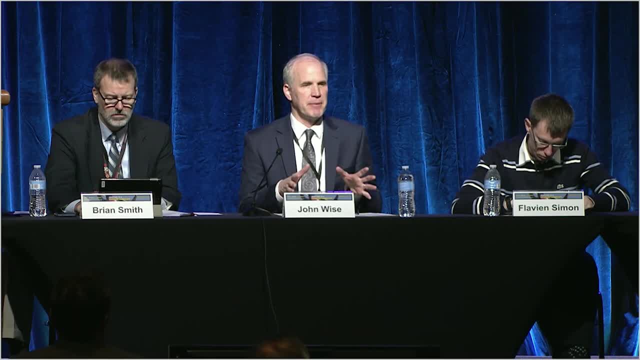 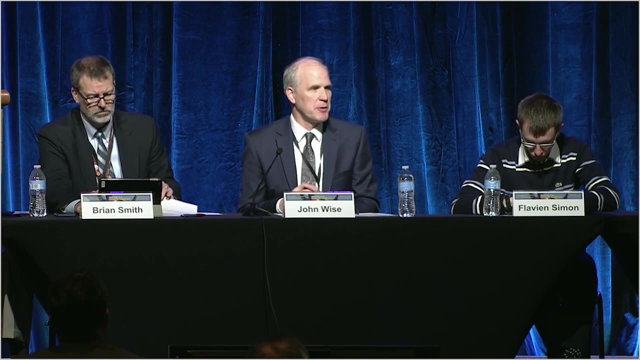 using risk information to actually shape an aging management program. How many inspections do you need to do? And so you know I won't belabor it, because I discussed it previously, but just the challenges of applying risk to a passive component. that may have been very. 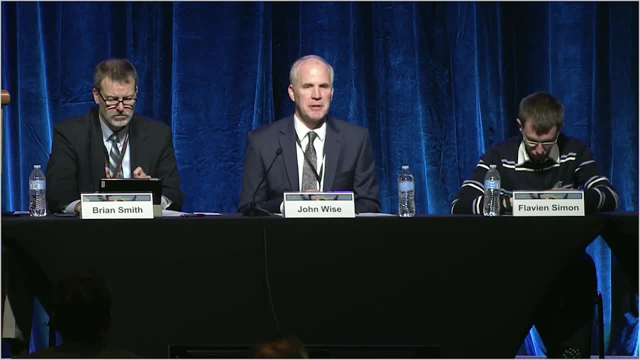 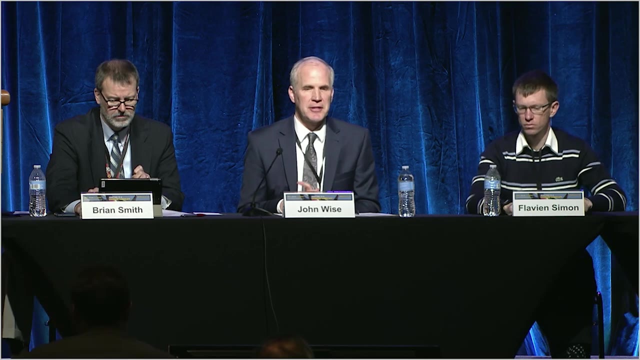 reliable over the years and using risk numbers to project future failures of such components can be difficult, especially when you're talking about very long term operations, But again, this is something that in the US, the regulators actually actively discussing these issues with the industry. so stay tuned, We'll see what happens. 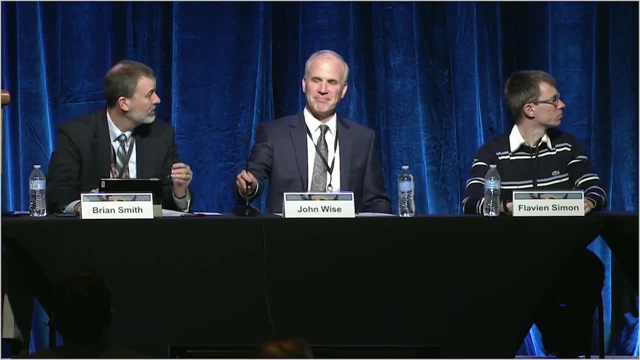 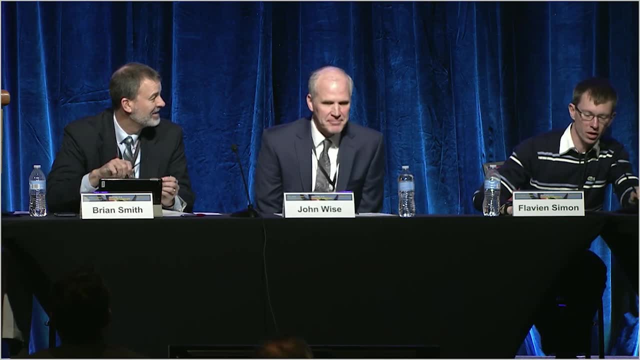 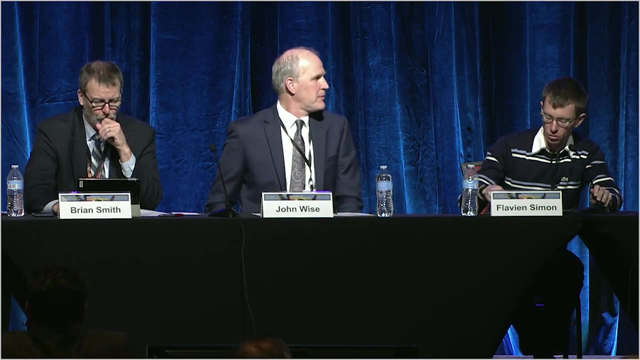 I'll turn it over to you. Does anybody else have a? are you considering risk in your activities? You don't have to answer, but Maybe something on which I can elaborate from John's answer is that of course we need to know what are the actions. 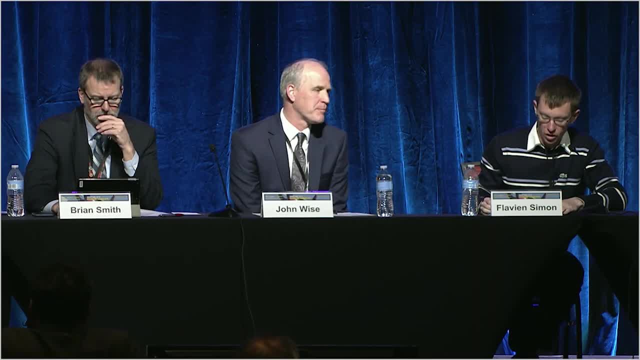 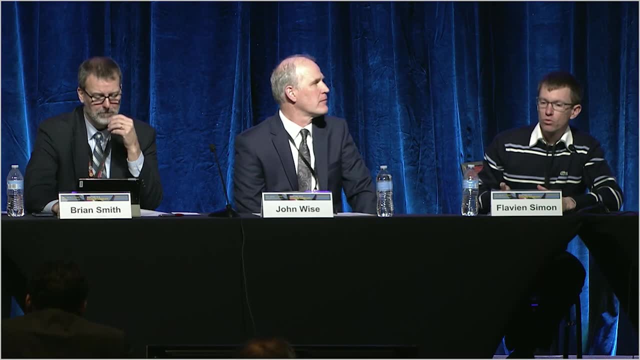 taken when there is a risk that is known and if they are appropriate. but on components that are not subject to any known risk, we still need to know what will the licensee do, and maybe one of the precise things to look at is: what is the sampling rate of? 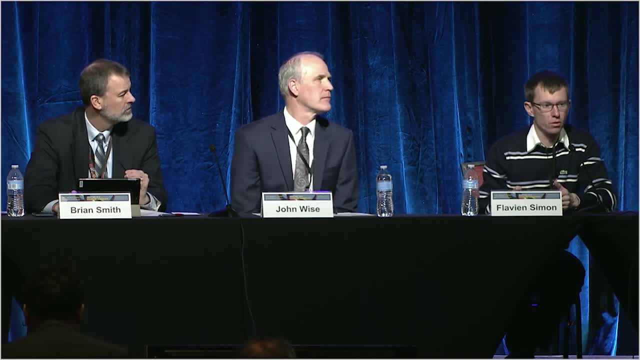 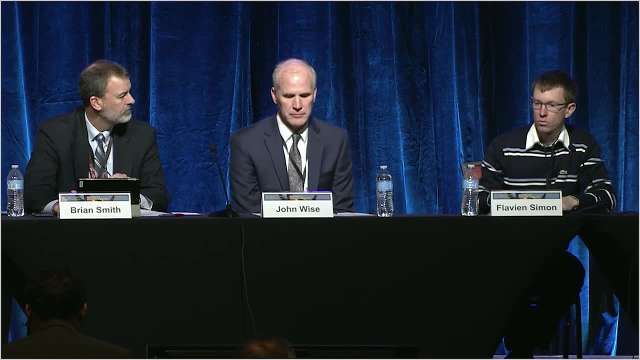 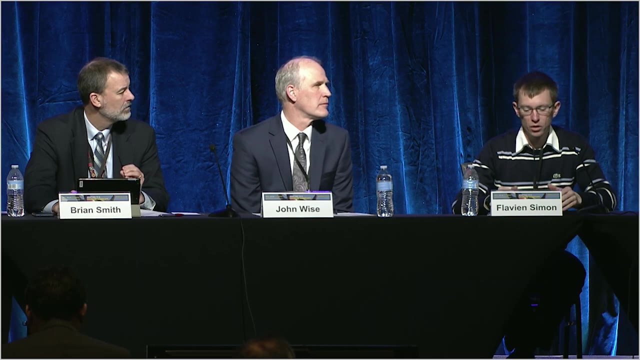 inspection programs that are planned for those type of components. I know there are some rules in some of the codes, some basic sampling rates. in France we don't have those, which means that when you're not doing an inspection program on a risk informed base, you don't have any reference. 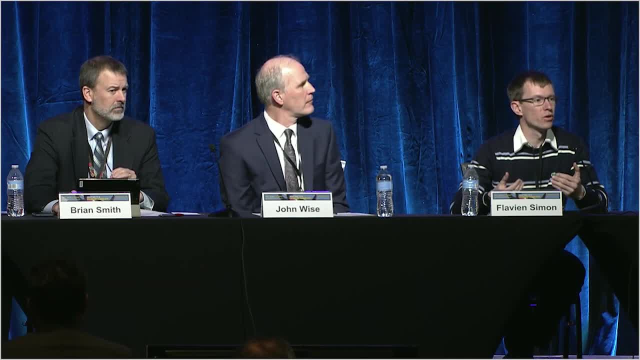 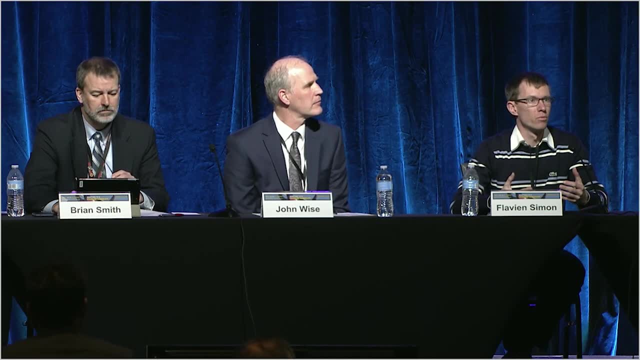 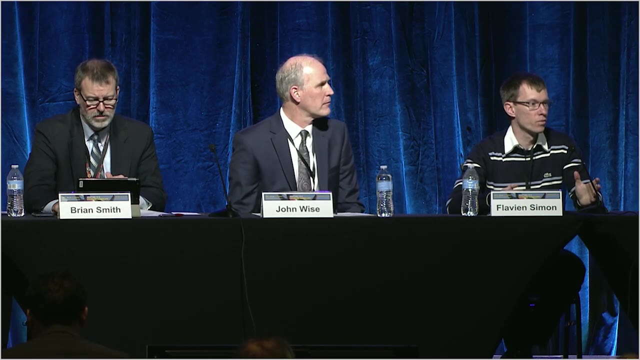 at all to assess the proper sampling rate, and I think this is something we need to think about in the next years, because it's quite a concern for me to have big, sometimes important, parts of our plants which are safety significant and which are not undergoing any inspection at all. 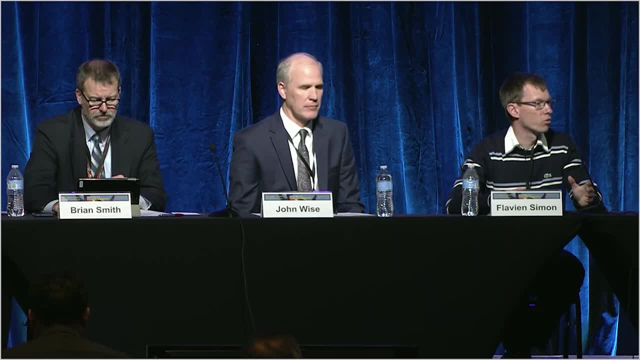 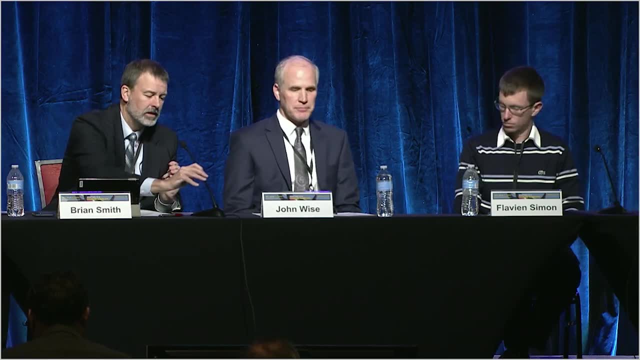 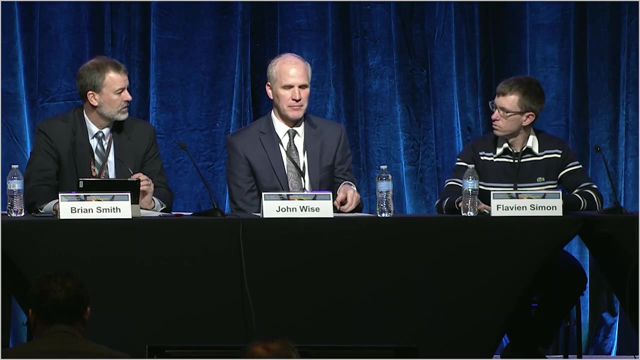 to determine what would be a good sampling rate in the future. Alright, So we had another question come in. I know it's addressed to Jinho, but I think, Haruku, you mentioned this as well, but in your remarks you mentioned utilization of artificial intelligence and aging. 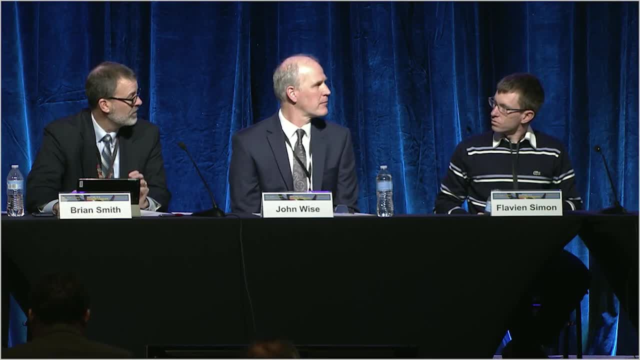 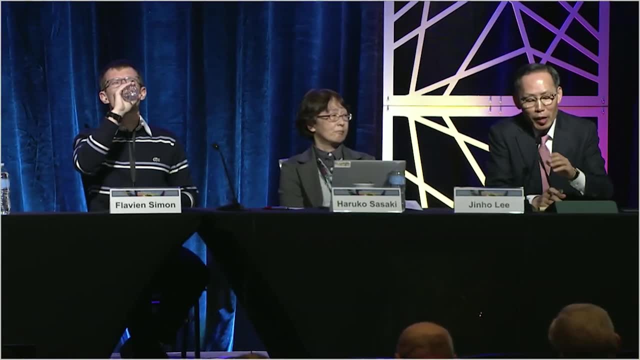 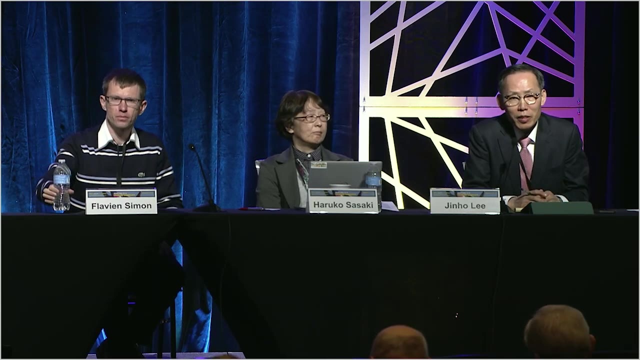 management. Can you elaborate on the potential and possible applications of it? Strictly speaking, I have no specific idea about that, but I think that we can get many ideas from today's technology. there are several examples in the case of the ISR, in-service inspections, most cases the 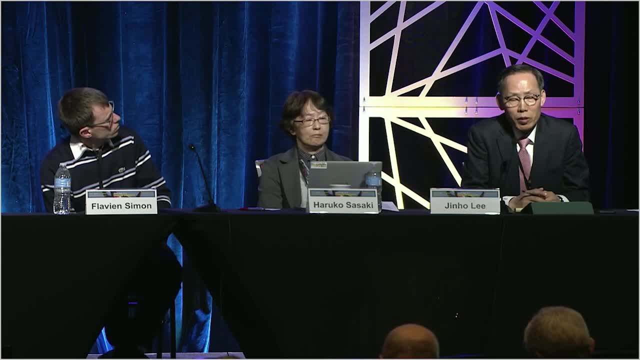 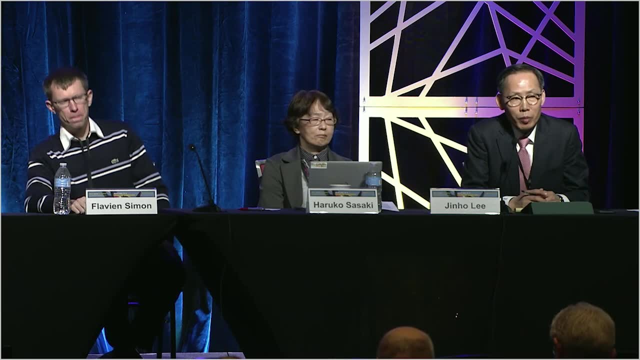 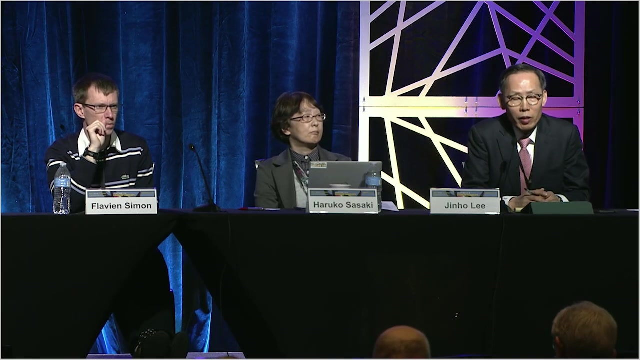 UT technology is being used. the conventional one is using the angle beam proofs, but nowadays phased array proofs are being used widely in other industrial side, because I think that those kinds of technologies can be used in the nuclear fields. Another one is to using computerized data analysis. 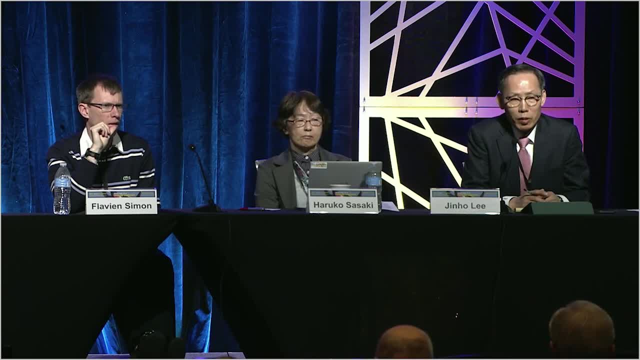 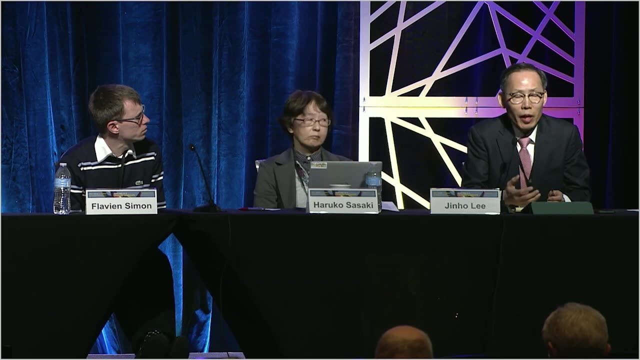 in the case of ECT, at the current method it produces lots of large amount of signals, data signals. if we use neural network and AI, then we can perform more effective inspection. and another very challenging one is to using AI pattern recognition technology. the high resolution cameras are being developed. 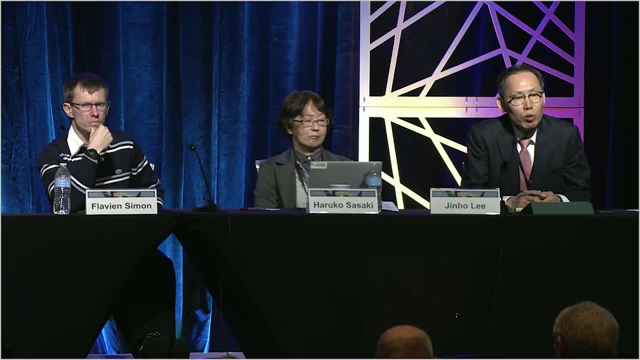 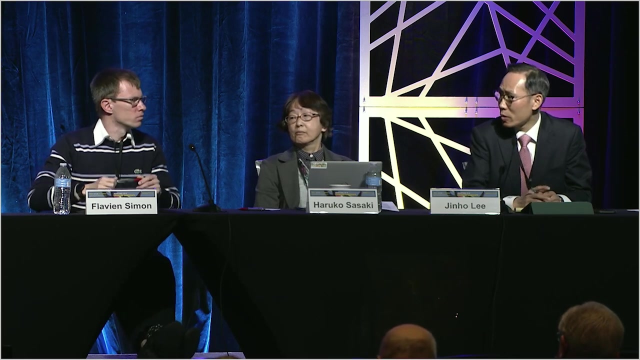 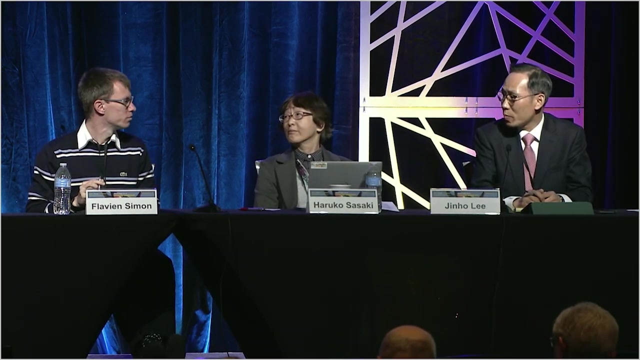 quite well these ways. If we use the pattern recognition technology, using the AI, then we can find more flows inside the reactor. that kinds of things could be a good example. Alright, thank you, Ericu. did you have any ideas? No, Something to share? 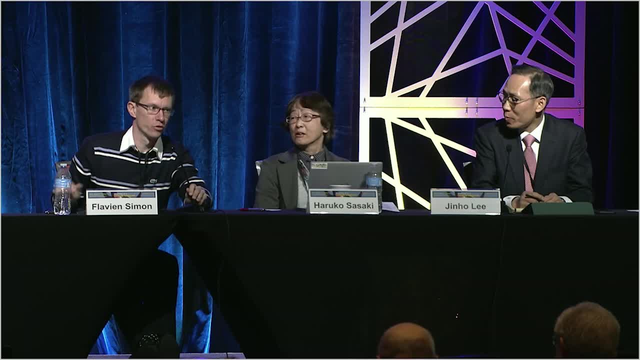 Yeah, something to share about IA, even though I'm not an IA specialist at all, so take what I think with a pinch of salt. but as I think that the principle being IA is to educate some model on some data, I'm not very sure that it's good to predict the 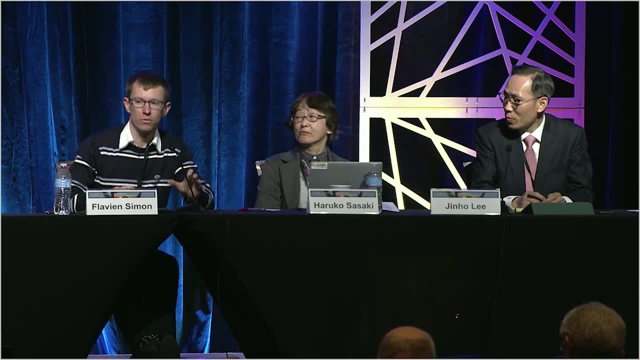 unpredicted if you don't have any sign at all. if you the data you got, I'm not sure IA will predict that there will be SCC on stainless steel in the next year. So I think we need to be, as regulators, careful about the design of some. 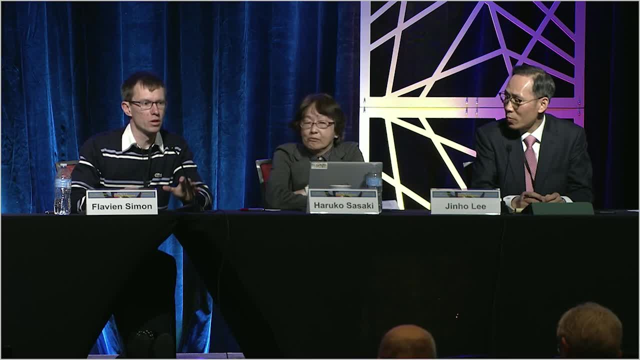 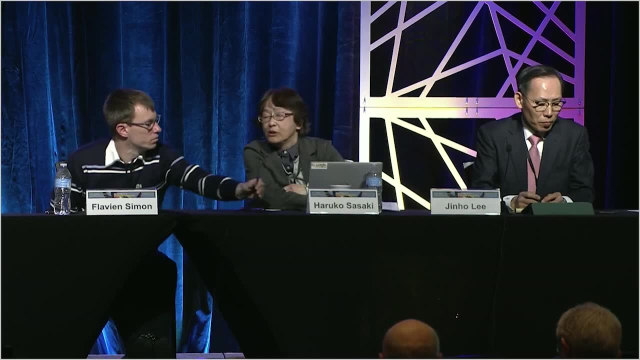 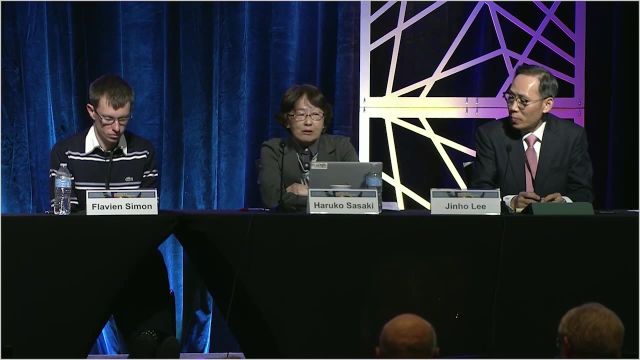 inspection or aging management programs that would be only based on IA predictions. Okay, Thank you. We just started to learning about the new technology and we are collecting the information from the other countries on stage. Okay, Okay, a question for you, Haruku. 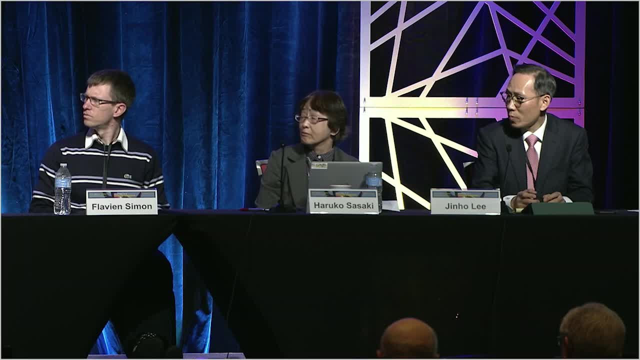 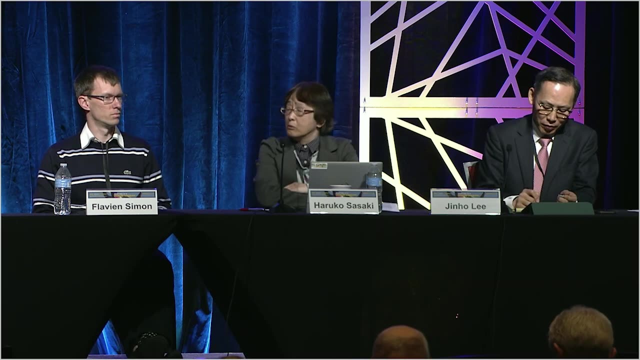 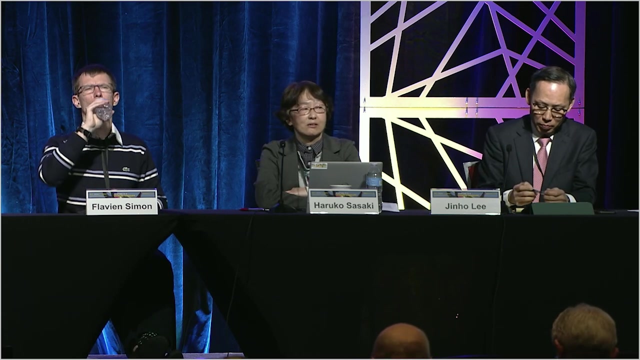 Was there any consideration for aging that occurred during the 10 year shutdown or because the plants were not operating? was that time assumed to have no deleterious effects? It's a difficult question. What you mean is impact to the industry or to the environment. 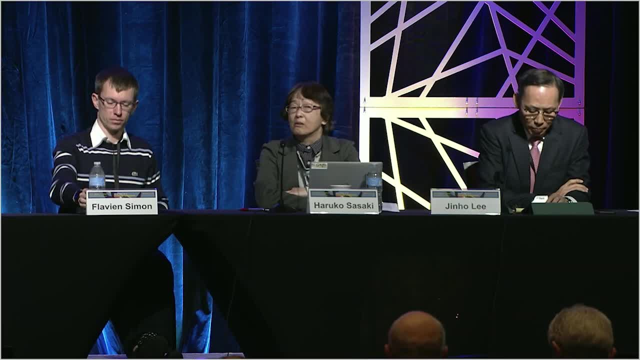 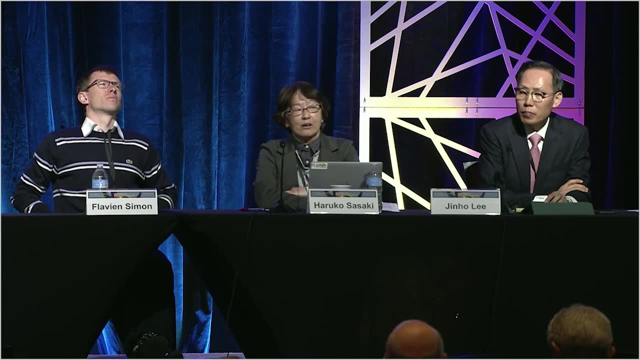 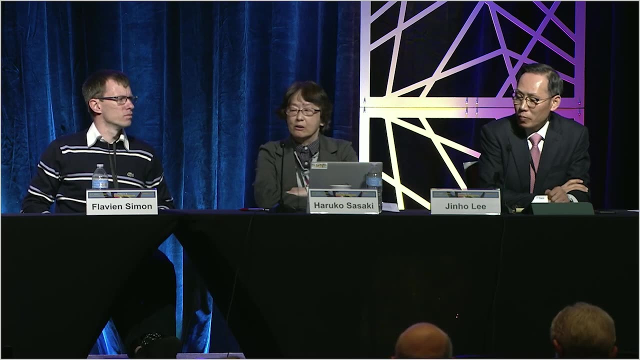 From an aging standpoint of the plant. was there anything specific you considered regarding the time that it was shut down? Yes, This is my opinion. Recency is in confusion just now And they trying to do something, for example, technical research, safety research is. 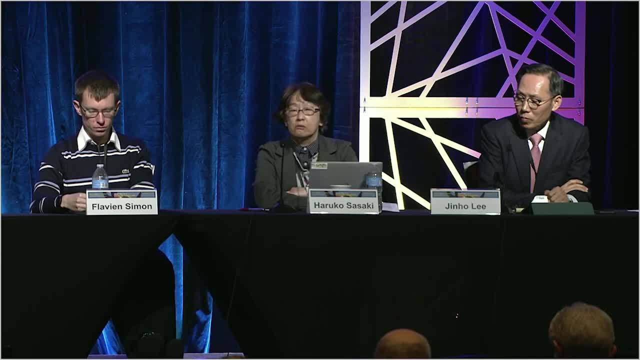 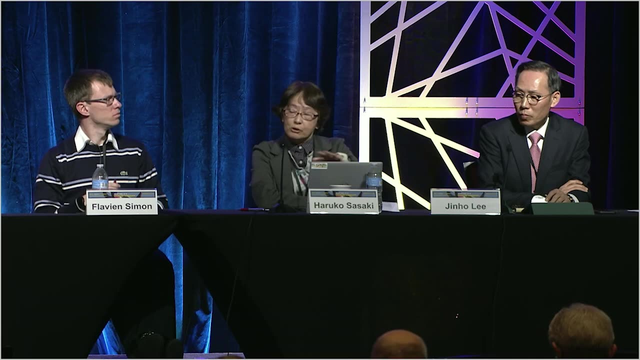 trying to use risk information method to explain about conformity of the requirement, But just now balance between industry and regulatory body is very not equivalent. Recency wants to start their plant, But we have very strong deterministic regulatory requirement, So I don't know how. 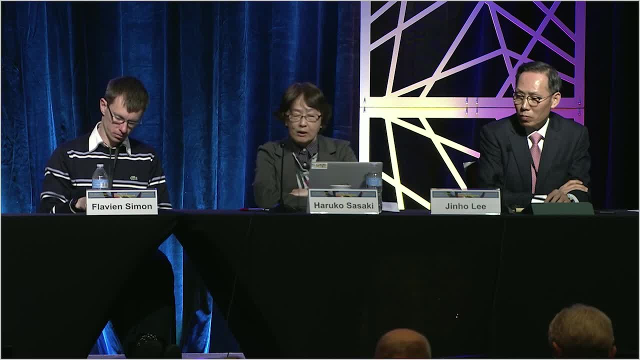 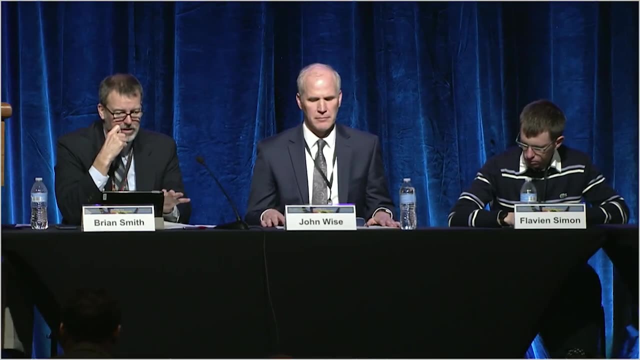 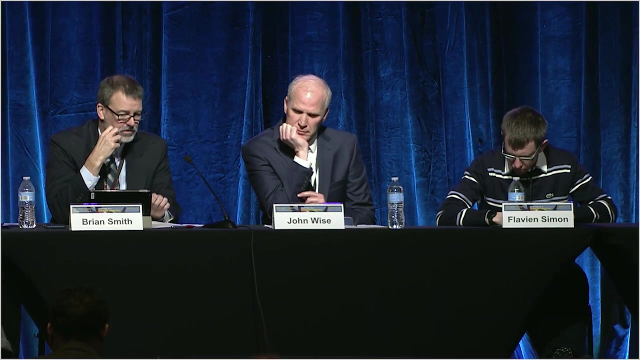 the situation, but it's very difficult to explain about that, Sorry. Okay, All right. We talked about operational experience a good bit up here and the evaluation of that. So, given the worldwide implications of aging management, how do you incorporate international operating experience? 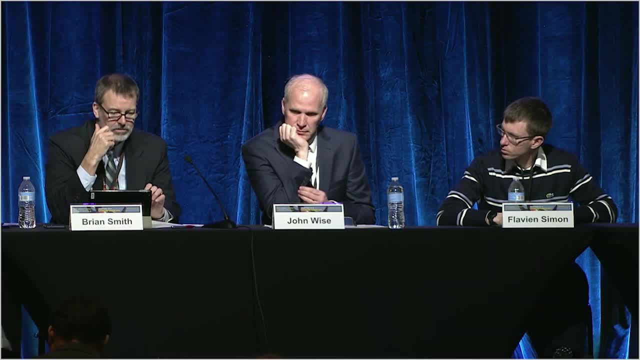 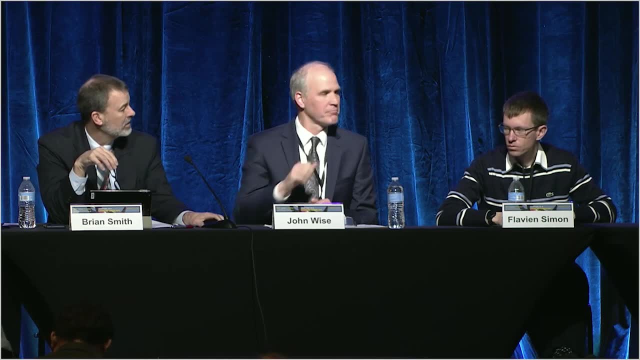 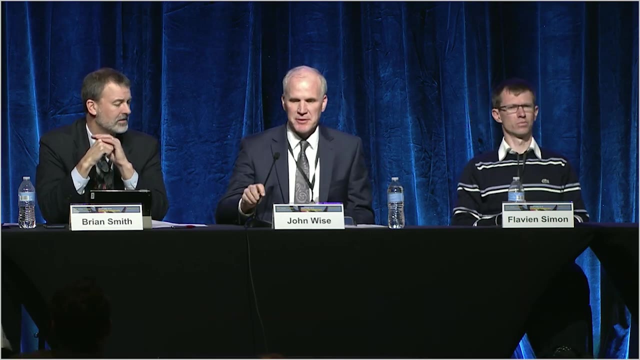 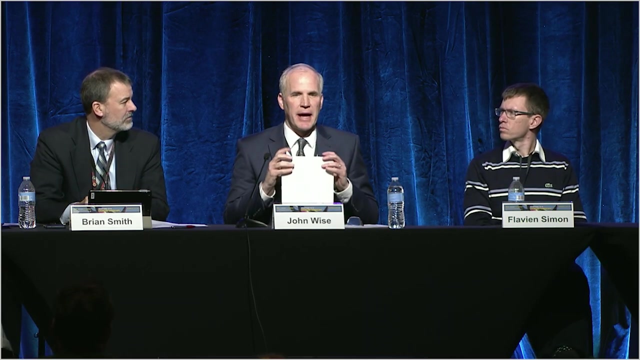 into your guidance, And how do you share operational experience with our international counterparts? John, I'll just kick this off. So a few mechanisms First of all. I know there are international operating experience databases that we certainly can pull from, But I guess I would say is: 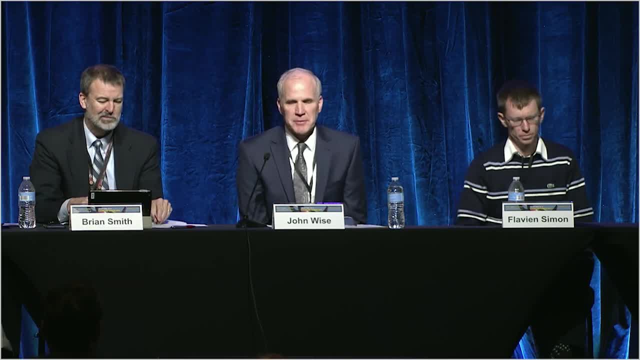 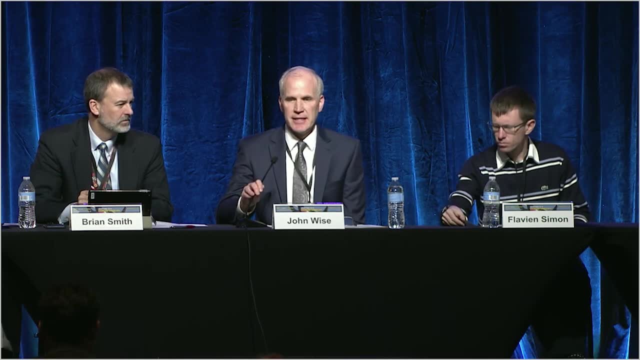 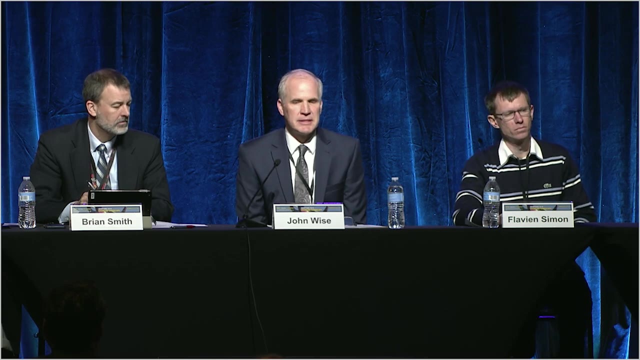 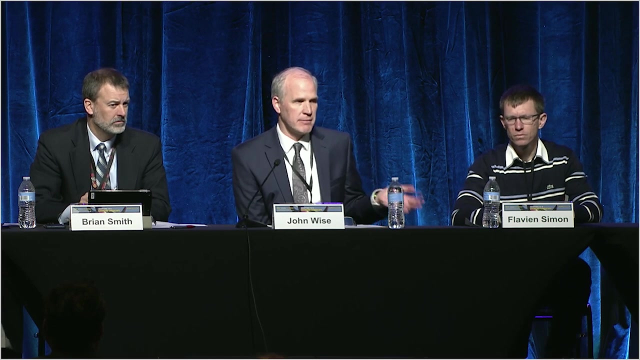 one of our, I think one of the most powerful means of utilizing international operating experience is some of the activities that Brian mentioned at the very beginning the kick off of this session, Which is developing relationships with our fellow regulators and international plants through cooperative, wide cooperative. 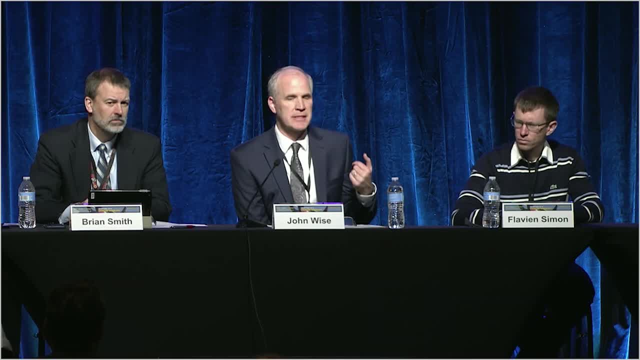 efforts like the IEI-IGAL program, for example, As well as one-on-one. It's very common for us to meet in these large cooperative groups, but we regularly meet with both foreign regulators and foreign plants. It's very frequent to talk about. 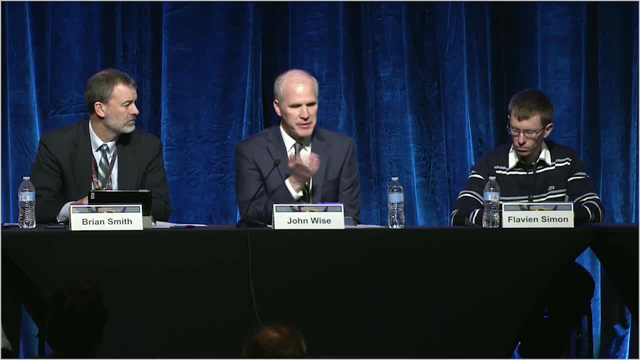 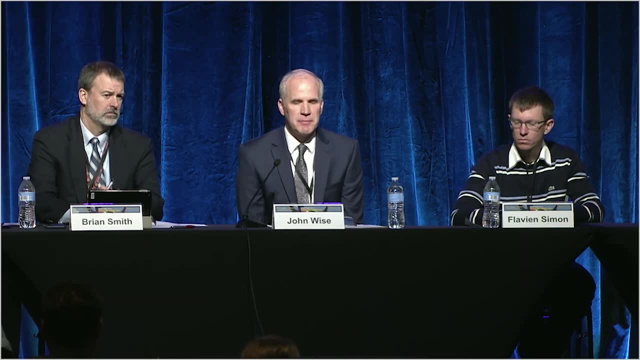 long-term aging issues, And Brian mentioned just a few of the interactions with the countries that are here on the panel, And I think what is most powerful about that is developing the personal relationships, because when something happens- and I'll just use an example of the French- 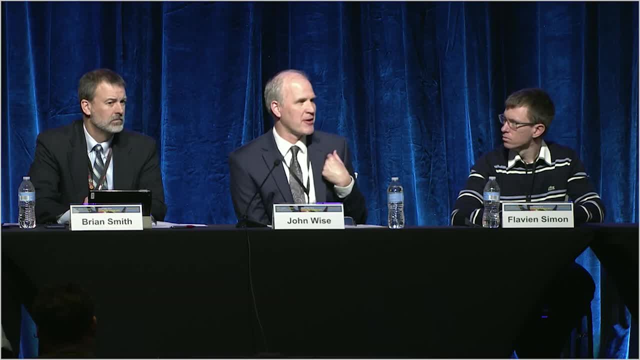 operating experience where they had cracking. You know what was our initial reaction to that? Well, that was to have our senior technical advisor, Dave Rudling, get on the phone and say, Dave, call all your contacts in France and get all the information you can. 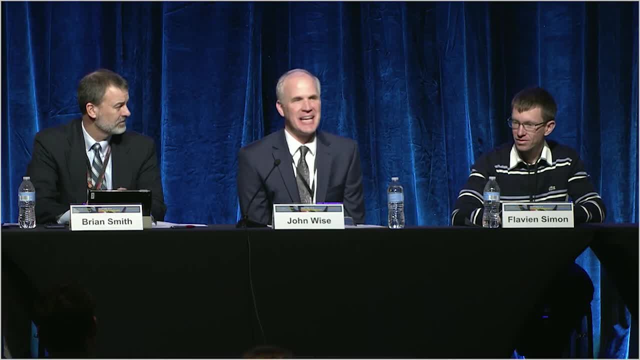 get. And how was Dave able to do that? It was because of all of the relationships that he developed through our interactions, and that's made our participation in all the international groups, whether it's NEA, IEA or others, just really valuable. 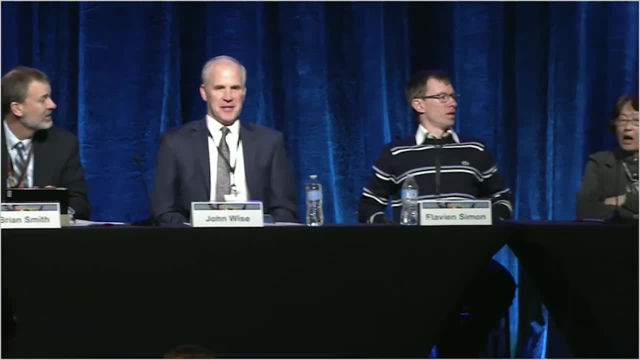 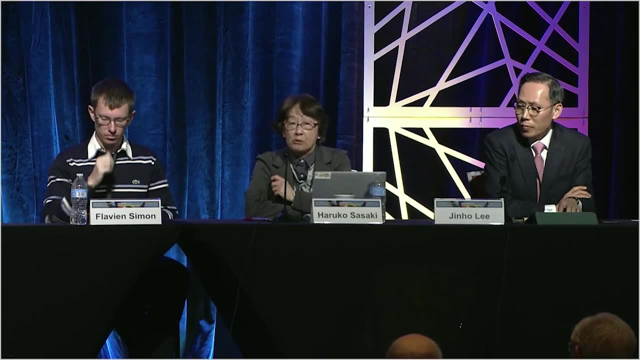 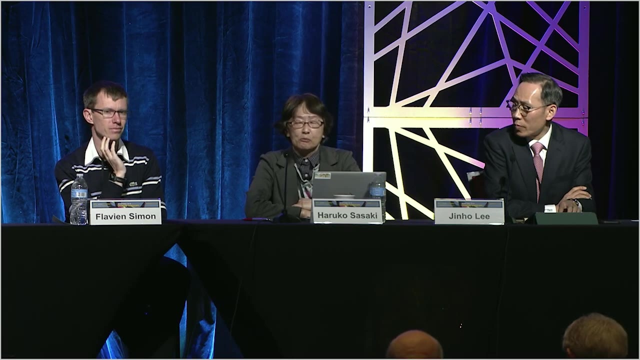 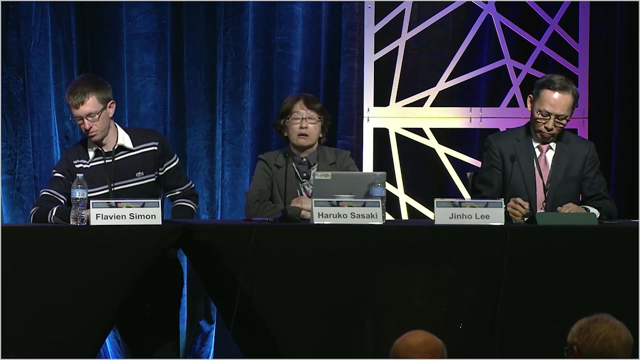 Anybody else want to? Yeah, I agree your opinion. In Japan important operation experience came from the personal connection Mainly, But we collecting the operating experience from all over the world And we make the consideration or resolution of the technical issue. 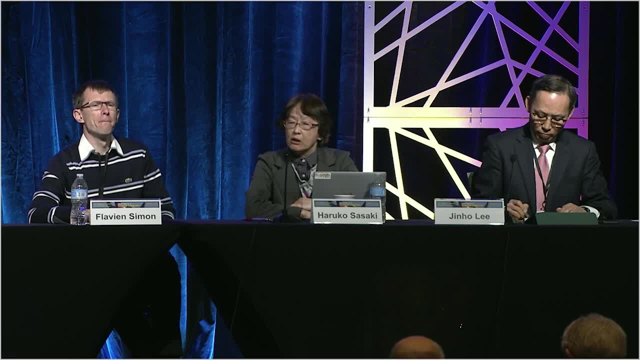 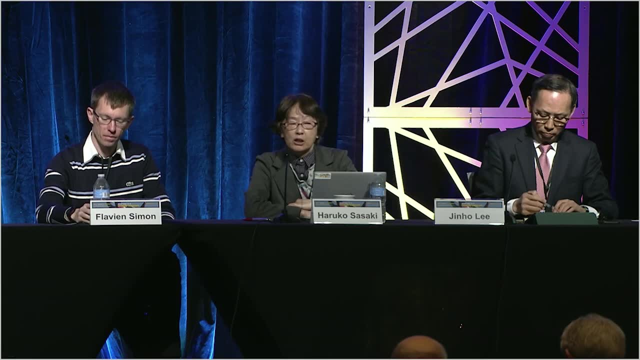 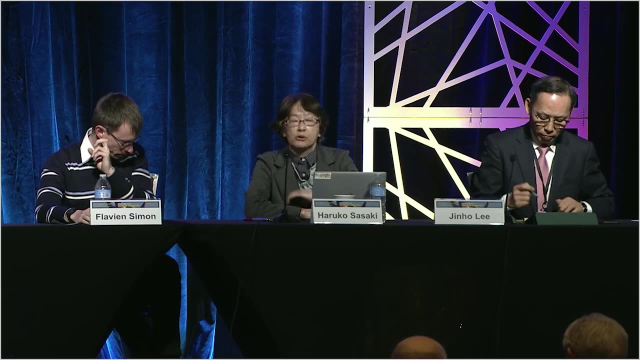 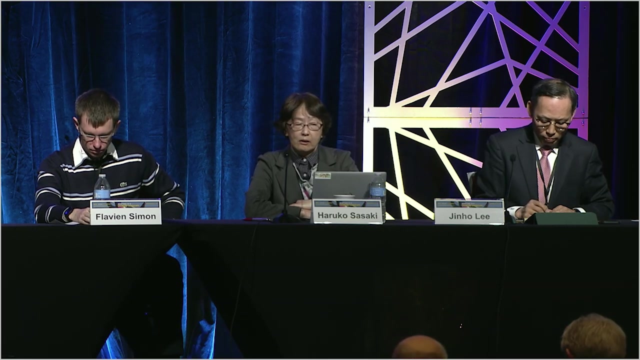 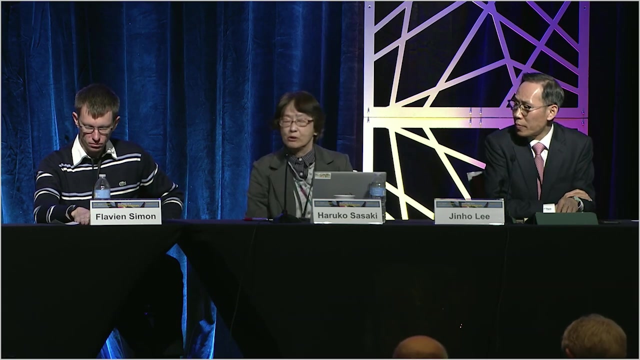 to make meeting material of the technical information review meeting And they provided to the licensee And the licensee showed the meeting material and considered the action and put into the PSR safety review of the licensee. But it's very important to correct method, as mentioned before you. 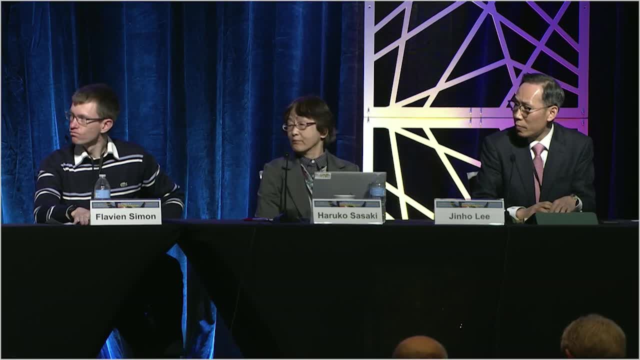 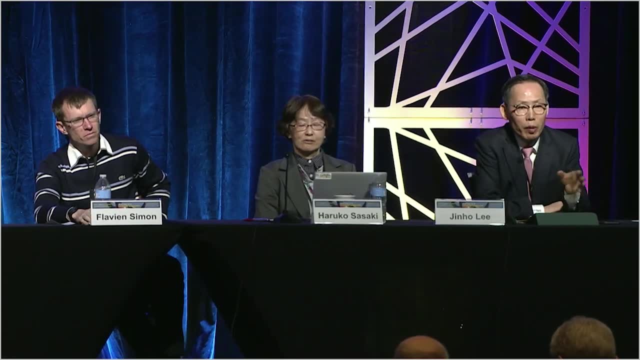 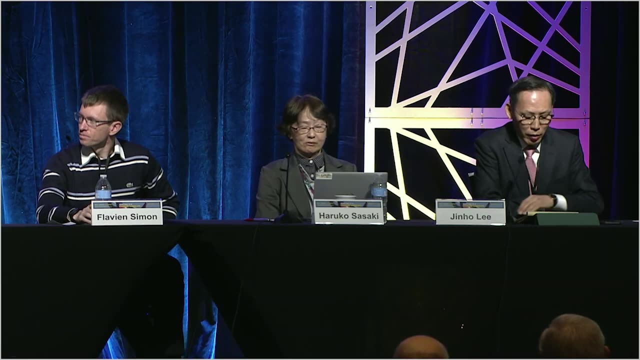 as you? Okay, Jeno, do you want to answer? or In Korea? we are using many different operating channels for the operating experience sharing. One of the approaches to using through the IAIRS systems is a multi-national data sharing and information sharing. 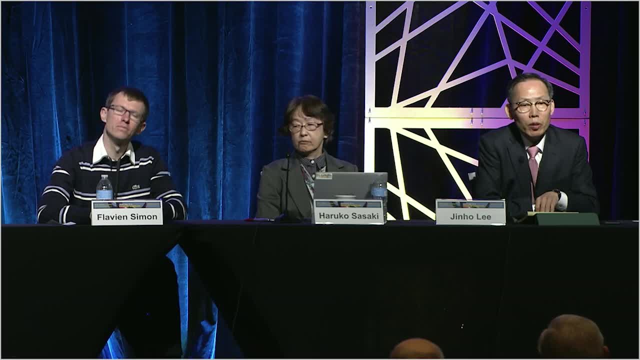 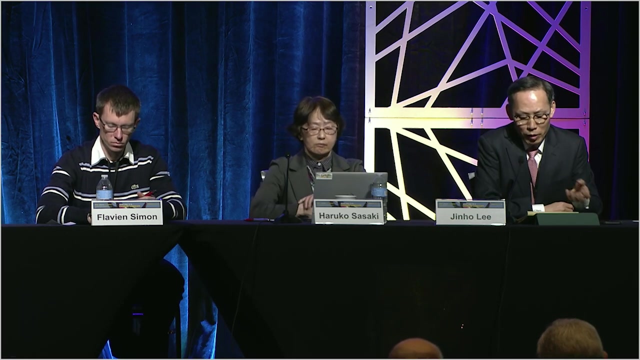 The other one is the TRM Among the three countries in Asia, including China, Japan and Korea. we are holding the TRM meetings every year. One of the important agenda is the operating experience sharing Through the channels we are sharing our information. 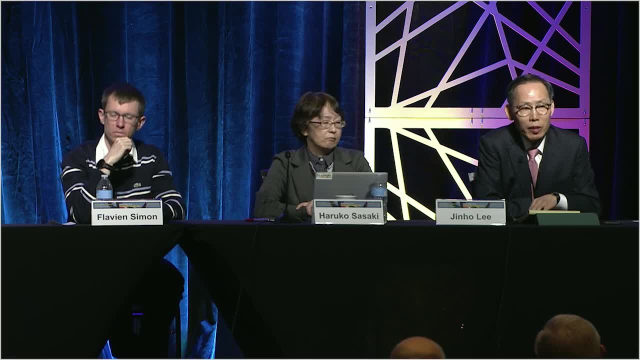 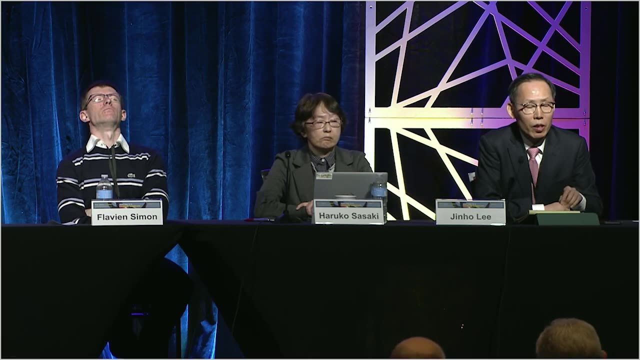 and we are using bilateral meetings. One of the good examples is the cooperation between Korea and the UAE. As you know, Korea exported the nuclear to the UAE. We are periodically sharing information with them And we also use our website. Using our website. 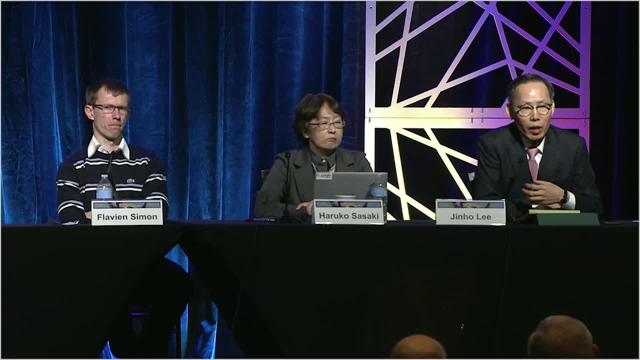 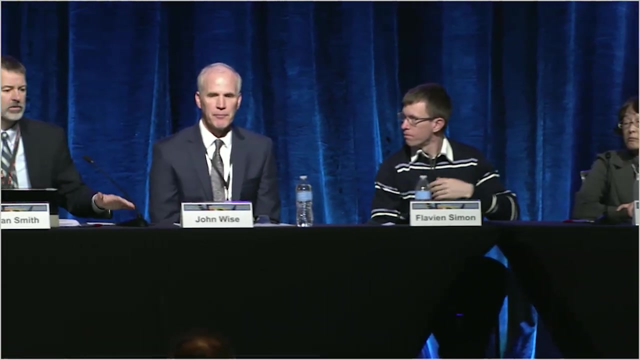 all kinds of information is omitted. If the foreign persons are interested in our information, you can visit our website and can download all useful information. Thank you, Alright. Well, thank you everyone. We are drawing to a close here. I just want to thank my panelists. 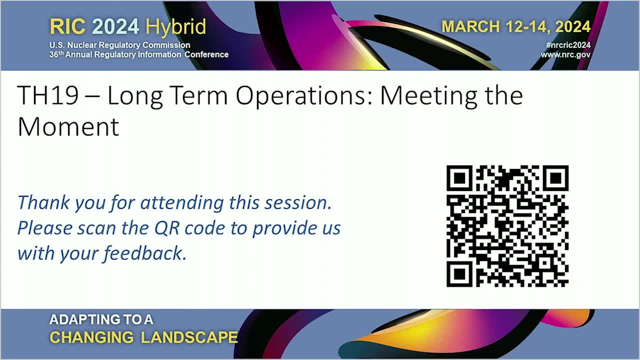